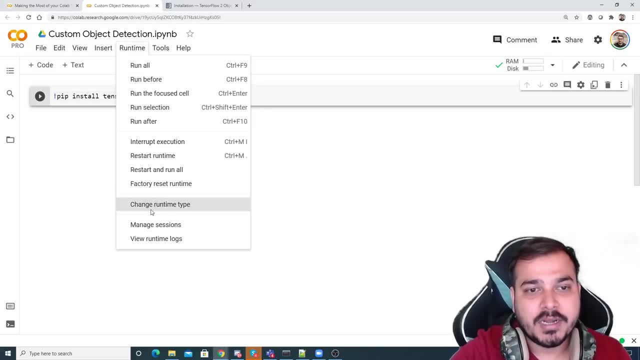 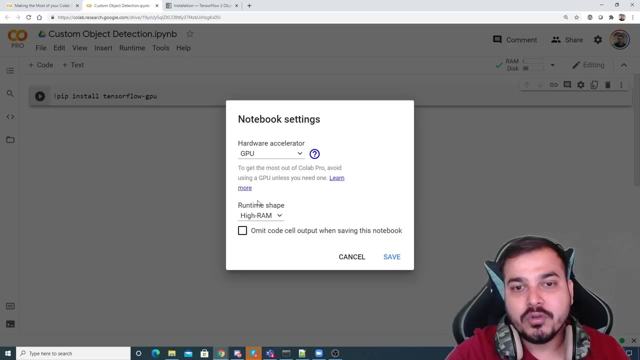 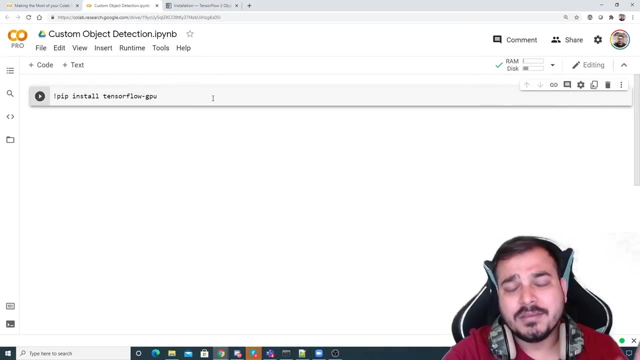 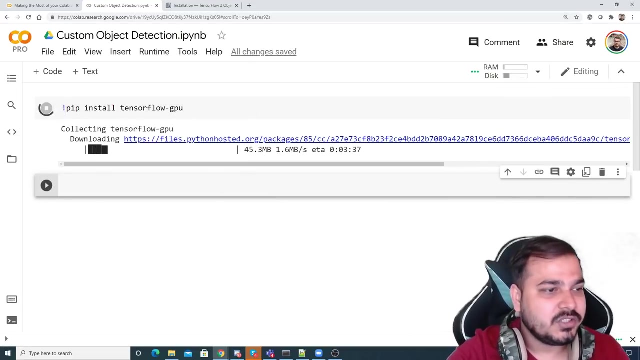 So I'm just going to install this, But before that, make sure that you change the run type- run type to GPU itself. So you just have to make and select GPU. When you're using Google collab pro, you also have this run type shape as high RAM, Okay. but if you're using normal Google, Google collab, I think you can directly do with it Okay. So just select GPU and just start doing. okay. So here I'm just going to install this, So this TensorFlow GPU will get started installing, And then I'm just going to go and see TFOD GitHub, Okay. 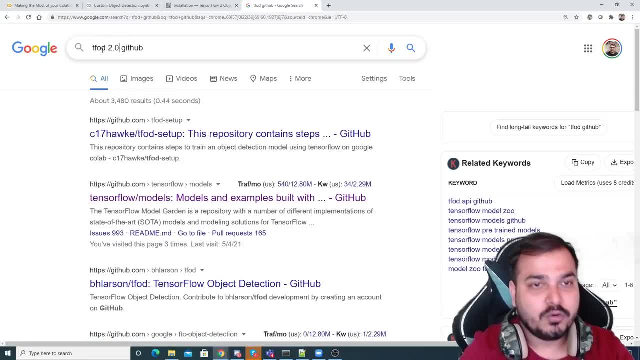 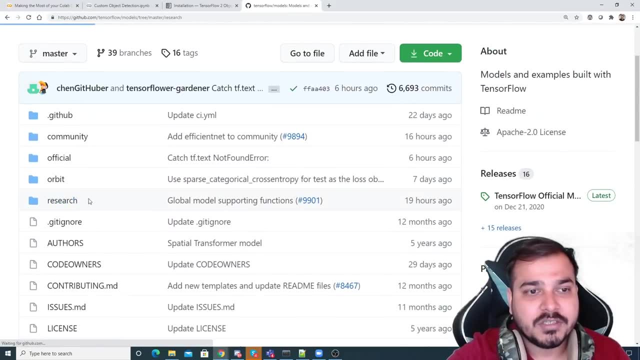 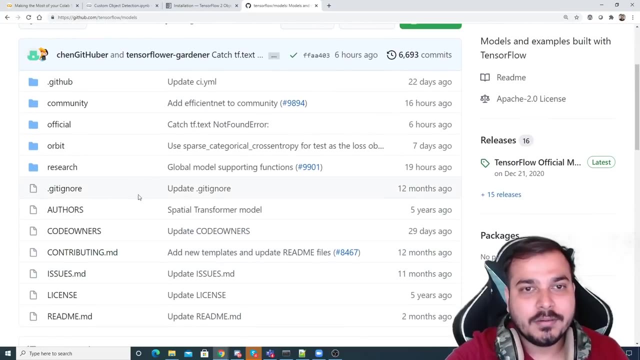 so just go and say search for tfod 2.0, github, and here is basically your example: tensorflow. this is their research folder, is there? yes, i really need to clone this entire repository for my purpose. so, in order to clone it, okay, because i'll be reusing this entire clone. 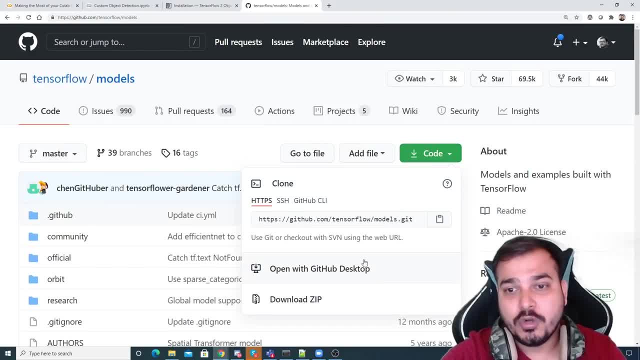 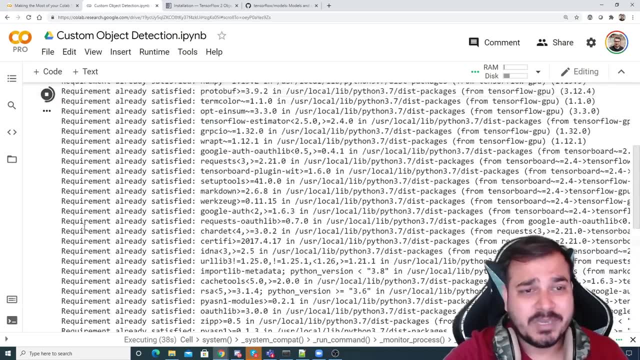 and we'll be making that whole setup itself. so i'm just going to go and copy this githubcom tensorflow models dot get, because this is what we have to clone and you have to follow the same steps. guys, nothing as such. okay, so by default, i think tensorflow gp will be there. i'm just trying. 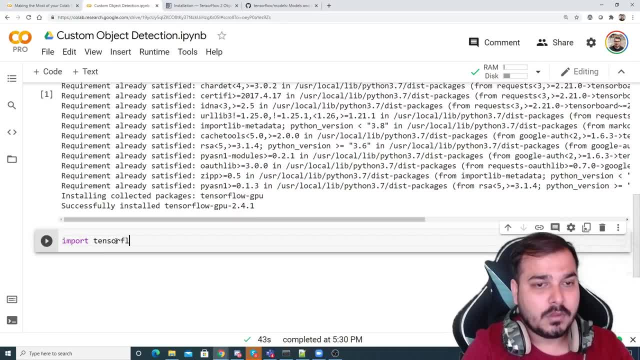 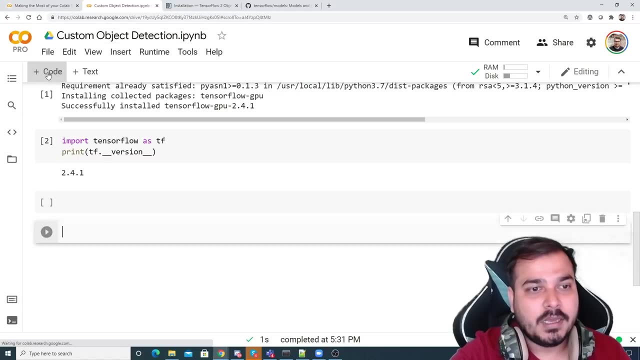 to check it out. so let me import tensorflow as tf and just let me see which is the version that i actually have. okay, so here is my print tfversion that is 2.4.1. okay, now let me just write many number of codes. probably now the next step. i'm just going to git clone. 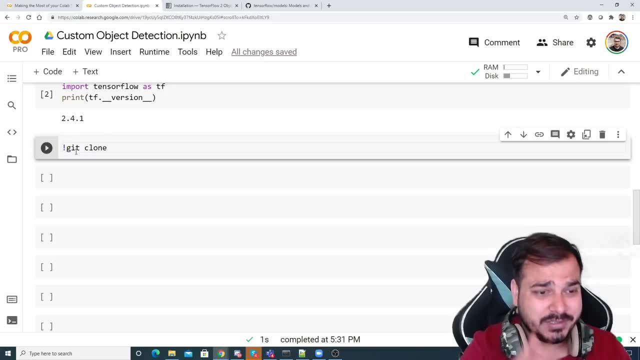 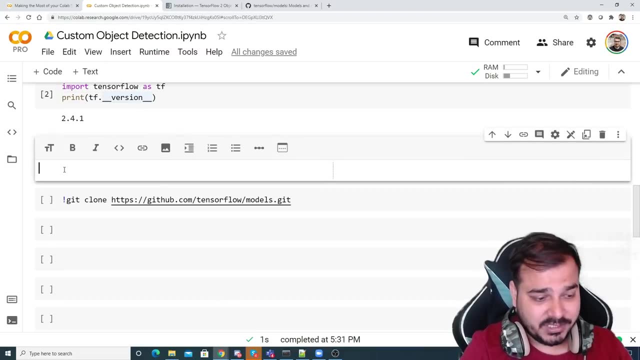 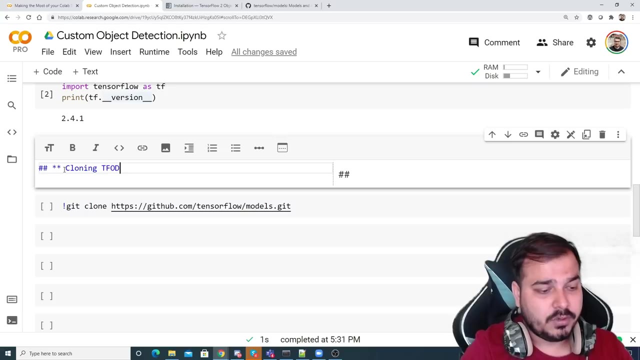 the entire tfod uh github itself, the repository. so i'm just going to paste it. okay, before that, let me just add up a code uh text saying that i can basically write something like this: cloning tfod 2.0- github- right, so that you will also be able to follow. anyhow, i'll be giving you 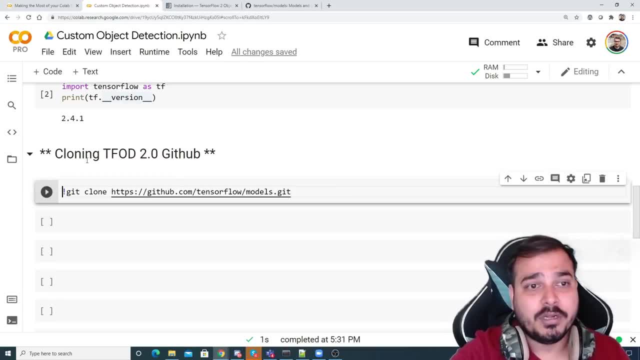 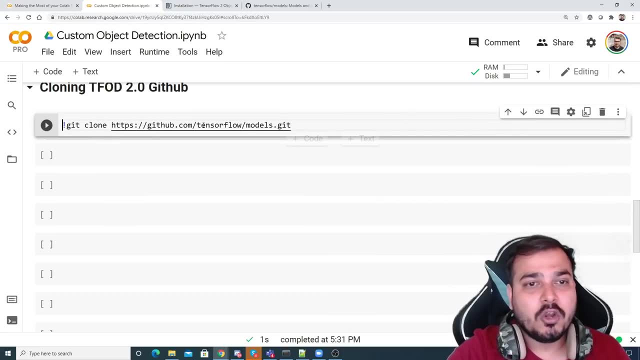 this, uh, so that you can follow it however you want. okay, sorry, this needs to make it as well. i think it should work. yeah, perfect, so let me clone this entire repository for this. i'll just execute it, the cloning will happen, and here you can see it is happening properly. 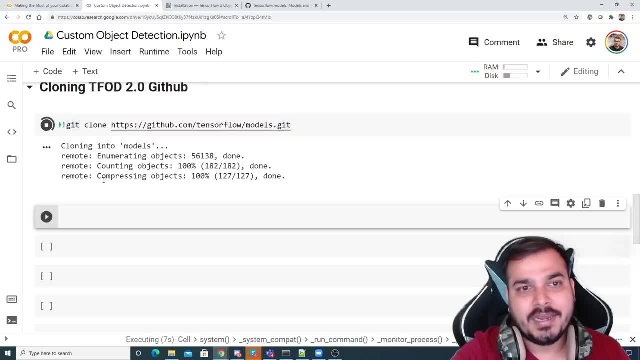 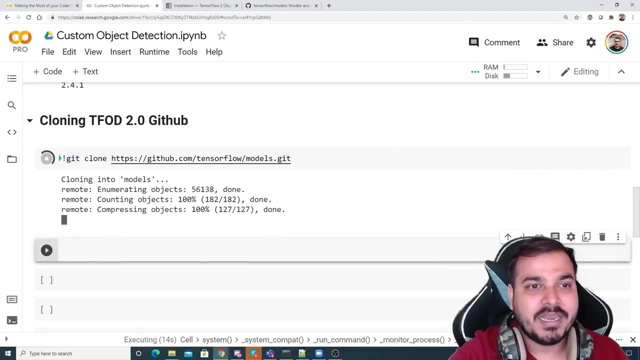 so the cloning, and again we have to wait. it is like nothing will happen very quickly, so we have to wait and for that, for some of the times we will be taking a lot of times and some of the times will not be taking a lot of time, and all right, so it is better that i go slowly. 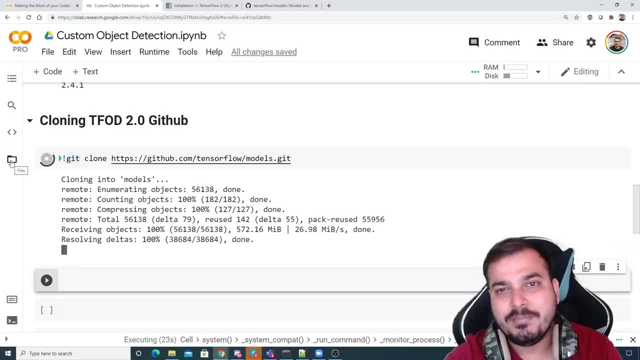 and probably i also divide this particular video into two to three times, and i will be able to do that. so let me just do it, and i will be able to do it in three parts, i guess, and then we'll try to do it, okay, okay, perfect, now if i go and just click in. 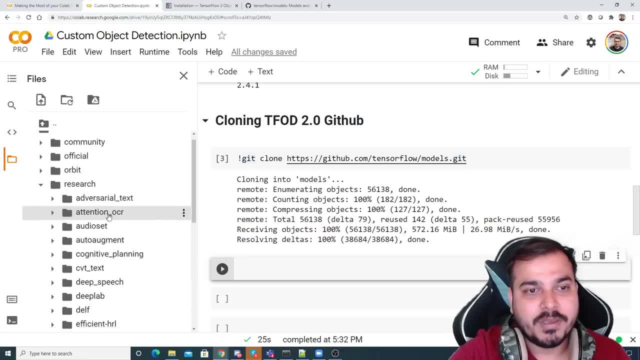 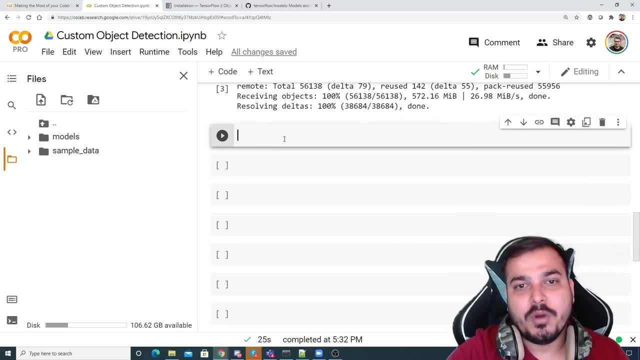 this folder. now this is the entire repository. you can see over here research folder and inside this object detection. all these folders are basically there. perfect, now. i'm in this. now, if i go and write pwd, so it will show me the current directory that is in slash content. now the next thing that 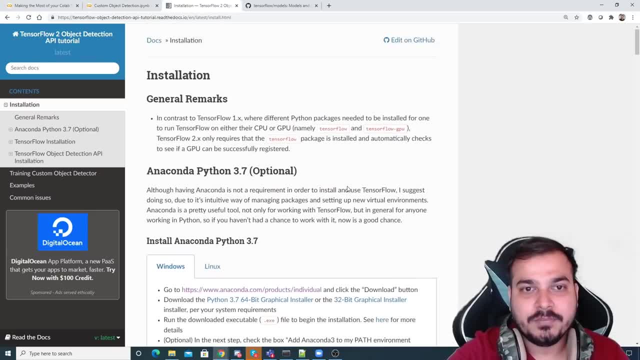 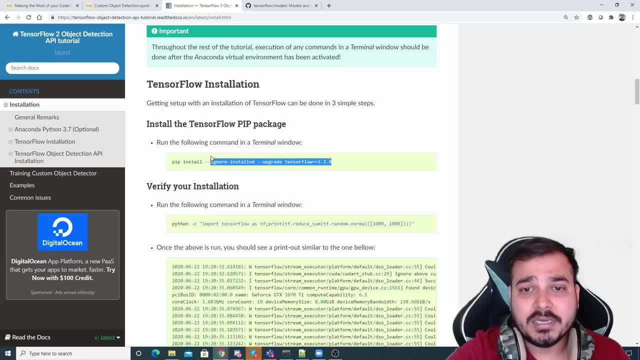 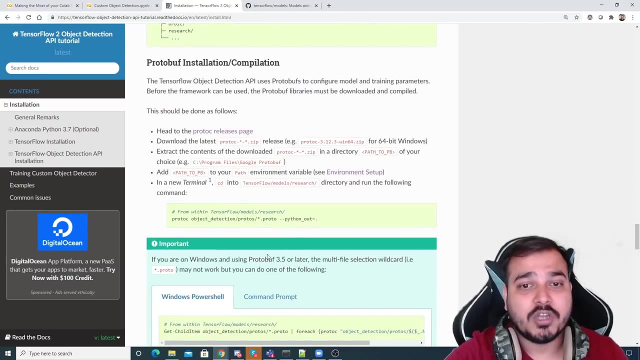 i really want to do is that let's go and follow this documentation now over here, it has told to i'll be having some python environment. it will say, to install the tensorflow gpu, which i have already done. okay, now coming to the next step, uh, what we actually have to do after the installation. 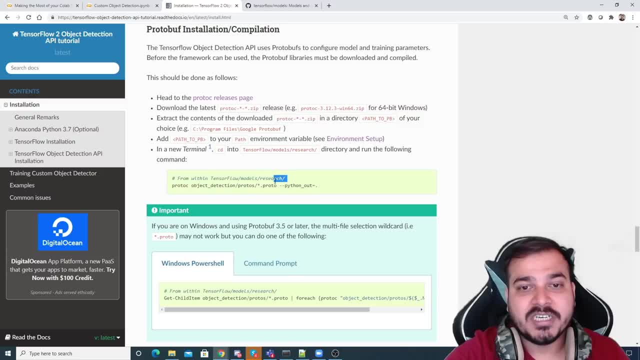 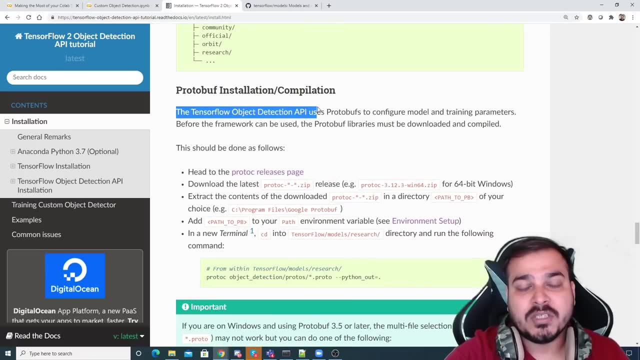 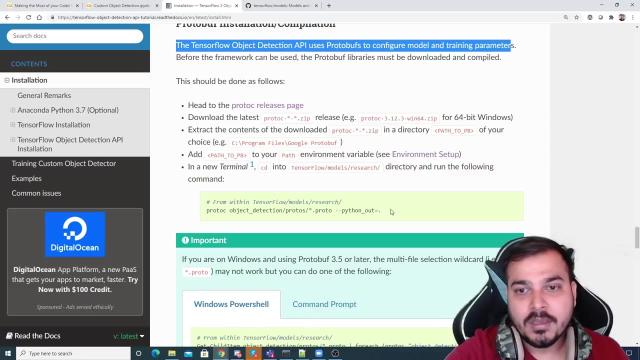 we have to basically execute this proto object detection. uh, python underscore out is equal to dot. okay, why this is done? because the tensorflow object detection api uses protobuf configure to configure model and training parameters. so that is the reason why i'm actually using this. okay, so i'm just going to copy this. but before copying this, i'm going to copy this and i'm going to copy. 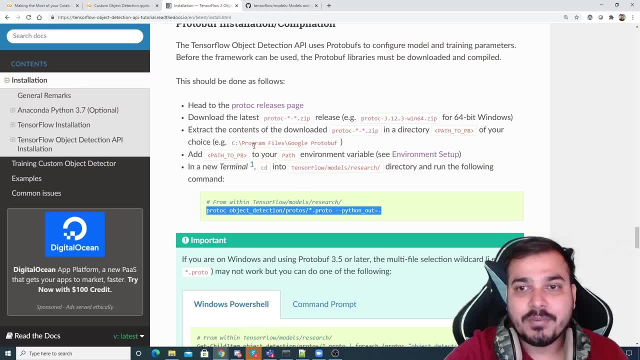 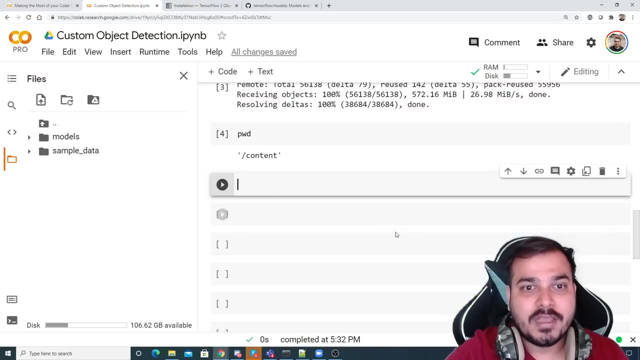 it what we have to do. we have to move into which directory probably? so this, uh, i have to go inside my tensorflow models, slash research. so if i go over here, guys, right now, i'm inside content, so i'll go inside models and then i'll go inside research now in order to go it what i'll write. 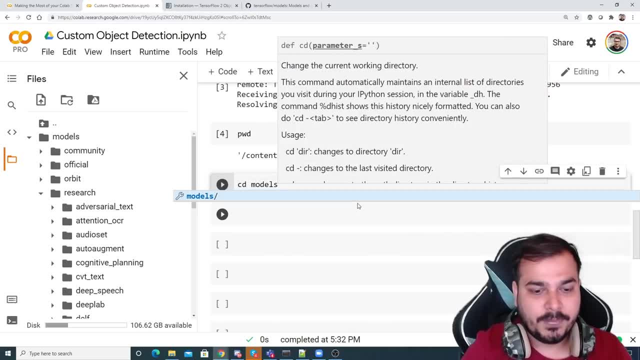 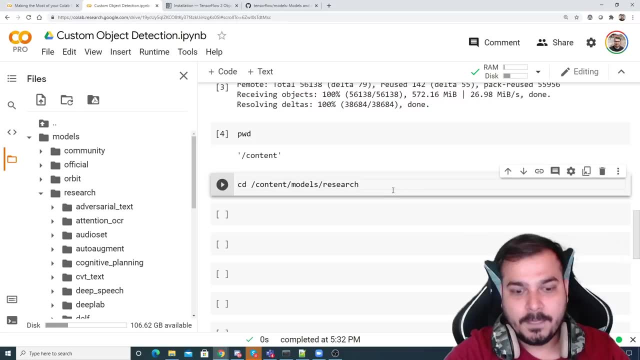 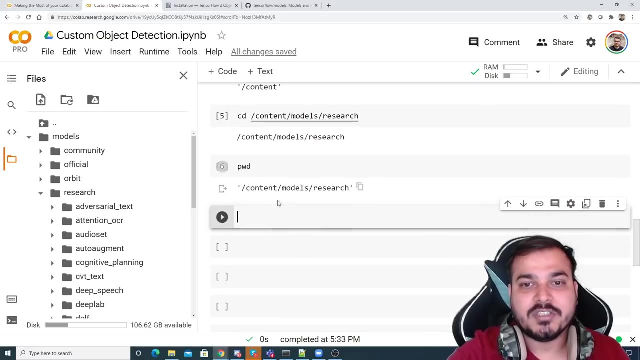 i'll write cd. change the directory to models- probably, okay. i'll just copy this entire path. okay, and i'll paste it. okay, so just execute it. cd this now. if i go and write pwd, i'll be inside this particular directory which is called as research. now, after going into this, i just have to copy this entire protobuf command. so i'm just going to paste. 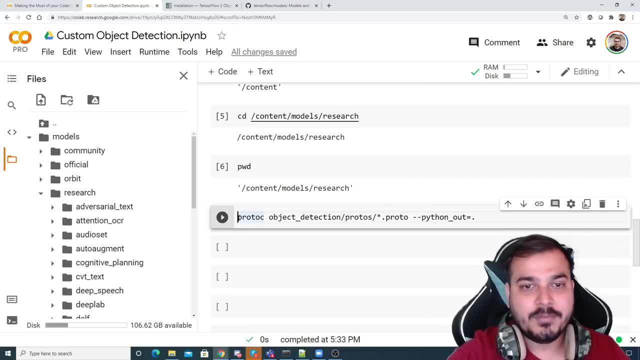 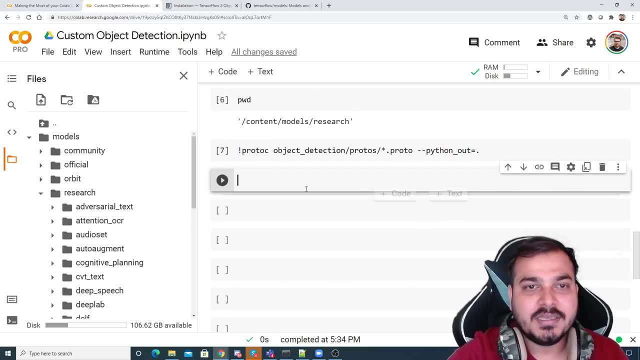 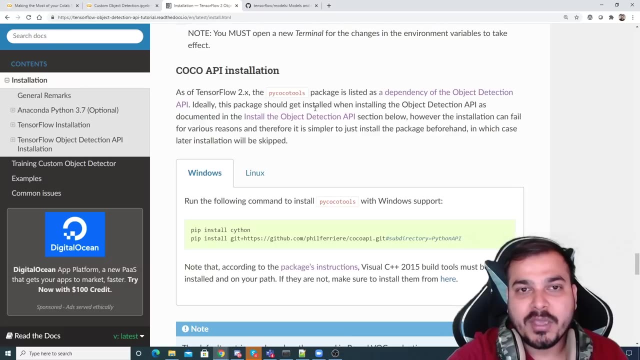 it and just use an exclamation mark, because this becomes a bash command altogether. now this has got successfully executed. perfect till here. it's amazing. everything is going perfectly fine, and let's go to the next step. after this, we have to do the coco api installation. in doing the coco, 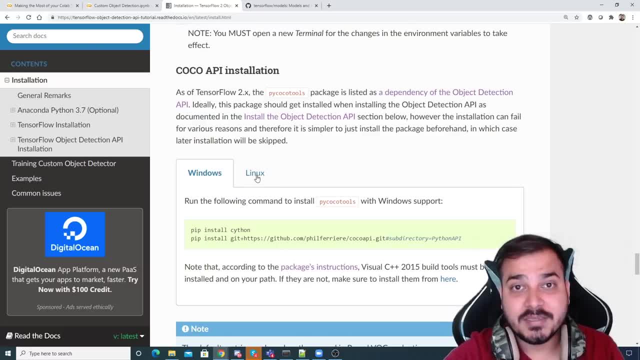 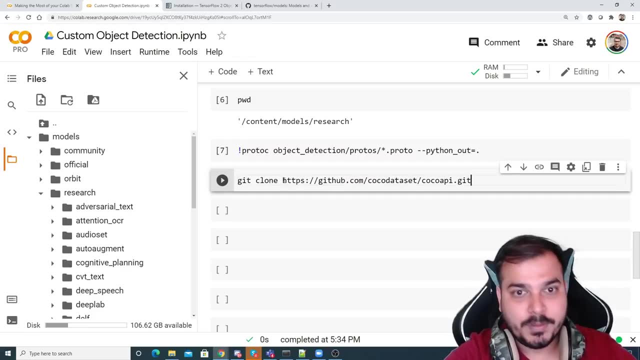 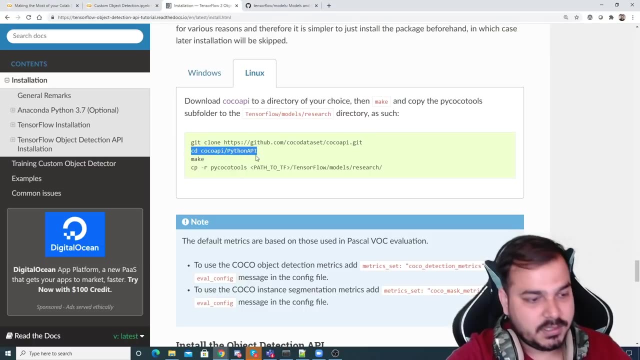 api installation and google collab. if i'm using it will basically be a linux machine, so i'm just going to execute this. git clone. okay, git clone, and here i'm just going to paste it. okay, i'll write like this: then let's paste it one by one: cd. this fine, this will be a bash command again. 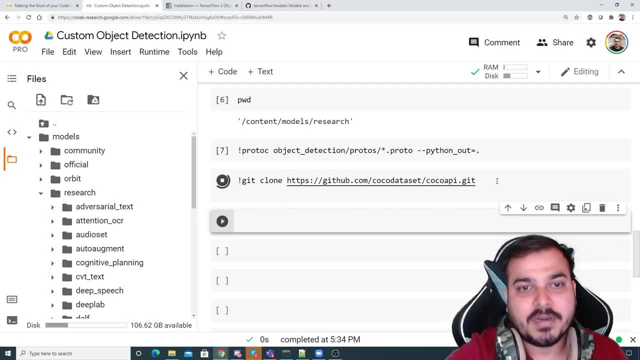 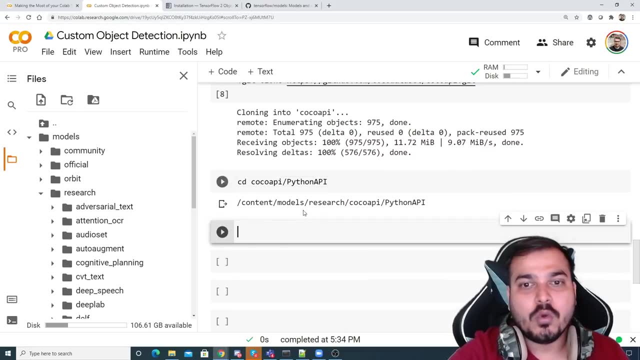 let me just do it line by line, so that it will work perfectly fine. okay, so api is getting cloned. then let me paste cd, coco api, python, api. so i'm inside this particular folder now and i will just be executing this make. make command is basically for the compilation purpose. 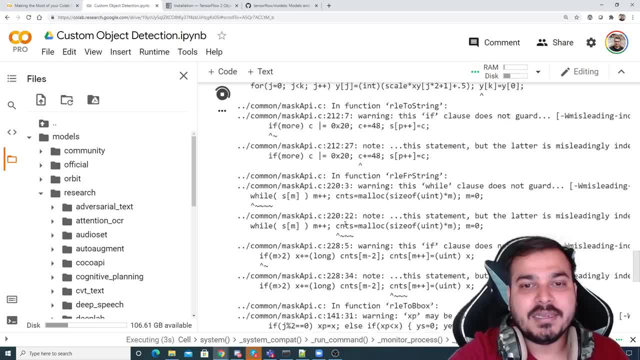 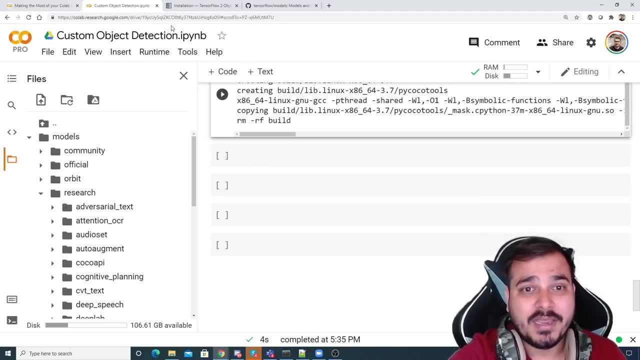 okay, so now the setuppy file. it will get executed. perfect, that has got builded. now, by using this main, i hope everything is working fine. i will come to know just by seeing it. then what i'm going to do is i'm going to copy this entire command again, paste it over here, and this is nothing but this. 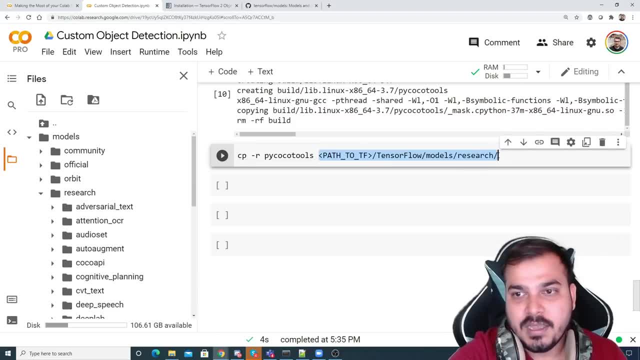 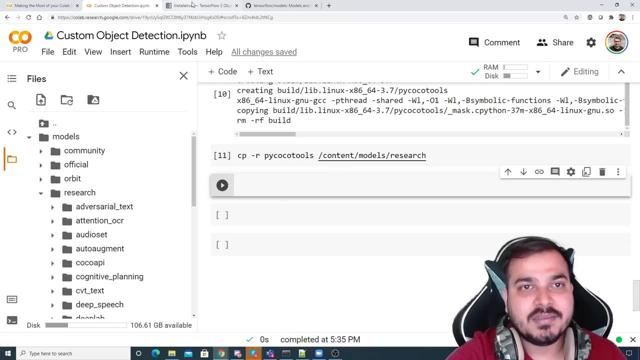 is the path of my research folder that i have to give, so i'm just going to copy this path and put it over here. right so done. let me execute it so perfectly. it works fine. everything is perfect till this particular step. okay, these are the basic installation. now in the second type, we 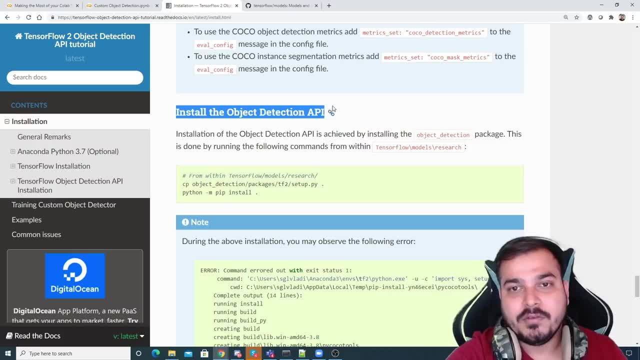 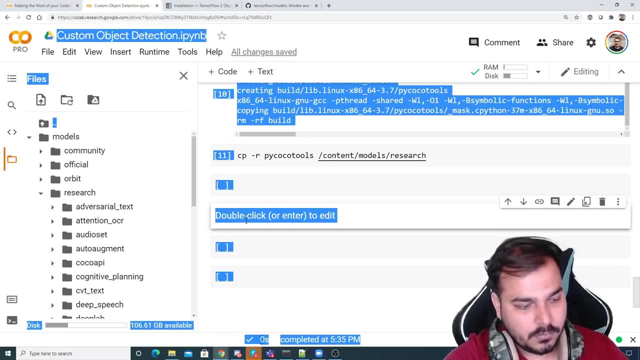 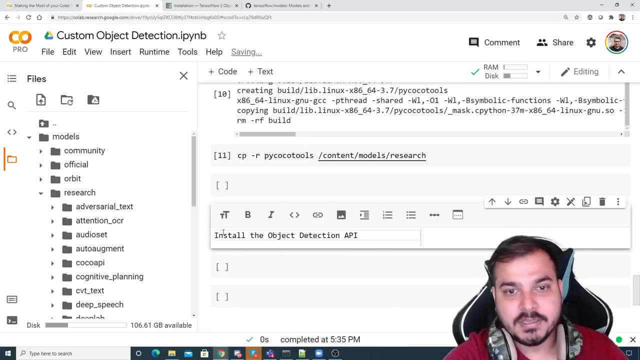 have to- uh, i mean, after that we have to install the object detection api. so i'm just going to copy this entire thing. i'll make this as bold. oops, i'll make this as text and make it as bold. right, i can make entire thing as bold. 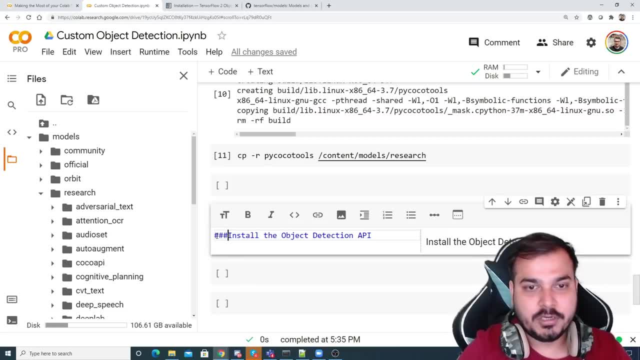 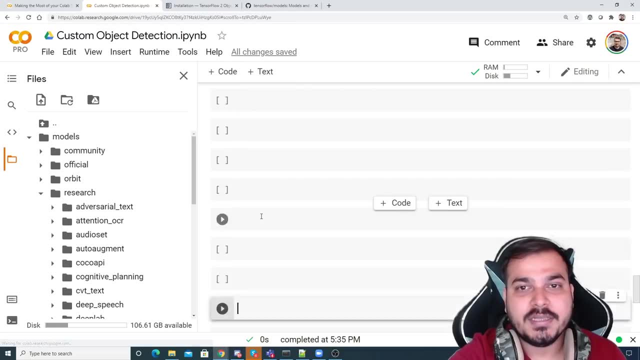 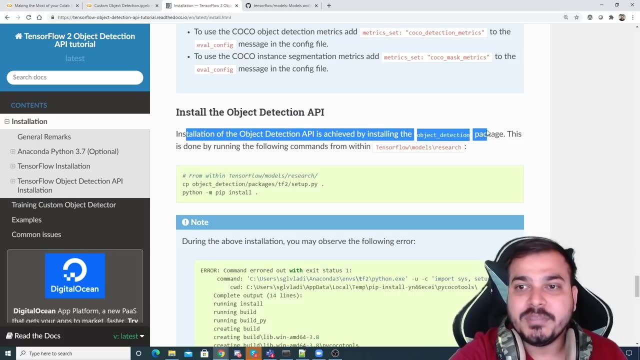 just to, i'll use triple dots and use this, and then it will execute: installing the object detection api. let me create more code cells now in order to do this again. this is also a dependent c. you can see installation of object detection api. achieved by installing the object detection. 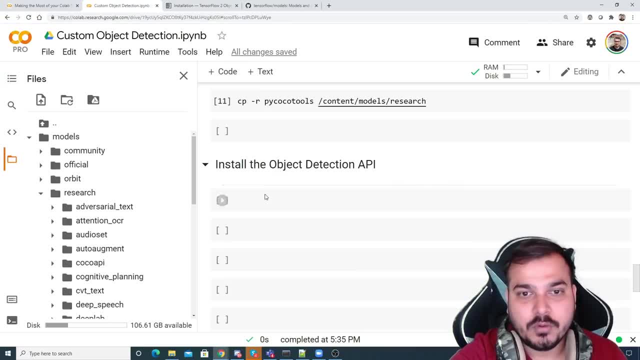 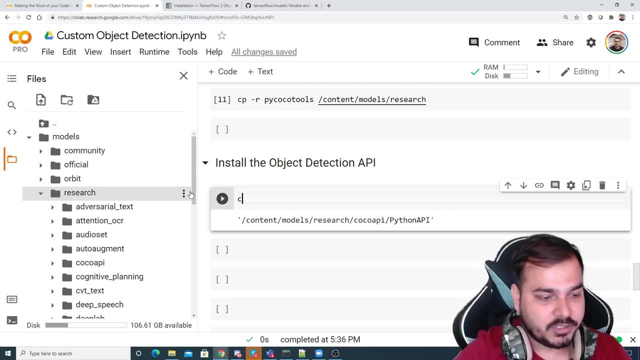 package right now. again, i have to go inside this research folder. so if i go and see what is my pwd, it will be this one. so what i'll do in order to come to the research folder, i'll just write cd dot dot two times. i'll try to execute. then again i'll try to execute one more time: cd dot dot. 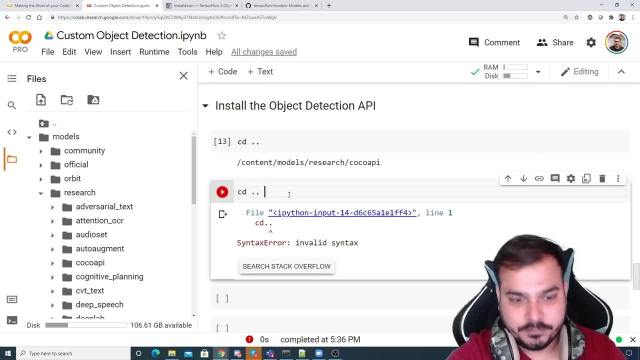 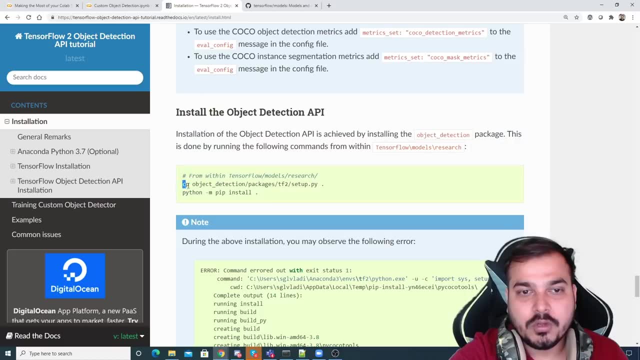 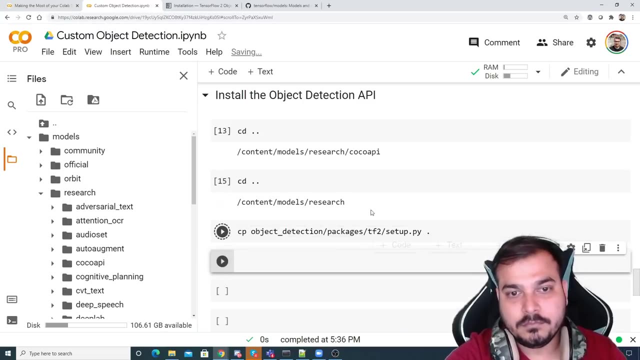 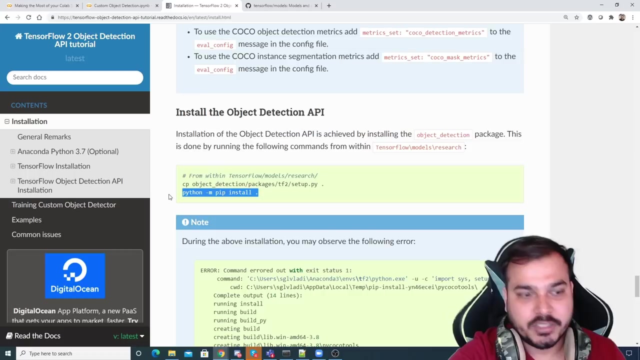 okay, sorry, cd dot dot with a space. okay, now i'm inside my research folder. perfect, i'm inside my research folder. now i'm just going to copy this entire command, okay. okay, because we are actually copying this setup dot py in the main folder itself, and then i will just execute this: python m install. okay, all the steps you just have. 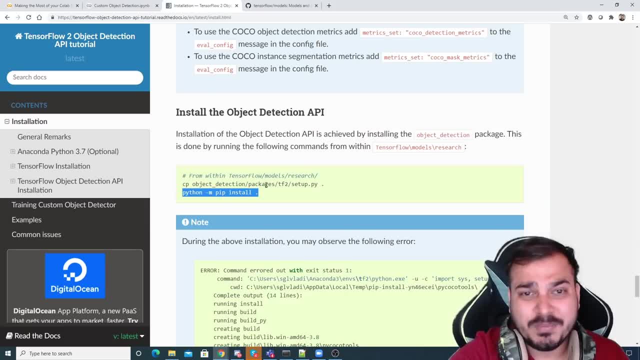 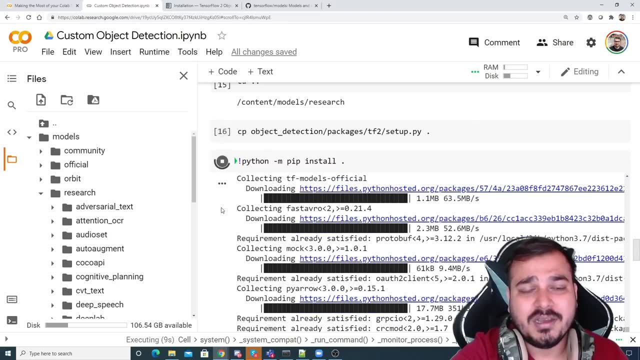 to follow. what is the steps written in the blocks? here now again, i have explained this already in the everything right in the setup part. only i have explained everything, and everybody was requesting: krish, please make this particular video in this google collab itself, right? so i'm actually doing. 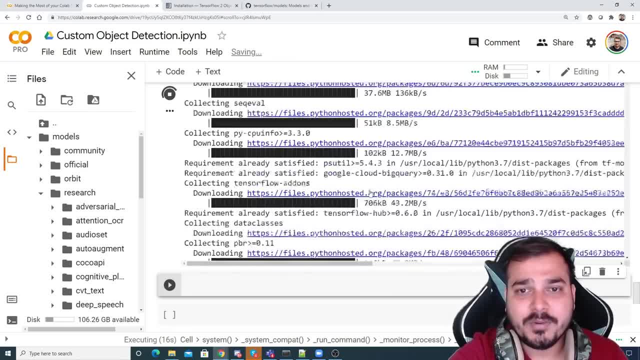 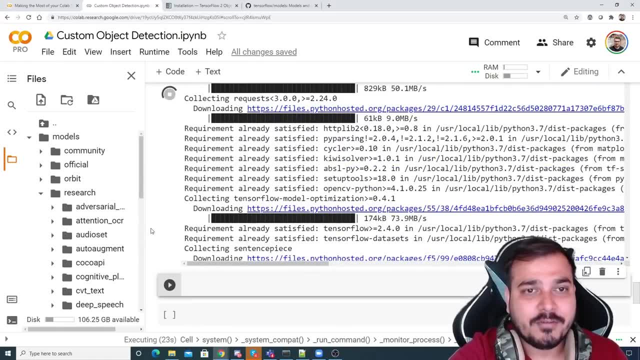 it for you. okay, so you can see over here, everything is going perfectly fine. it will take some amount of time, but, yes, it is good to wake and this is just one time task, guys. so we have to do this kind of setup and automatically, at the end of the day, we will be converting everything into model. 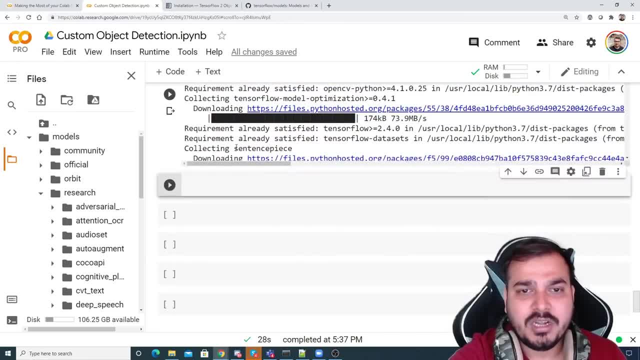 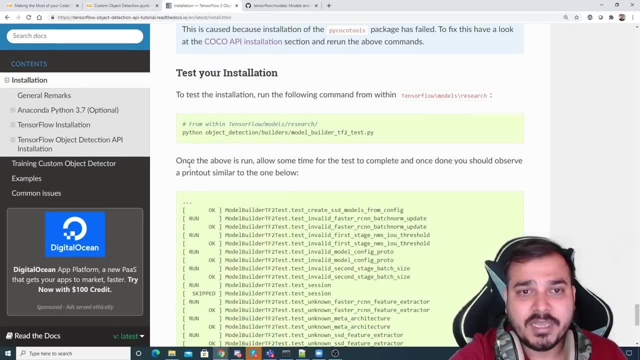 and anyhow, i'll be giving this so it has got successfully installed. uh, so here you can see: requirement already satisfied. perfect, we are in the right steps that we are going. now coming to the next step: test your installation. you want to test your installation? just go and copy this: 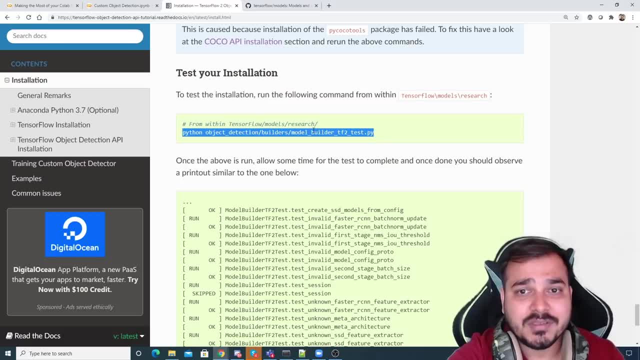 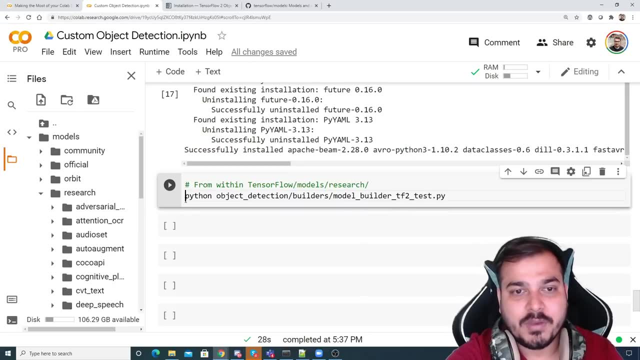 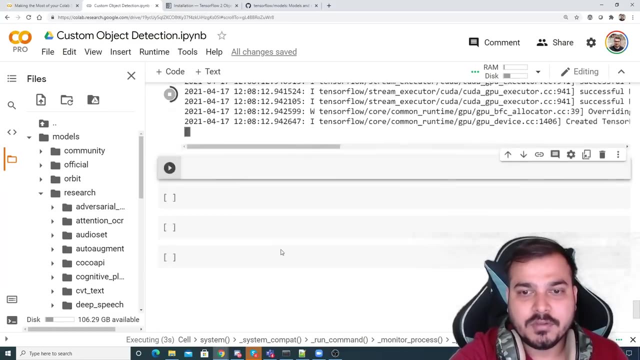 particular command and, again, everything should be happening inside your research folder. okay, from your research folder. that is the most important thing. so here i'm just going to paste it and just try to execute this one. okay, so here you is, successfully done. so this will also work successfully and probably it will show 21 tests. 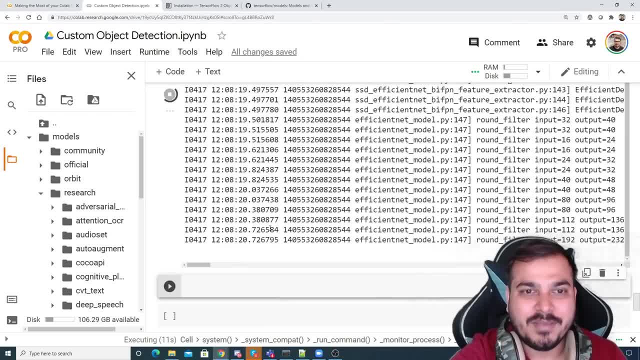 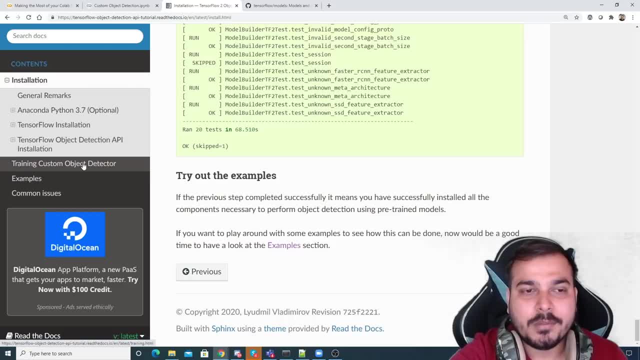 in successfully done so many tests in so many number of times and everything then after that. we can start our examples now in order to do the 10 custom object detector. now we will be going to the next step. i just clicked on the training custom object detector. now we need to prepare. 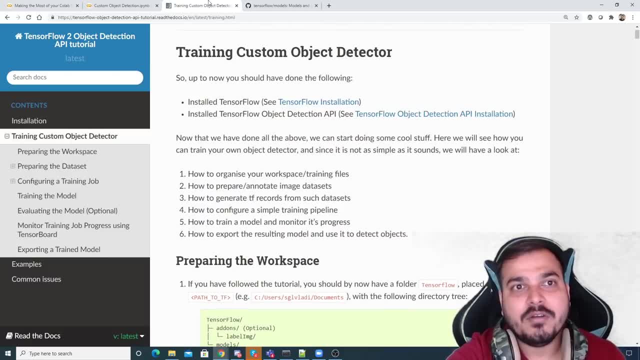 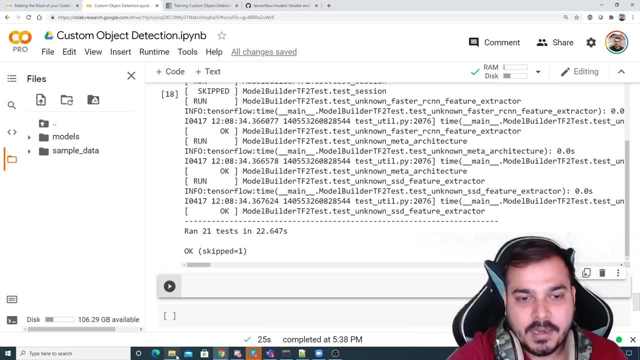 the images now. in order to prepare the images, first of all, we will try to define a folder structure. now here you can see that it has ran successfully. now this is my entire thing, guys, models, and this is there. now i have created a folder structure for you. this: 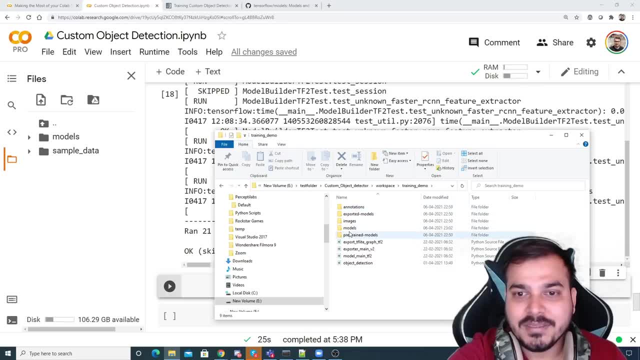 workspace training demo folder. inside this i will be having this folder structure like annotation, exported models, images, models, pre-trained models, and all what we'll do is that we'll also try to make a folder over here. so i'll just create a new folder and just follow this specific pattern. okay. 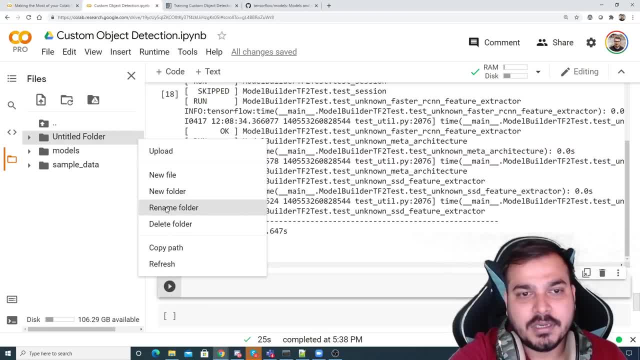 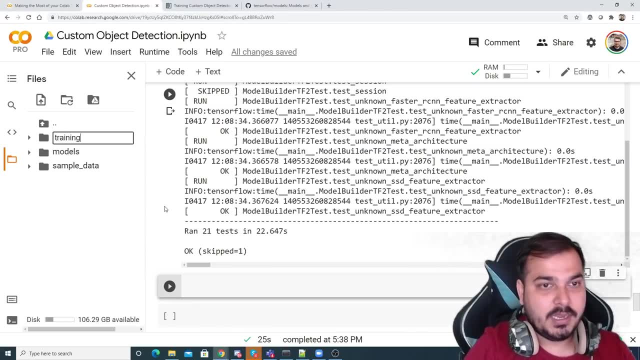 so first of all i'll say, okay, make it as rename the folder. i'm just going to rename it to training underscore demo, okay. so i'll say training underscore demo. now, why i'm making this particular folder structure? because it will be whatever custom thing that you really want to do we will be doing inside this particular. 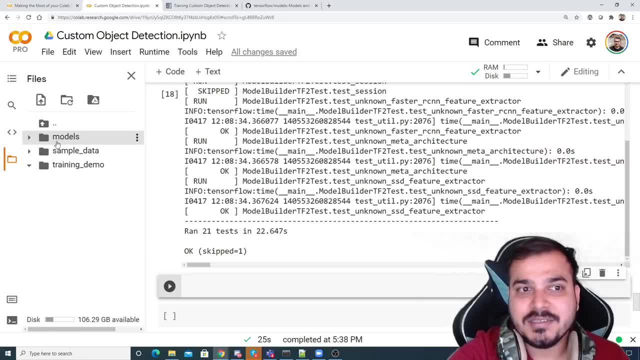 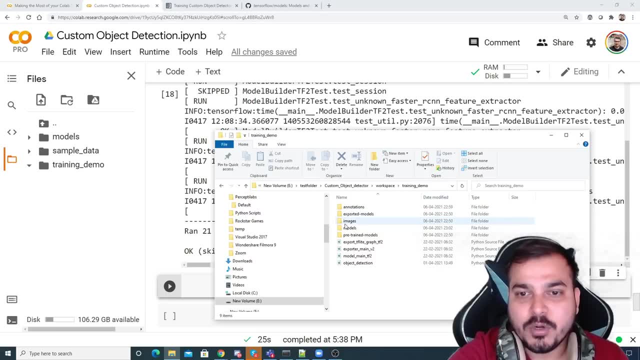 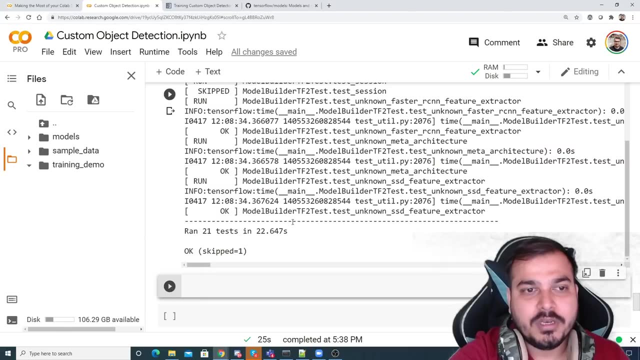 folder and whatever things we require from this model folder inside this research. we will be using it from here. now this training folder is done, then you have these all names like annotations. you have this exported models, images and everything. so let's make this five folders quickly. okay, so um new folder. so 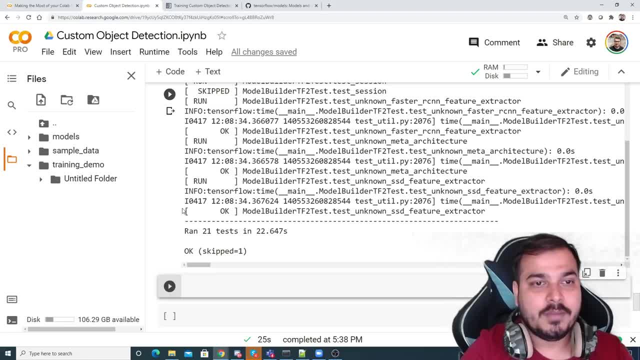 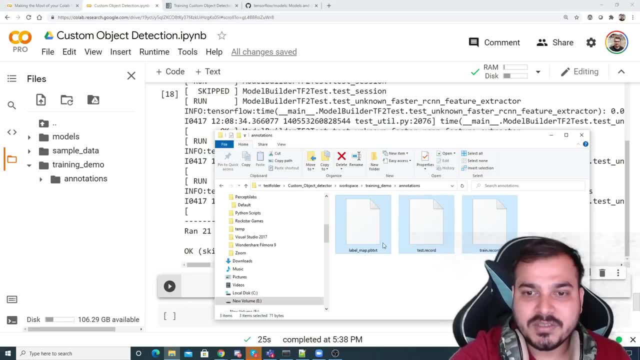 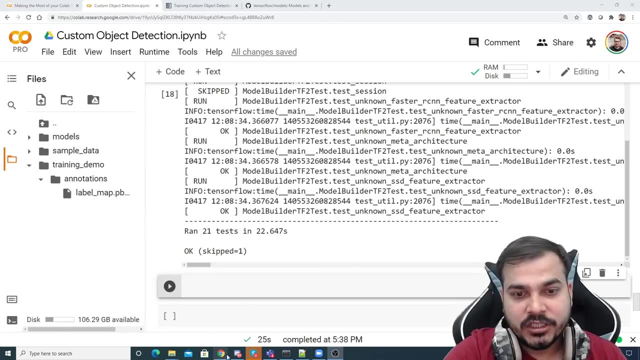 i'm just going to write annotations, okay, so this is my first folder. inside the annotations you'll be able to see this three files. okay, how to create these three files, i'll just show it, but let me just upload it over here inside this annotation. so, guys, uh, this annotation folders, uh, i'm just going to. 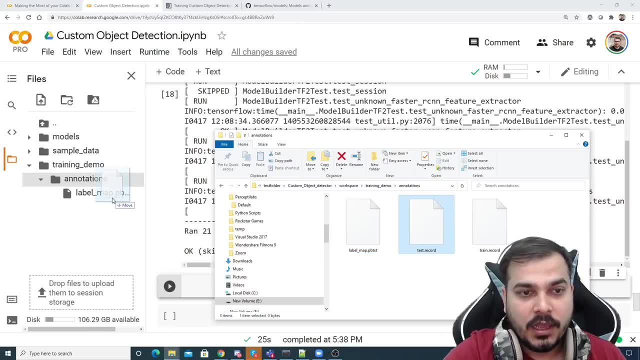 put all these particular files, that is, tf dot record and test dot record, uh, so that you know- i'll talk about this tf dot record, why it is used and all but uh, just just understand the test dot and train dot record. i'll just try to put it. 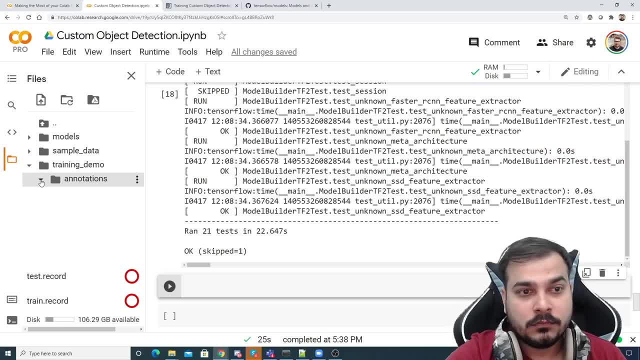 till then, let's make the other folders also. so other folders after that annotation is exported models. so i'm just going to create new folder and i'll say exported underscore models. this will basically be having my final model, once it is trained. okay, just follow this particular folder. 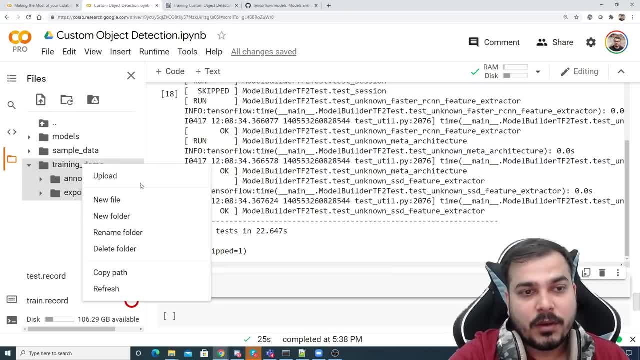 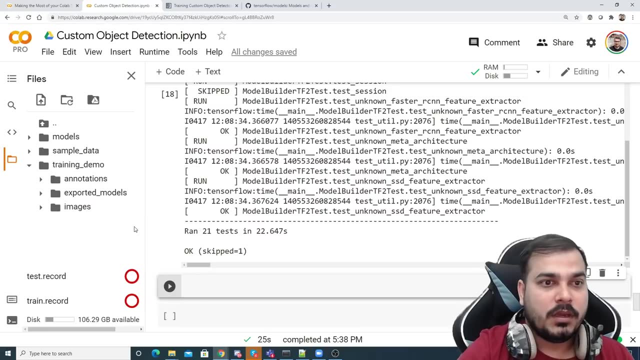 structure, this entire folder structure i'll be providing you. then i will probably make a new folder called as images. okay, so here it is. i'm just going to make this particular folder as images and then i have models. okay, and in the blog also it is mentioned that probably it is better that. 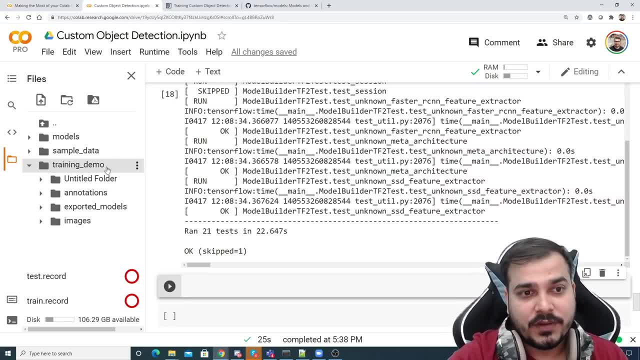 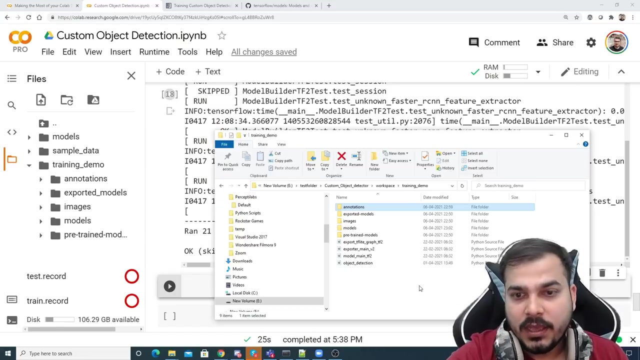 we create this so that it will be, we will be able to understand. so so, finally, we create models also, and then i have something called as pre-trained models. so i have pre-trained models. i think it is pre-trained, pre-trained models, right, so done. pre-trained models is there already. and then coming to the 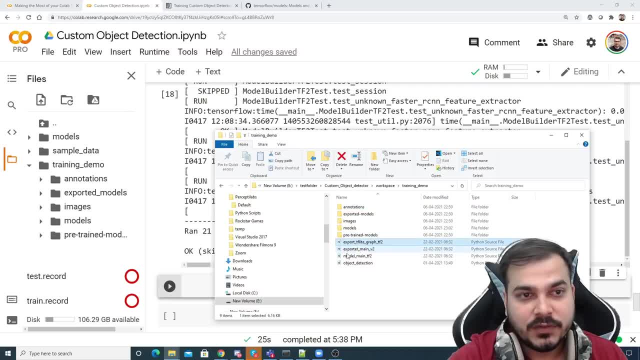 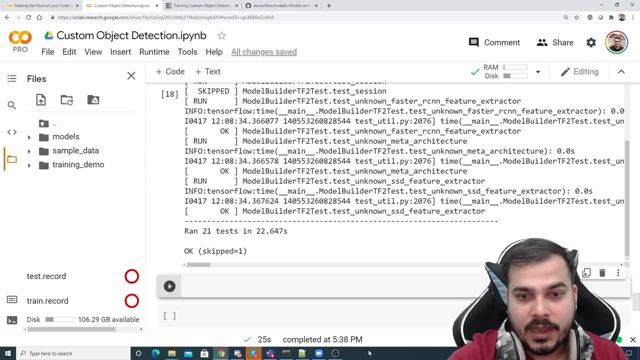 next. next one is the pre-trained one, and there is a PuTTY show also up so that you can get easily. forget about it by onakte. and if you are not having any trouble getting up to 10 million, ver 막 bach tele ho pr id, whatever. uh, this is it. it's just a basic tool, bee. 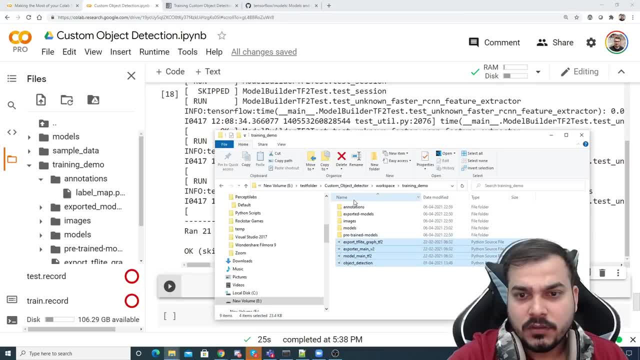 get uploaded. let's try once again inside my annotation folder. so if i go inside my annotation folder, this is my train and test dot record and i don't require it also let. let me just keep it away. i don't require it right now for this particular folders, but i can see all the other. 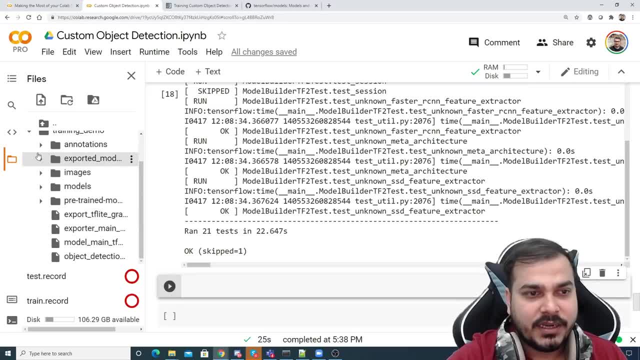 folders that are present amazingly over here, right exported models. then i have these images, you know, and probably i have this models and everything now inside my images. i will create two more folder. one is the train, okay, just to keep my folder structure intact, and the next one will basically be my test. so these two folders are basically required, uh. 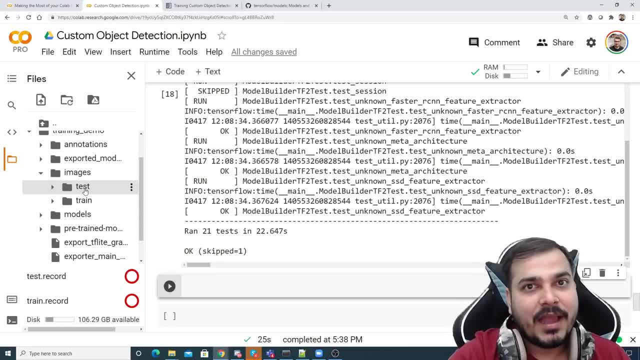 and when i'm why i'm using this particular folder? because this folder will actually have all the annotation images with us, right? so train and test now. let's go and annotate the images. now. for annotating the images, what we have to do is that i have already kept all the images in. 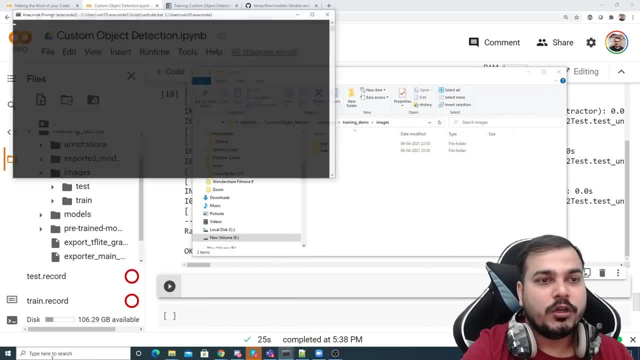 the folder, so i can just drag and drop them into my folder and i can just drag and drop them into the folder and i can just drag and drop them into my folder and i can just drag and drop them into inside this image folder and for annotating it. first of all, i'm going to quickly. 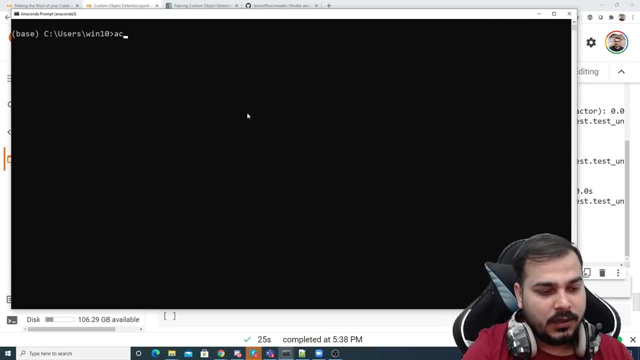 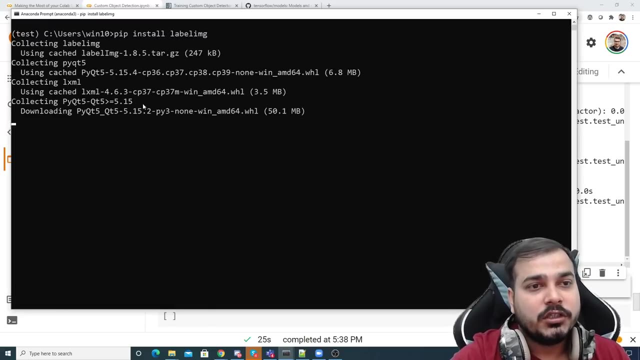 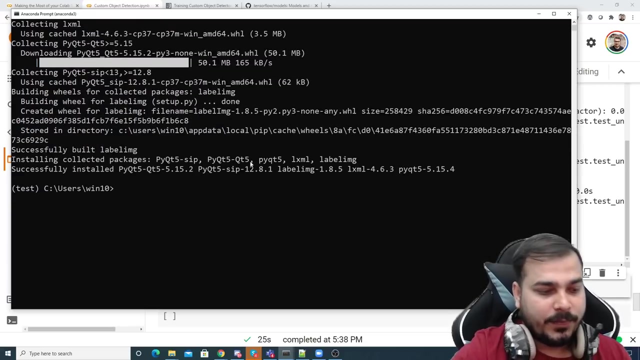 go to my environment and probably install label img, because i'll. i'll just show you how to install the label img. so for that you just have to write pip, install label img, and now the installation will happen quickly. okay, so installing completed package. perfect, now the. now the installation will happen quickly. okay, so investigating is completed. now this is done. what i'm 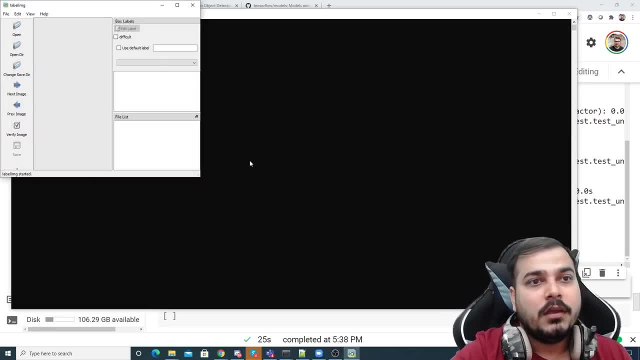 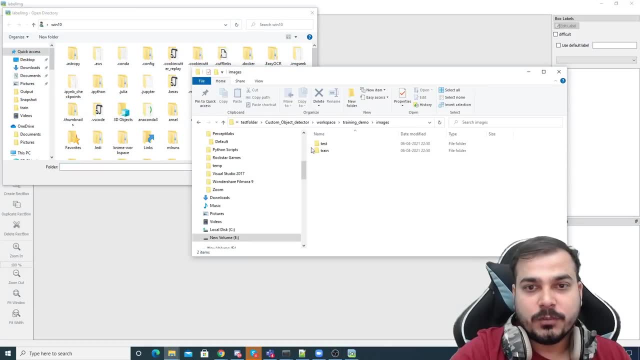 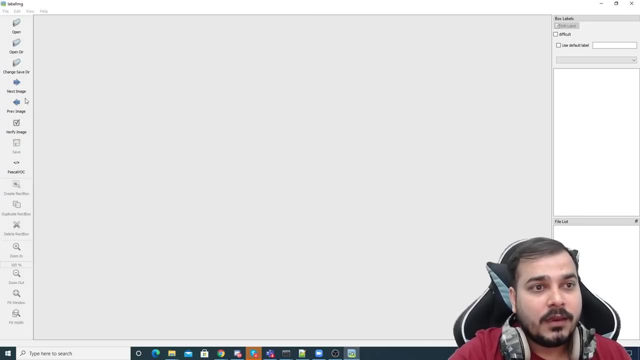 going to do? i'm just going to call label img and execute it. so here is my label img. over here i'm just going to open the directory with all my images folders. so suppose if i want to go with training, i will go and open it so that i will be able to open my all training folders. now let's go. 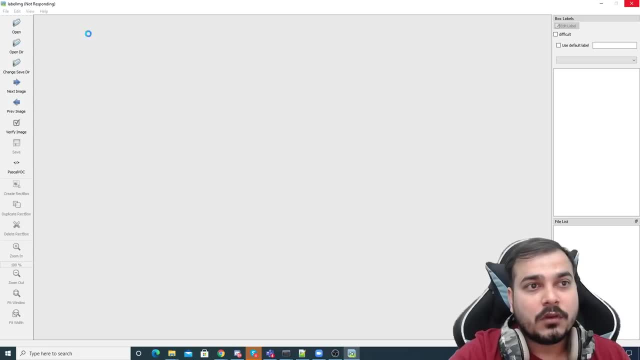 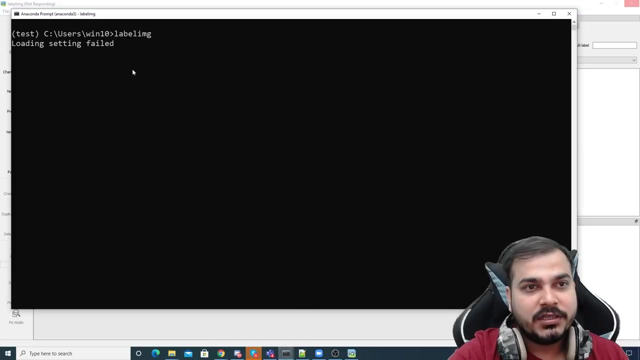 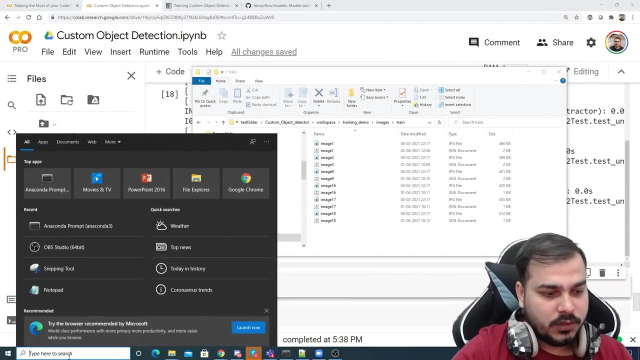 and okay, this is not responding. still, it may take some time. also, okay, let's see, because i'm trying here, i really want to show you how to do the annotation. okay, not a problem, let me just restart this. probably. let me close this quickly. now what i'm going to do. i'm just going to again open anaconda prompt. 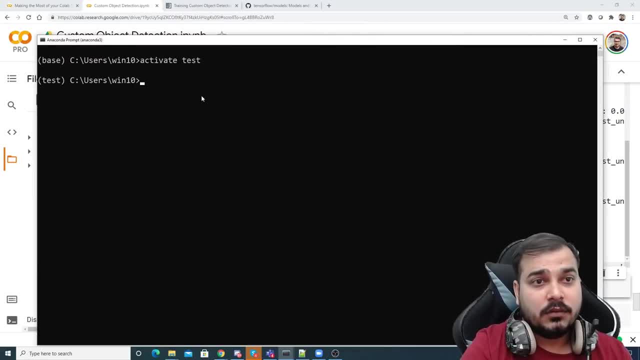 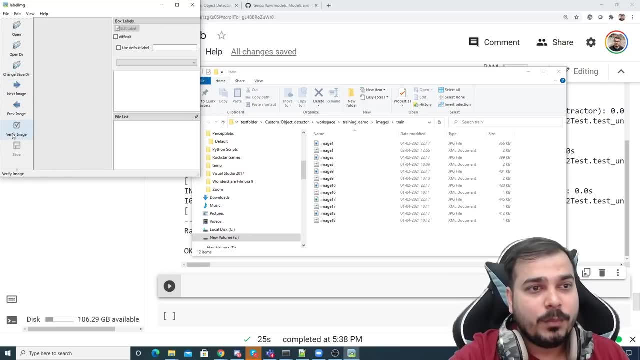 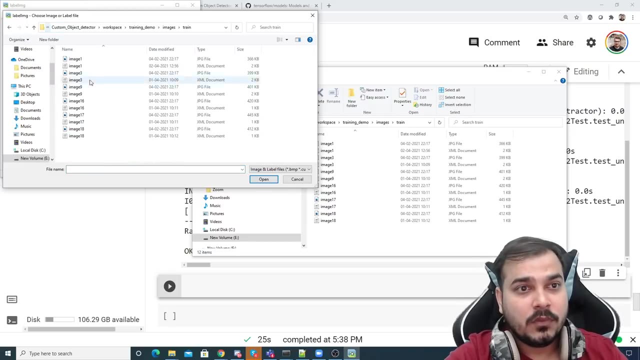 activate test. okay, and just i'll write label img. i don't know why it got stuck previously, right, so here it is. let me open one. i'll just show you one example, guys, quickly, so that you will be able to understand. suppose, if i take this image one now, this is my image one, guys. okay, this is my. 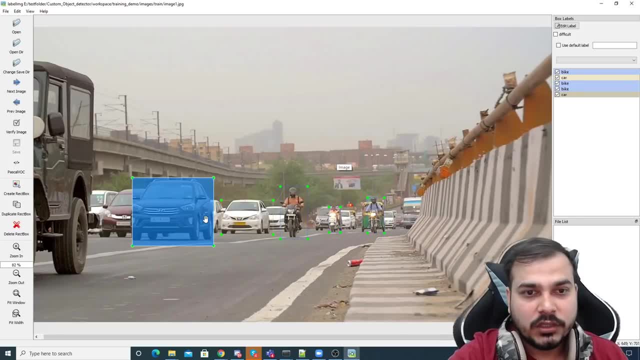 image one how the annotation needs to be done. i'll just try to give you an example. okay, suppose i see there is a bike car and all so here you have an option which is called as create rectangular box. suppose let me delete this once. okay, suppose i want to annotate this specific image with respect to cars. i will just go and select this. 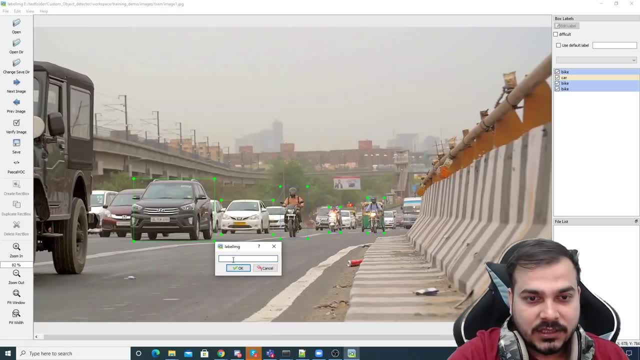 entire thing like this, right, and then it will ask me what label i want to put. right, you have to make sure that you remember this particular name. later on it will be useful for us to create this, so i'll just click on okay car. so here you can see it is ending added. then you have to save it. okay, save. 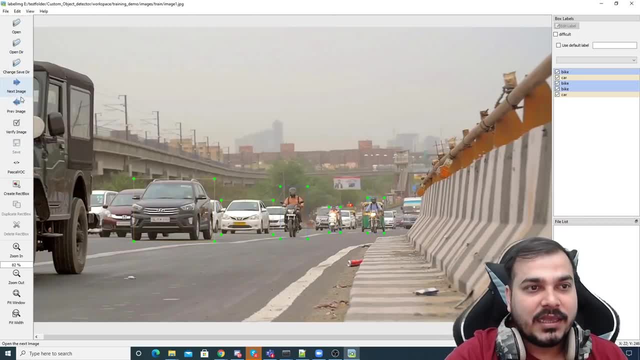 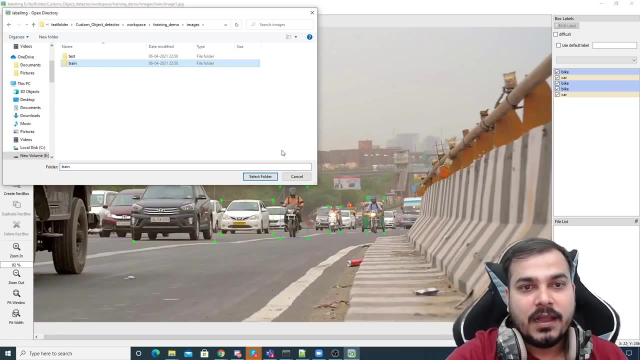 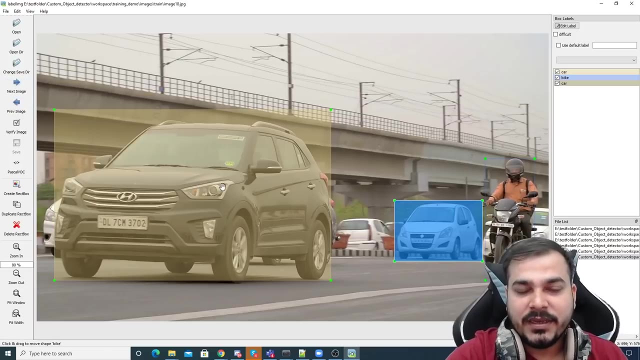 this as image one and this xml will get replaced like this. you have to do for every images, guys. how do i find out? for every images? probably. let's see this. i'll select this. i'll select this now whenever i go next, you can see for every images. i will try to annotate this. see, this has been entered by car. this image, this image. 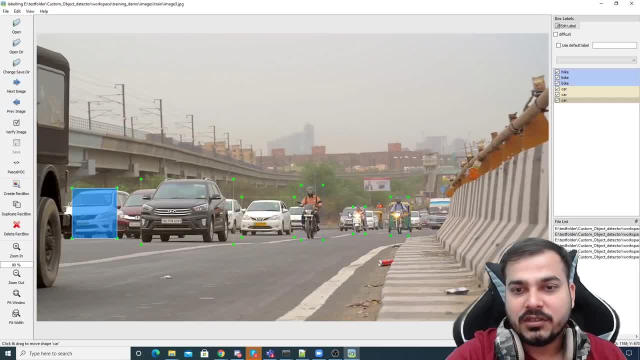 everything we have to do, this specific annotation, right, with respect to bikes and all. probably you have to annotate autos, rickshaws, anything that you want to do, it will be possible. okay, so this is what you have to do. after this is done, you can close it and then, when you see this annotation, 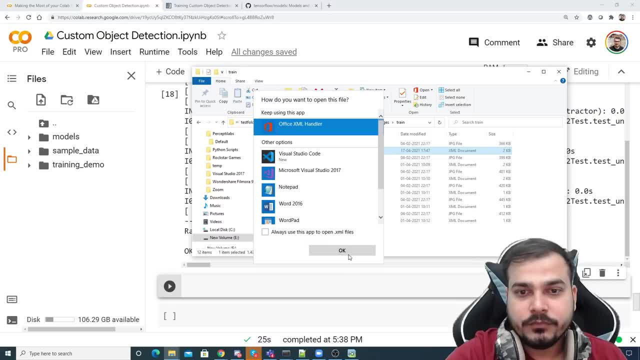 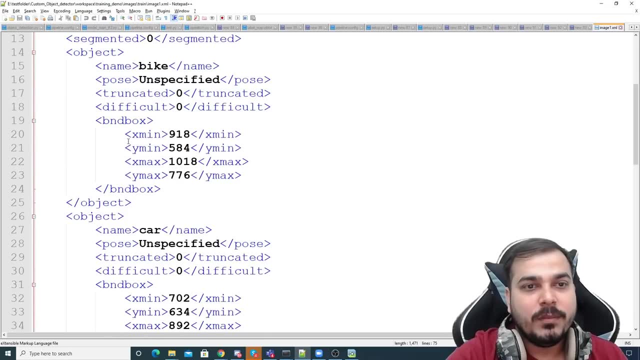 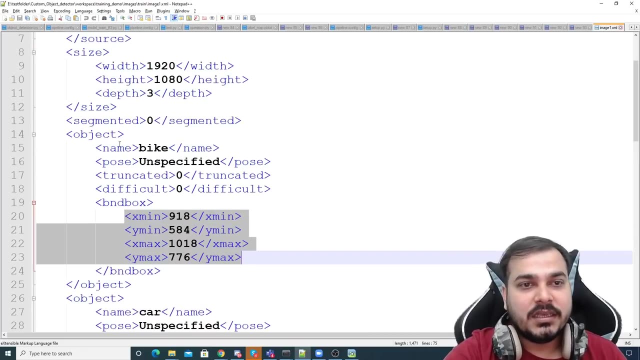 what will this xml file, if i just show you right, if i just show you the xml with respect to the notepad plus, plus, here in the xml file, you will be having this: all values, the bounding boxes, values with respect to x mean, y mean, x max, y max. everything will be right. see here, probably. 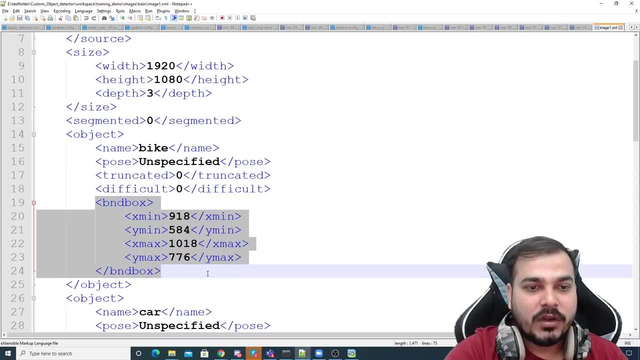 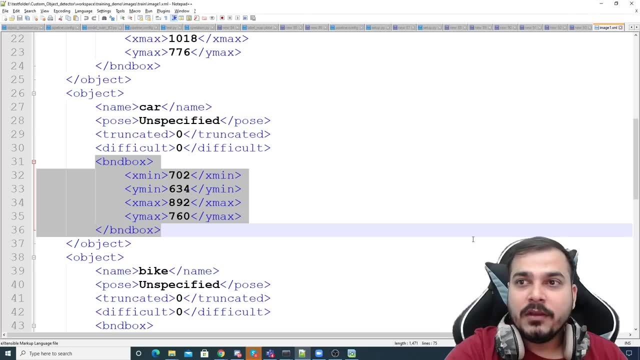 one annotated image is bike, then you'll be getting the bounding box coordinates. similarly, if you have annotated car, you'll be getting the binding box uh values with these four values, right? so i have all of these values, right? so that's why i'm using the xml file. so that's why i'm using the xml file. 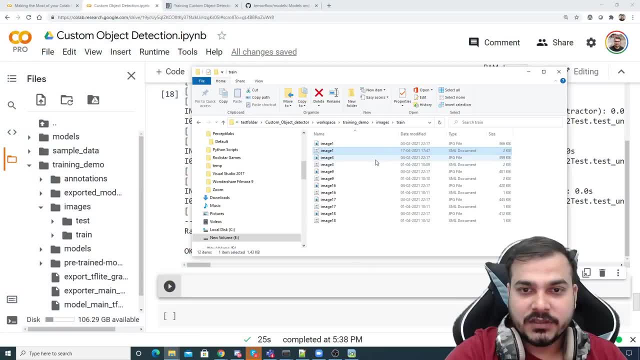 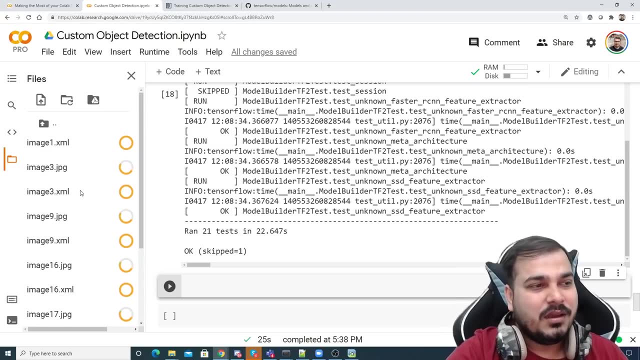 now what i'm going to do. quickly, i'll go over here, i'll go inside this images folder and then inside my training folder i will upload all these particular images. okay, so i'm just going to upload all these images inside my training folder and, yes, you can also do it from your. uh in the 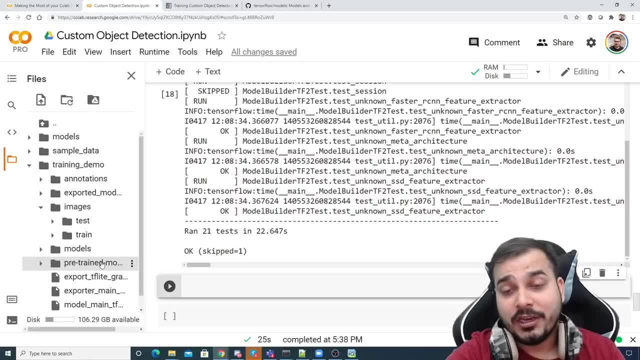 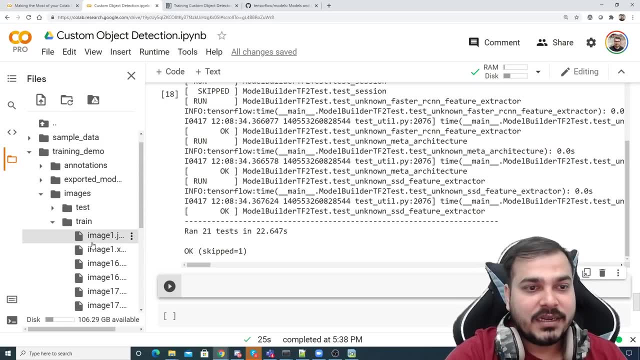 google collab also. nothing like not much difference, but yes, uh, actually google collab pro gives us longer run time, sorry, longer. if you don't do anything, then also the session will be hold on. so here is all my files that is present inside here. okay, now. similarly, i'll try to upload it for the 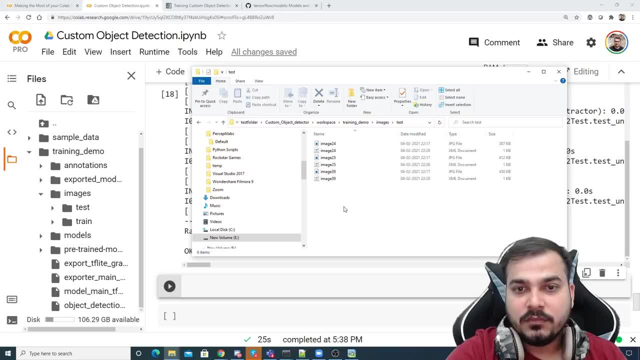 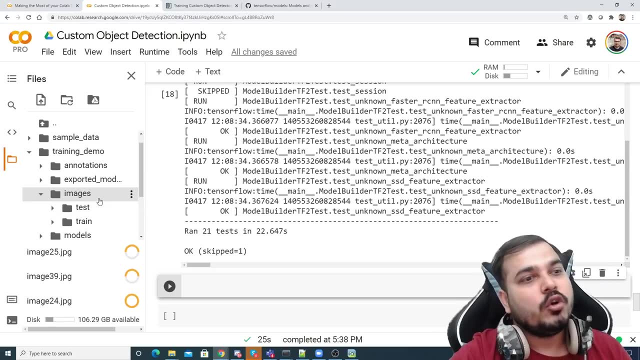 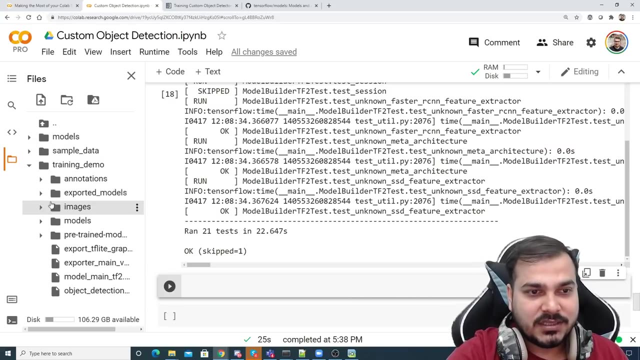 test file. so i'll go over here images test this entire thing and i'll just move it over here. well, and i have just taken very less number of images, uh, just to show you how to quickly uh create this custom object detection. i'll also run it for less number of times. so, guys, this too is. 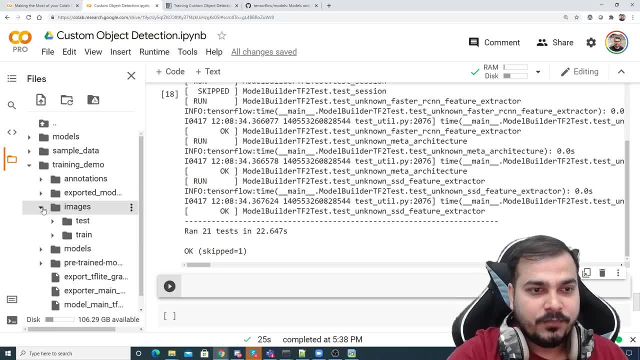 done so. in my images i have all the files. i have everything now in my exported models. here you can see i don't have anything. in my models also i don't have anything, and in my pre-trained models also i don't have anything. now let's go do one thing now. what i'm going to quickly do is that. 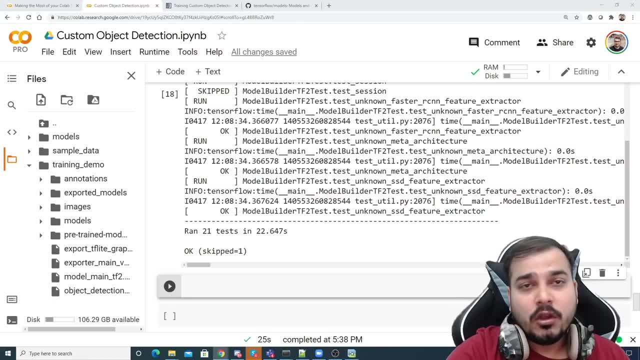 with respect to my pre-trained model. you know i need to copy a pre-trained model from the object detection or from the tensorflow model zoo, and for doing that i'll just show you how to do it so that it'll be very, very efficient for you, and you should also follow this specific thing right. 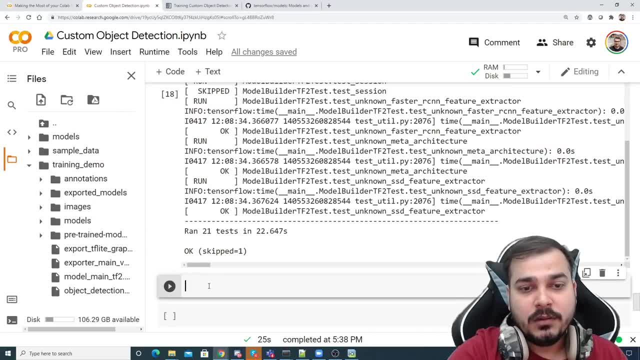 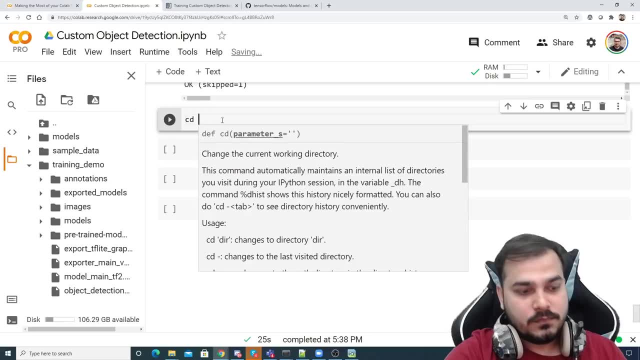 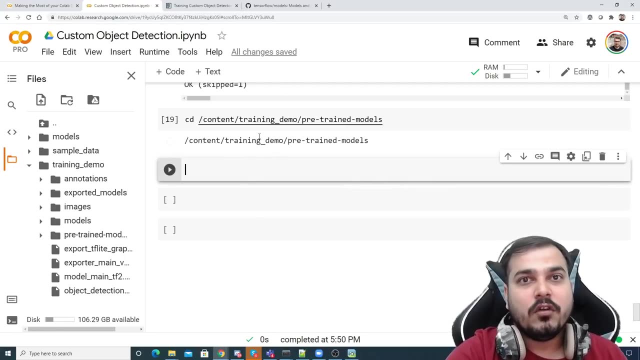 now, first of all i'll just go and take this path of pre-trained model and i will just run write cd and i'll paste it over here. okay, so i'm going inside this pre-trained model because inside this path only i have to download my tensorflow model zoo library. so if i go and 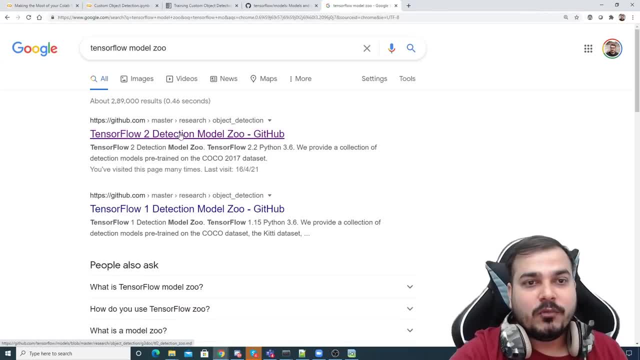 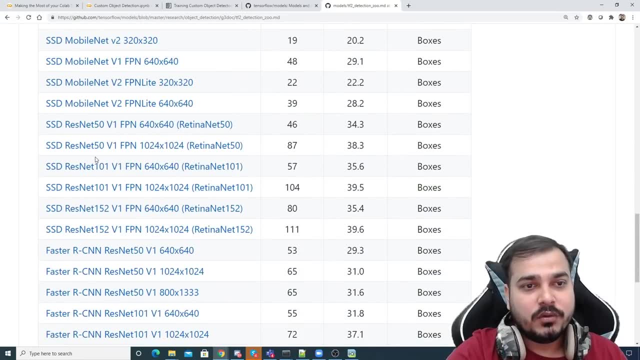 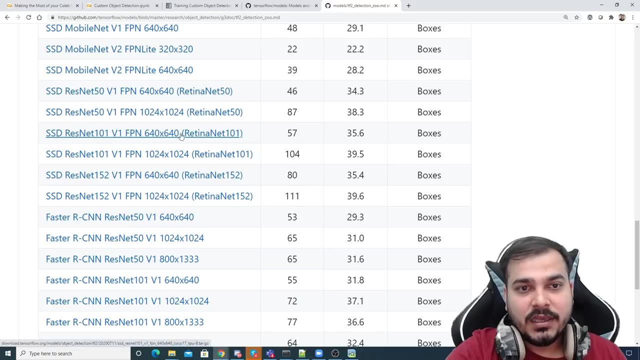 search for tensorflow model zoo. okay, i'm going to first of all use this particular model and then do a transfer learning on this right? so for this case, what i'm going to do, i'm just going to take one of this particular model for this particular scenario. i'll take resnet 101 640 640 retina net. 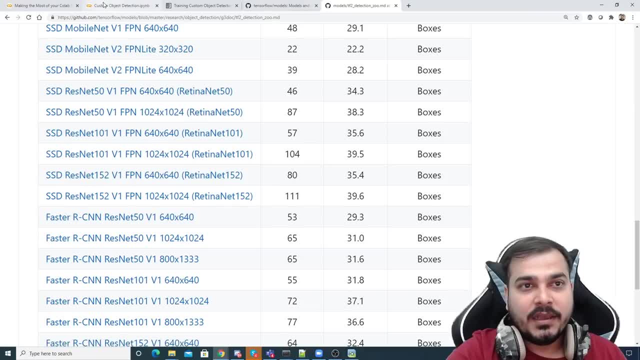 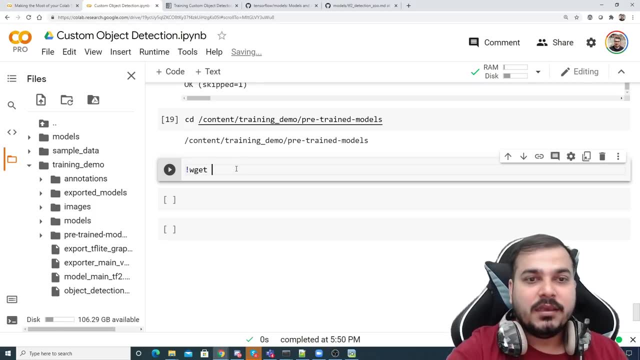 101, so i'm just going to copy this link address and, in order to download it, since google lab in the back end linux environment is there, i'll try to use wget path and then i'll just paste it. now. what this will do is that this will directly download this zip file inside this pre-trained. 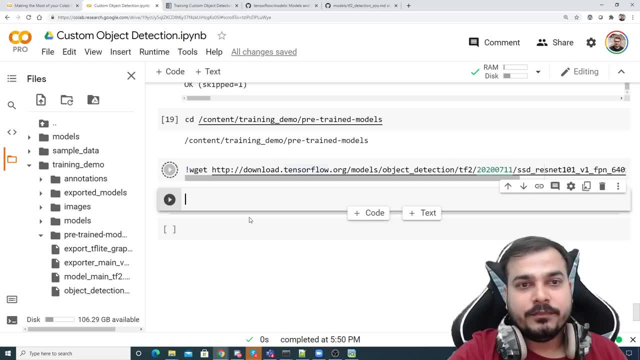 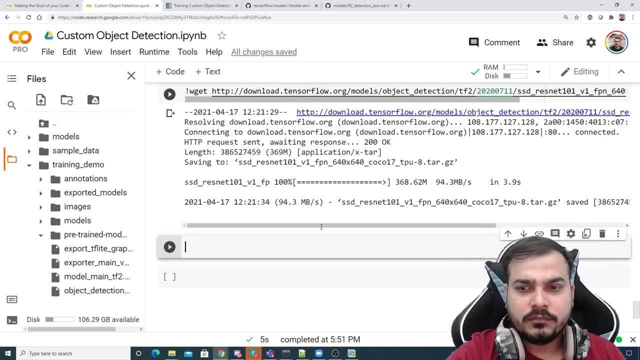 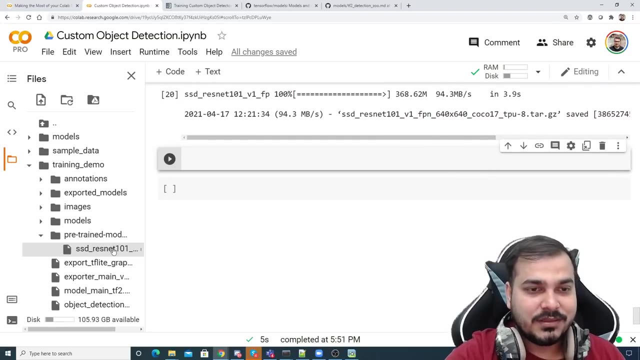 folder. okay, pre-trained folder, so let's execute it. okay, so here you can see that it has been downloaded. it has started downloading. it will take some amount of time. okay, the downloading has done. now, if i go and see this particular folder here, you'll be able to see this. this will be still in the tarzz file. 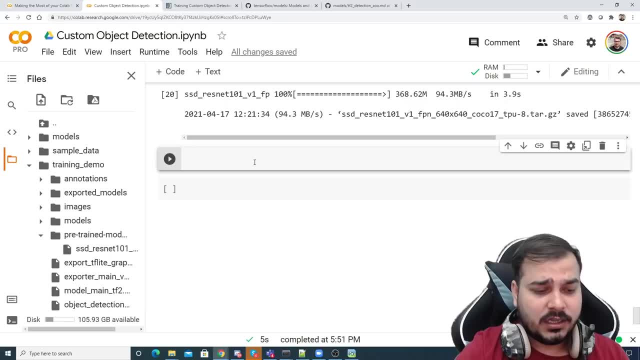 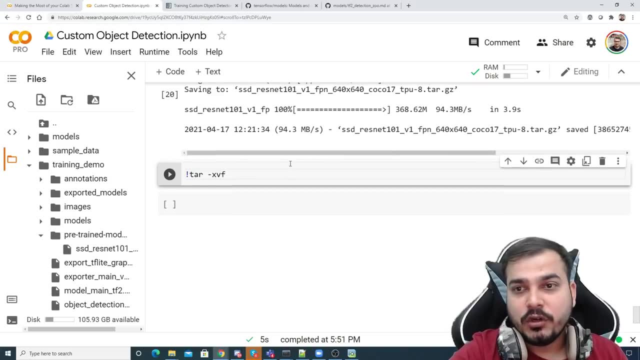 now, in order to extract it, i will be using another command, which is called as tar xvf. and then what i'm going to do? i'm just going to give the tar file name right. so i'm going to give the tar file name right. so i'm going to give the 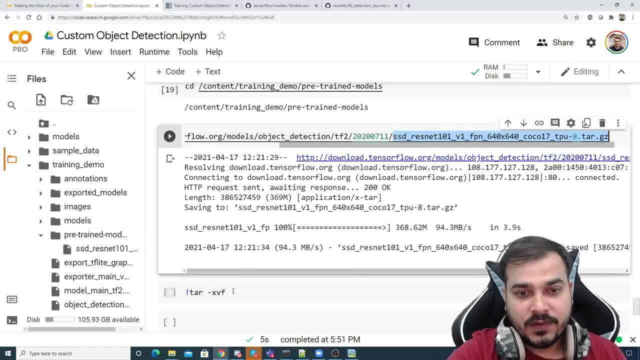 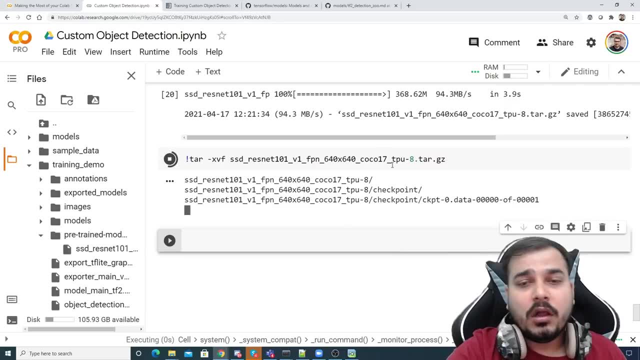 tar file name. right, so this will be my tar file name, the zip file name. so here i have executed it, and now this will create a folder inside this where it will extract all the things that are present inside this particular zip file. okay, so now, if i try to execute it again now, here you can. 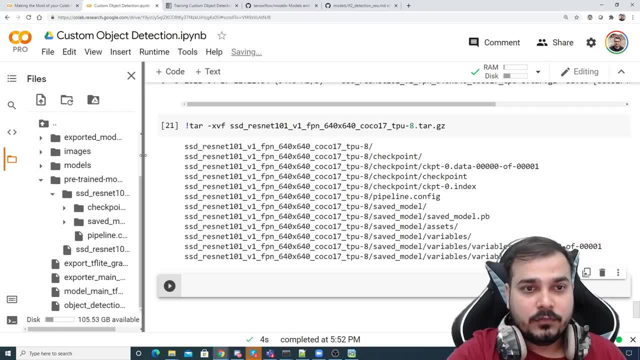 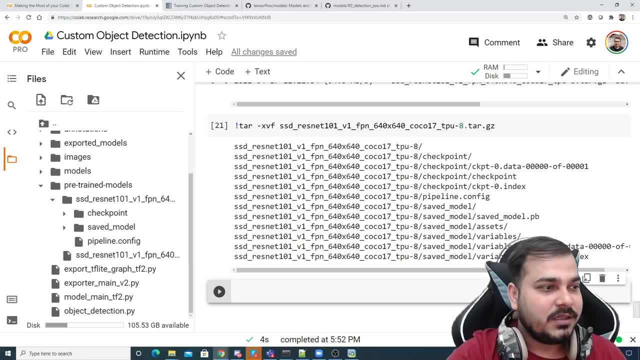 see that. this is my folder. that has got extracted right. see this, this is my folder. this is having checkpoint, same model and pipeline config. perfect, right, we have done this. particular steps now coming to the next step, with respect to a pwd. uh, again now, if i go and check out my pwd, okay, and here you'll be able to. 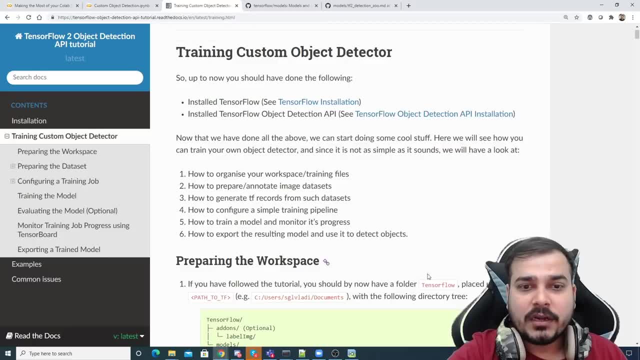 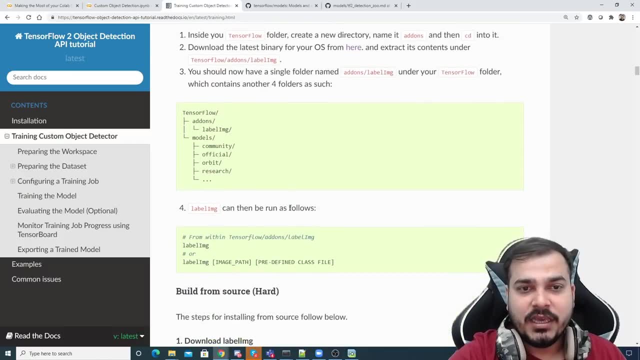 see that i'll be having this specific folder right now. let's go back to my training customers. so we have done this, we have done the annotation, we have prepared the data set with the help of label img. everything is ready. now you have to start the process from here, okay, so let's see, see this. 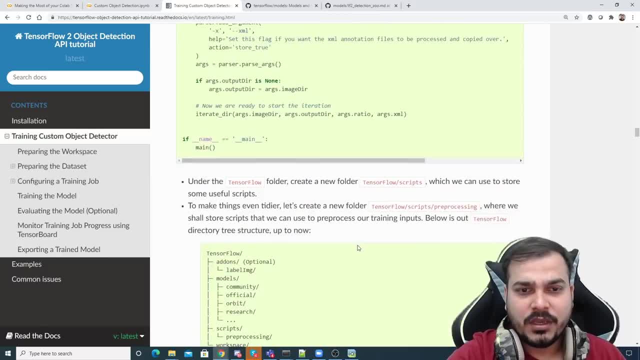 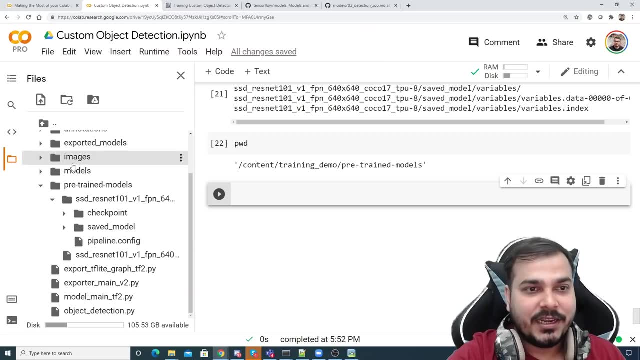 annotation. everything is done, everything is given over here, guys, step by step. okay, just follow this. first of all, i need to create this label map. now where this label map is basically created. if you go and see my annotation folder there, i have already put up this label map dot pbtxt. now, if i 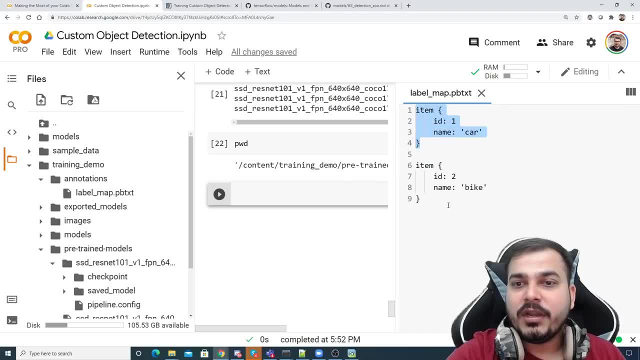 go and see this label map over here. this is the format of putting the number of classes and, according to the images that i have annotated, i just have two classes: one is car and one is bike. okay, so this car- bike will be there. uh, this annotation, i will try to give it to you, so you 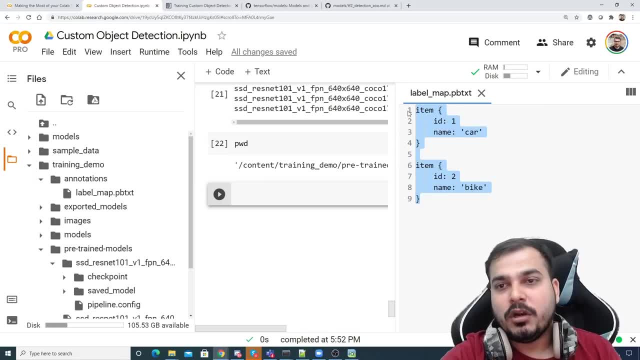 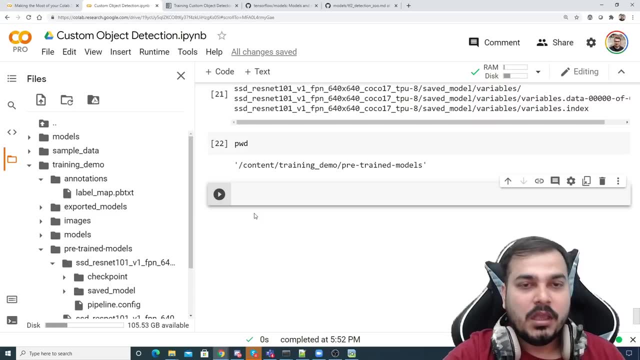 don't have to worry much about it. okay, so this label- map dot pbtxt- i have actually created and it is inside the annotation folder. perfect, now. coming to the next step, what we have to do now is that, if i go over here, we have to create this. 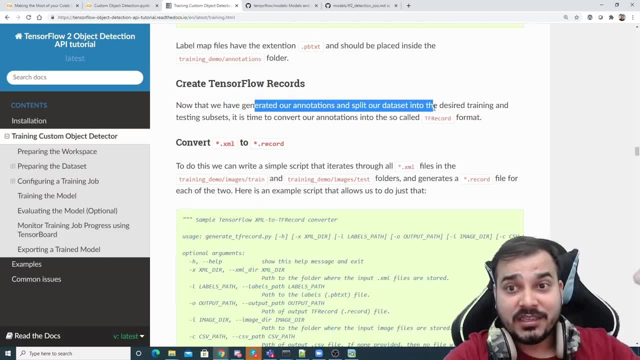 tensorflow records. now we have generated our annotation, i've split our data set into train test split also. now it is time to convert it to tf record. now, inside this- guys, you have already seen that inside the test data set- you have this xml file. right, it has bounding boxes, coordinates. 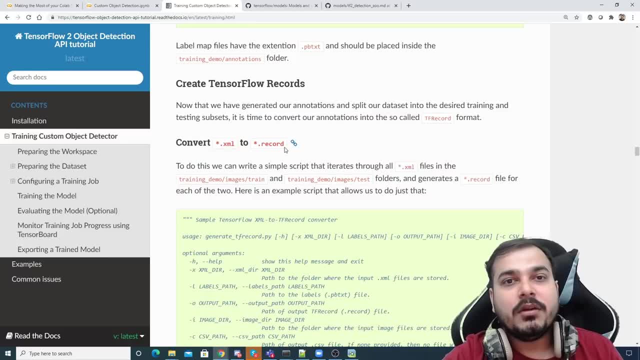 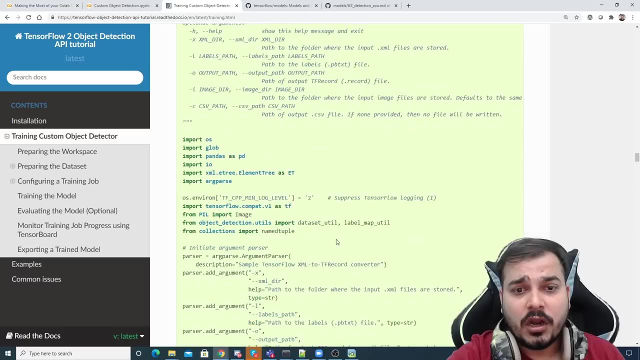 dot record. okay, so tf record format that will be able to understandable by the training model that i'm actually doing, you know. so we need to convert this into this. that basically represents our data sets, right? so in order to do this, what we have to do? um, we will be running one file, which is called. 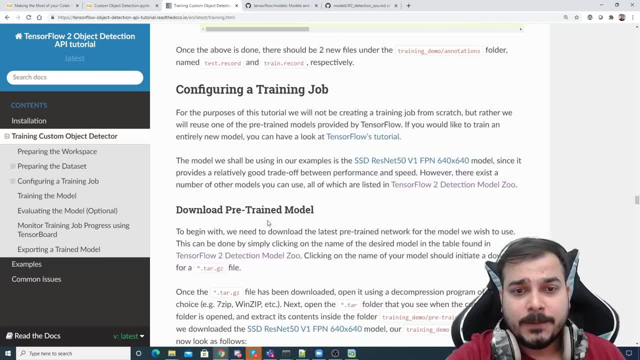 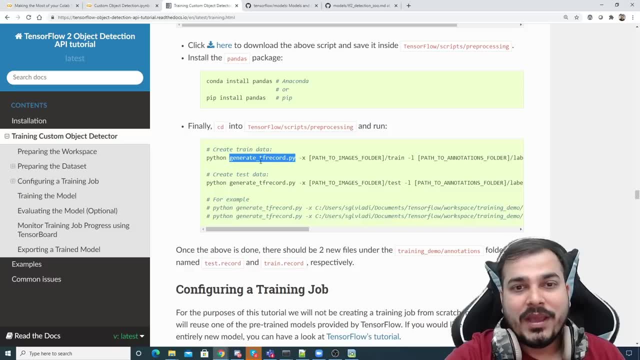 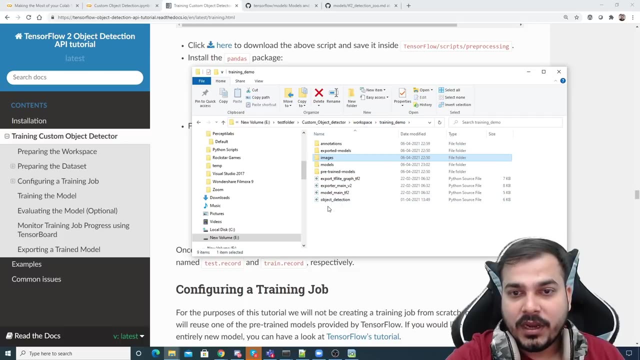 as which is called as uh. if i talk about this particular file, just give me a second. that is called a generate underscore tf record dot py. now, where is this generate underscore tf dot record product py. so if i go over here you can see that uh, one of the file that i've actually kept. 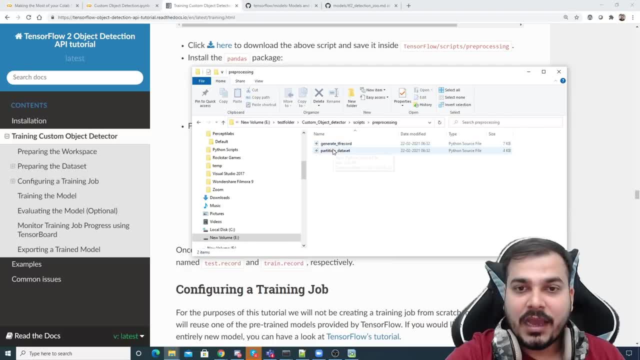 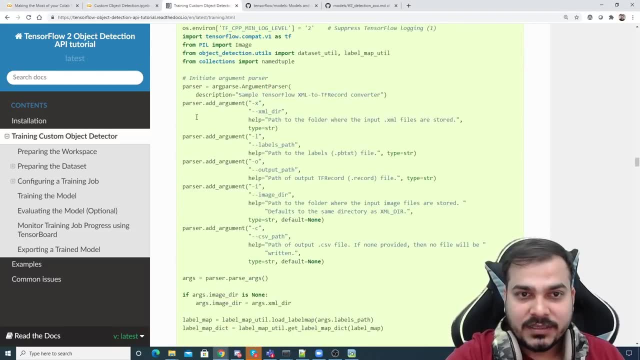 will probably be in the scripts folder. so here i have. i have this particular file generated underscore tf. record now where this file i got generated from. i just copied this entire code. see this entire code. i've just copied it, okay, pasted it in a dot py file and i've kept that. 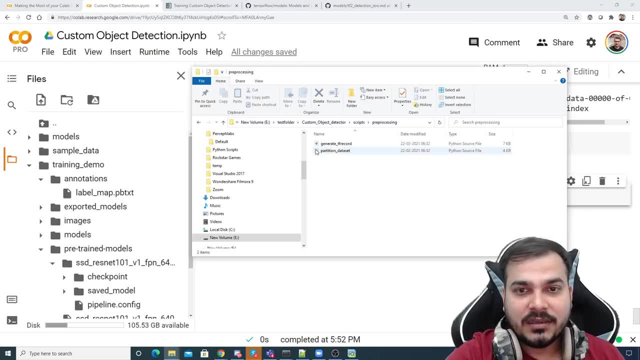 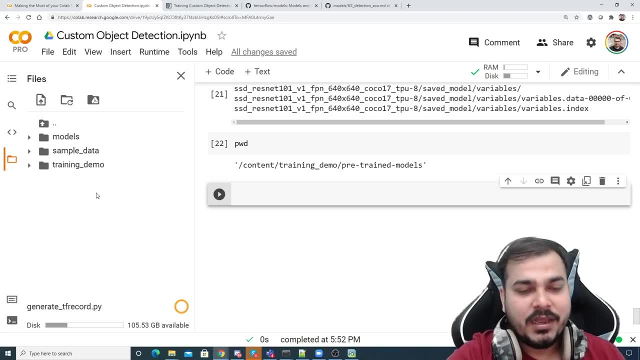 file ready. okay, now what i'm going to do. i'm just going to add this particular file inside my training demo folder. okay, so here i'm just executing and copying it in my training demo folder. now here is my entire file: see generate underscore: tf record. okay, now what i have to do? i have to just go inside this. 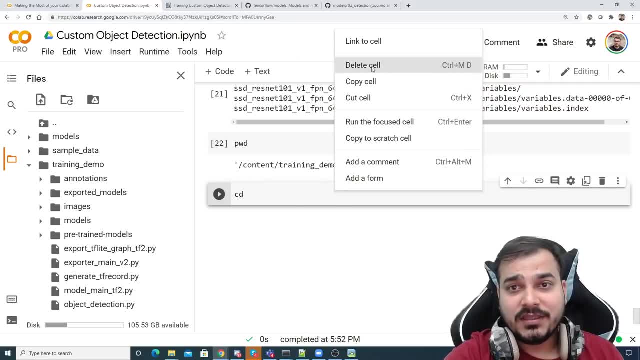 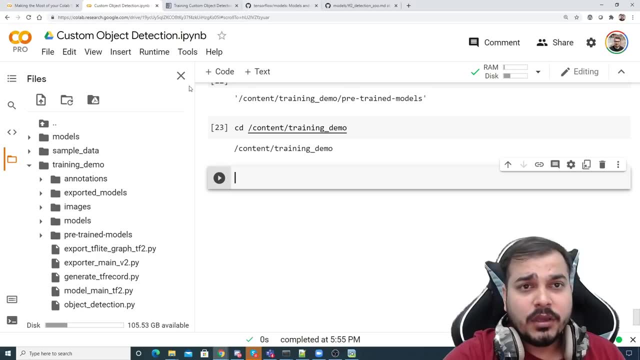 particular path. so i'll write cd because i have to execute that particular command. right cd and execute it now. i'm inside my training demo now. in order to execute that particular file, i just have to copy this entire command. so i'll just copy this: create training. 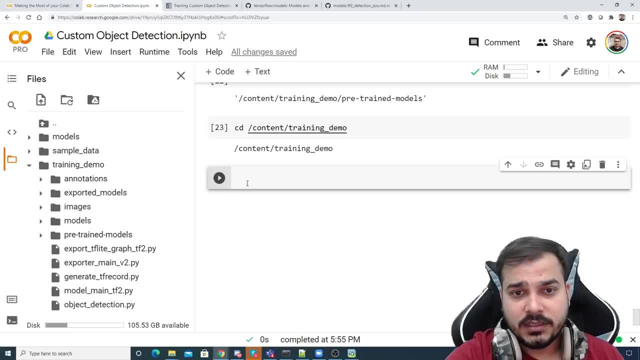 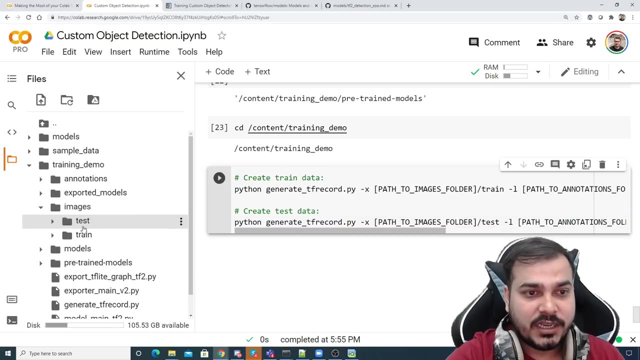 and test. okay and go inside this. okay, now see this: if i really want to create the train tf record, first of all i have to execute python: generate underscore tf record dot py. path of images folder slash train. now what is my path of the images folder slash train? i'll just execute this copy. 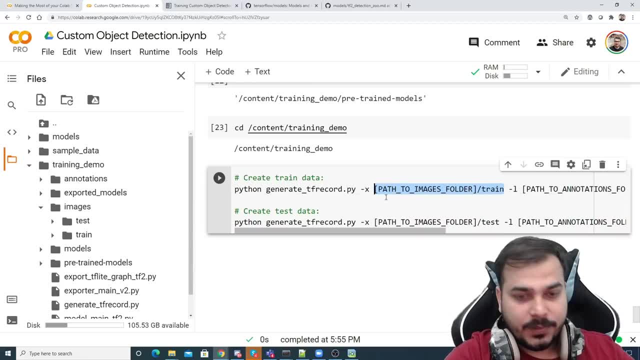 path and go over here, paste it over here. right, so i'll paste it over here. so train path is there. then it is having: it is asking me label underscore map dot pb, txt path. so that's is obviously. we know this and it is inside my label map, so let me just execute it quickly. 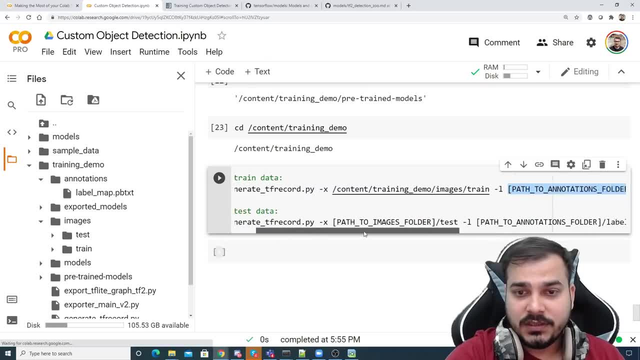 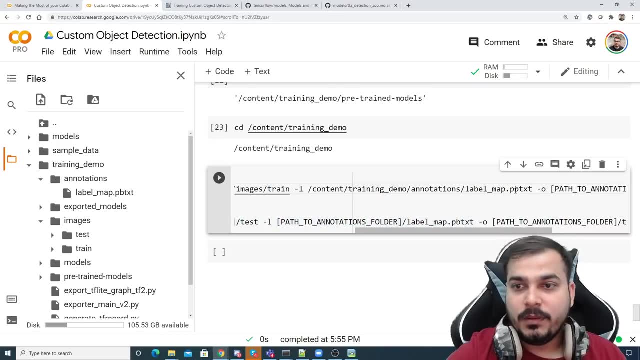 see, guys, you have to be patience with respect to uh this because, understand, you have to follow this particular steps, right? so i'm just going to remove this and this will be my label: map dot, pbt xt. then final path is basically with respect to train dot record. now, what i'll do is that i'll try. 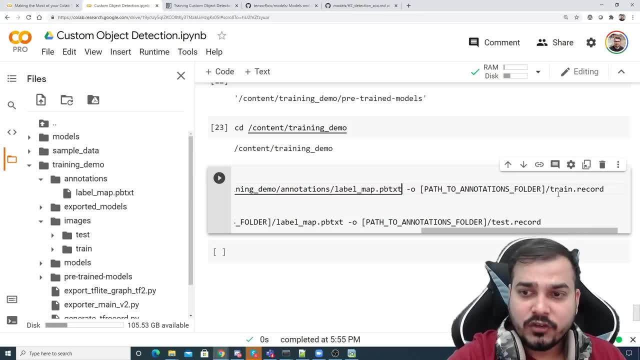 to uh save this particular file. this is the output file. i'll try to save this inside my annotation folder only. so copy path and i am just going to put this inside over here. okay, perfect, all the steps have done. now, similarly, i have to do it for the test one, so i'll copy this. let's see the test. 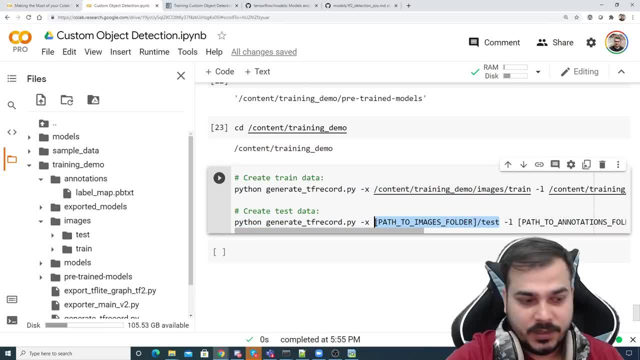 path. so test path is here, so i'm just going to copy and paste it over here. done first step. then i have this label underscore: map dot, pbtxt. again the same path. whatever i have written over here, let me just go- and oh, it's moving very fast, let's see. so i'm just going to use my keyboard. 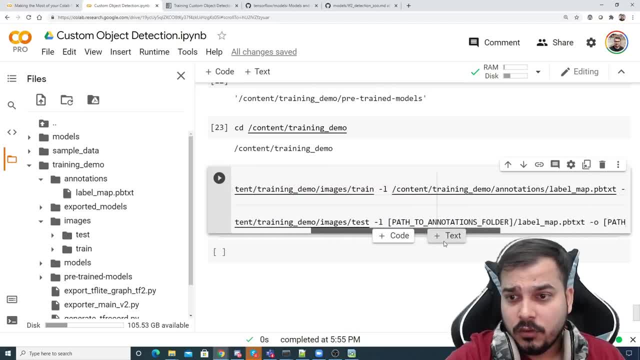 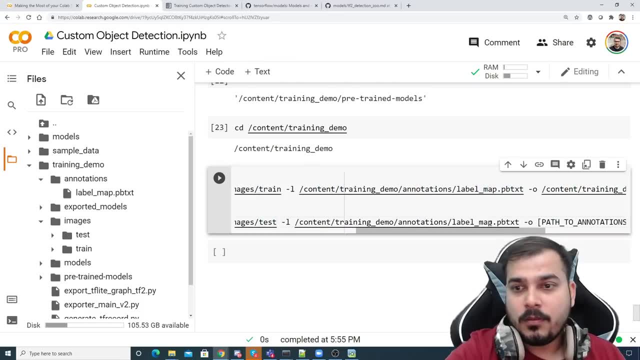 because sometimes it moves a lot right. so here you have. okay, then final path is basically with respect to my threcord. so again, i'm just going to use this annotation path. so annotation path and what i'm going to do, i'm just going to remove this. so three paths i have to give over here you. 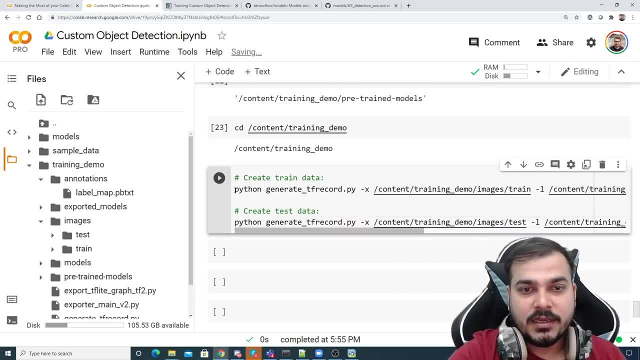 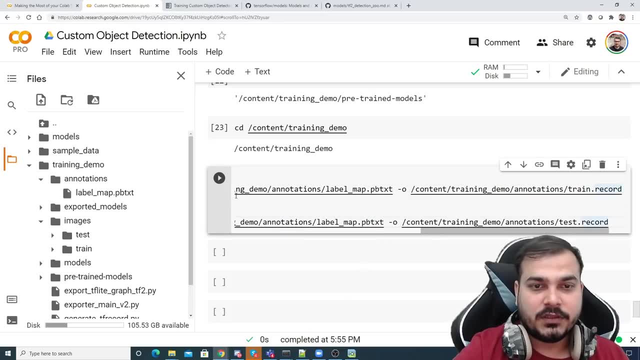 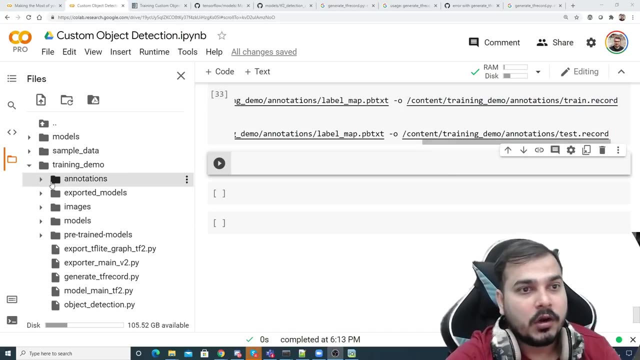 have to update it. okay, with respect to this, now, since i'm running python with this specific file name, what i'm going to do, i'll just write exclamation, because usually it takes this particular car. so, guys, after executing this, let us see that, whether trainrecord and testrecord, 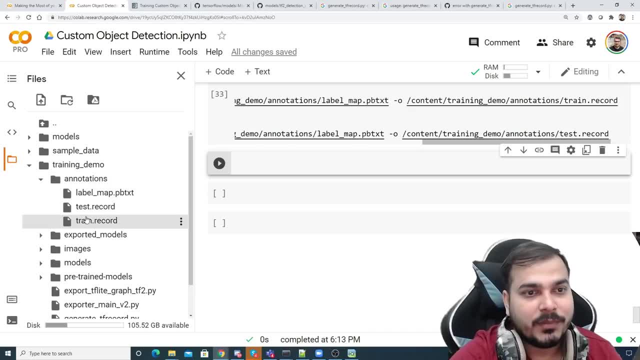 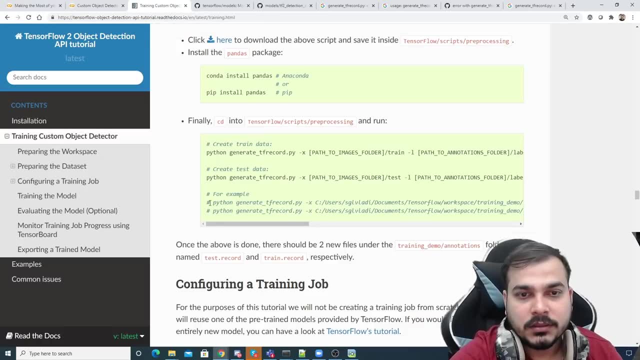 has been created or not. so you just go to the annotation folder. so here you can basically see the trainrecord and testrecord, right? so this particular file is there now. coming back to our block, uh, this step is basically done. now we need to configure a training job right now in order to 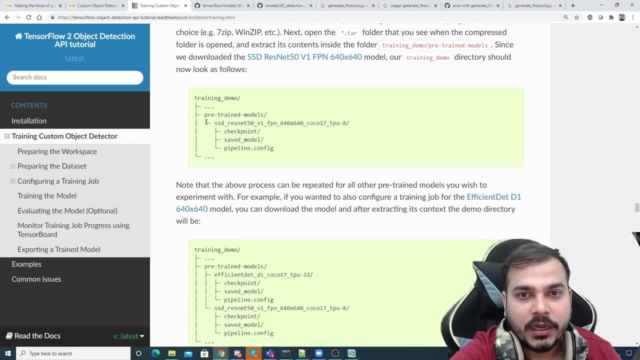 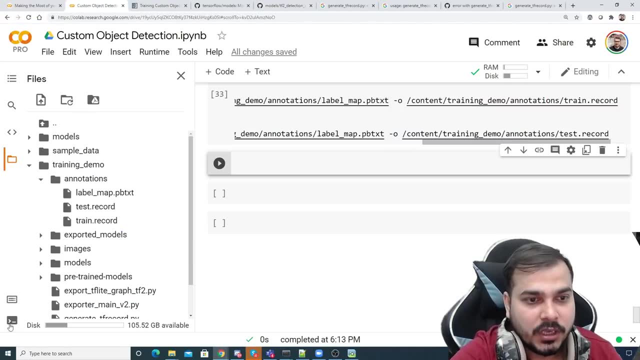 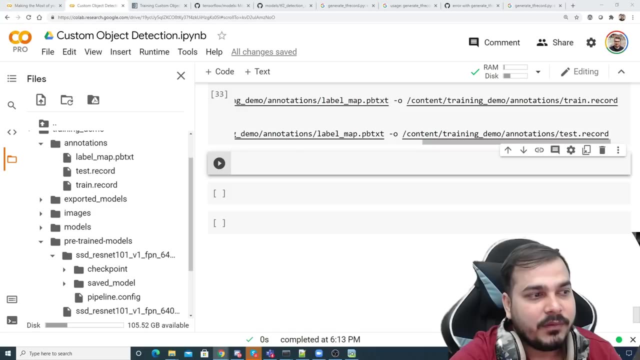 configure it. what we have to do is that we will try to create- uh, this, this entirely this- ssd resnet from the models. we have already downloaded it. so here you can basically see in your pre-trained model. everything is there right now. what we are going to do in the next step is that probably we 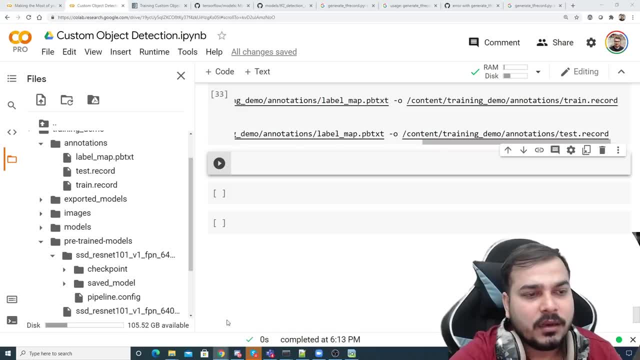 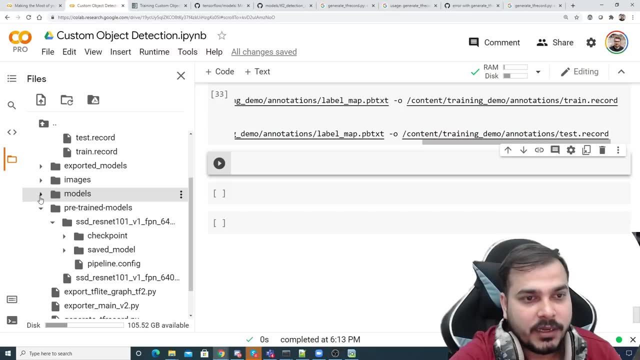 will try to create a folder for this model, and we will try to create a folder for this model, and that particular folder will basically be: uh, taking the checkpoint from this, okay, so suppose here is my specific model right now. inside this particular model, i will try to create a new folder. 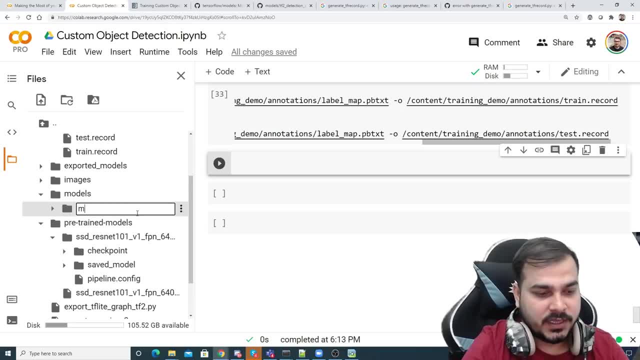 okay, so this folder name, suppose i say it as my underscore ssd, underscore resnet 101, underscore v1, underscore fpn. so suppose this is my entire model file and inside this folder i will try to create a new folder called pipeline config. okay, and this will help me start the pipeline config. 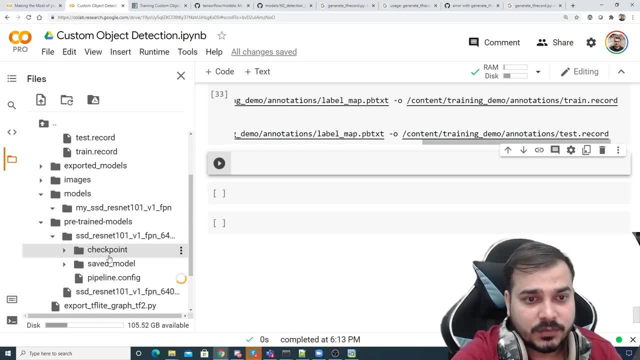 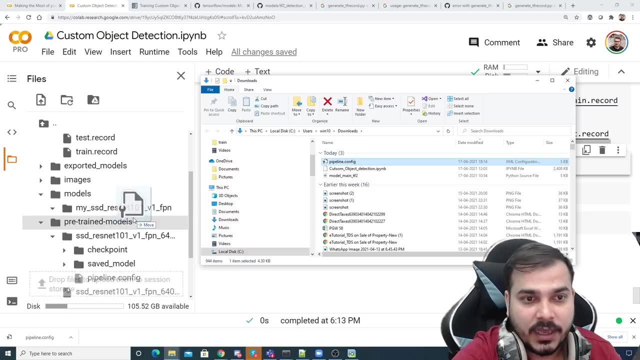 okay, i'm going to just load this pipeline config, okay. so let me download this pipeline config file, because this pipeline config file will be uh important for us. so i'm just going to copy and probably paste it over here, and now we are going to update this pipeline config from this, remember. 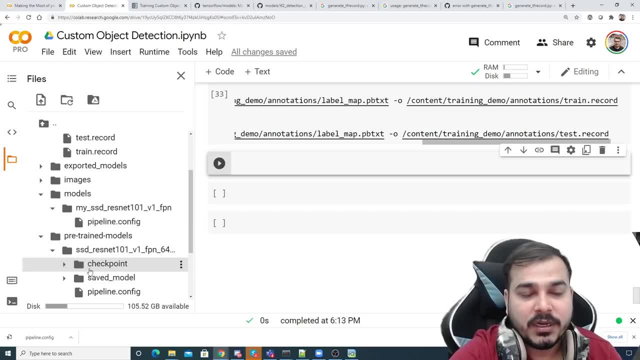 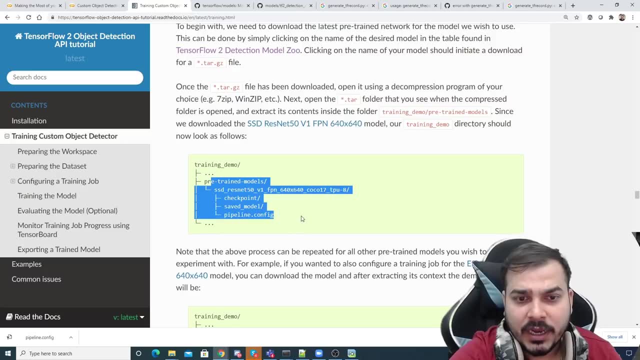 this pipeline config, we have to refer it from this particular pre-trained model, right, and that is what all the steps is basically given. so here you can see that inside my pre-trained model i am going. i already have now what we are going to do. we are going to make folders to configure this training. 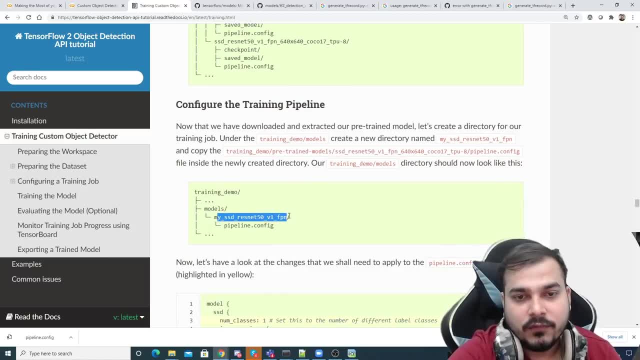 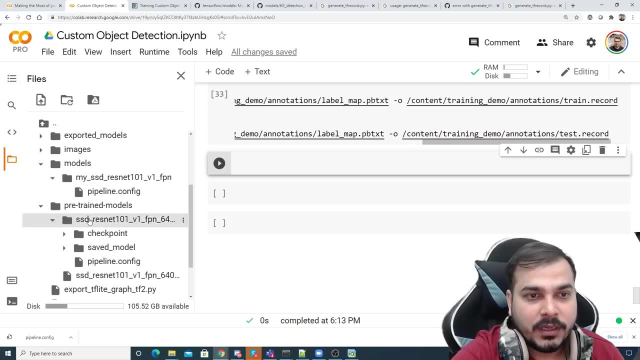 pipeline. so inside my models folder i have created one folder which basically refers that and this is basically the pipeline config. now i'll open the pipeline config. okay, i'll be opening this pipeline config that is present over here and now here. i need to make some changes now. first change that. 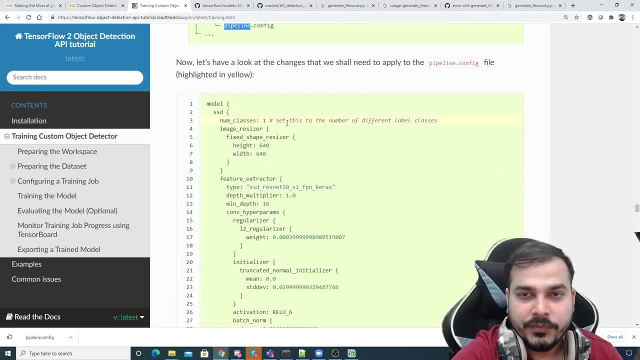 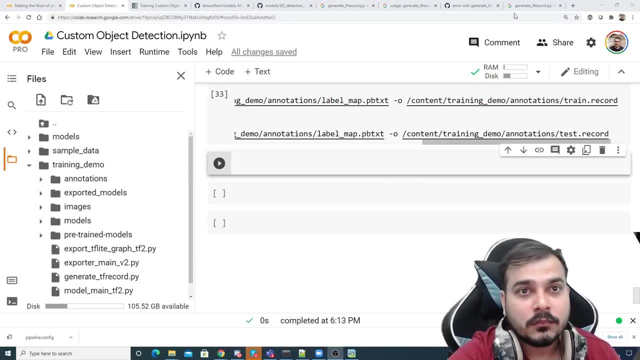 i really need to make is- and again, this changes is also given over here- okay, first change is the number of class. in my case, the number of classes will be two, so i'm just going to make it as two. so, guys, the next change that i have to do is 131 line number. so what i'm going to do again, 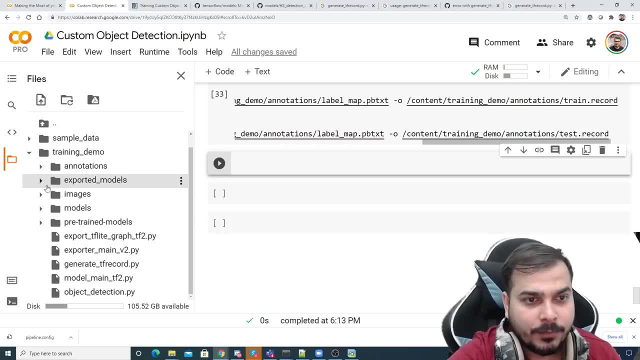 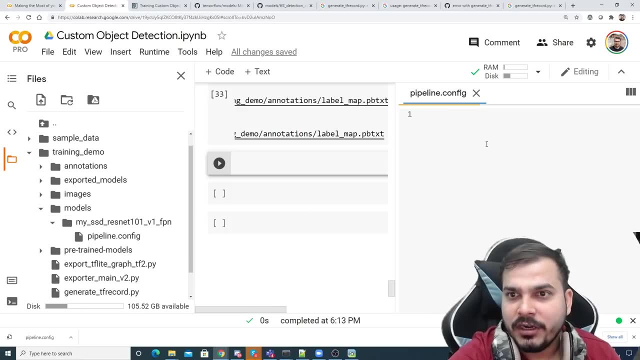 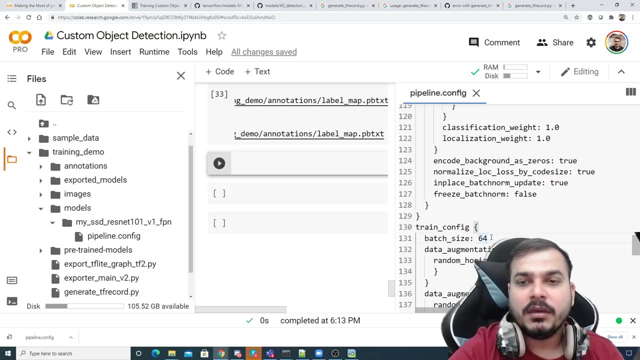 where did that go? i will just open my pipeline config, which is present inside my models. okay, so this one, the changes i have already done, i guess. so number of classes: two, and let's go to 131 line number and 139 number it 131, it is 64 bits. 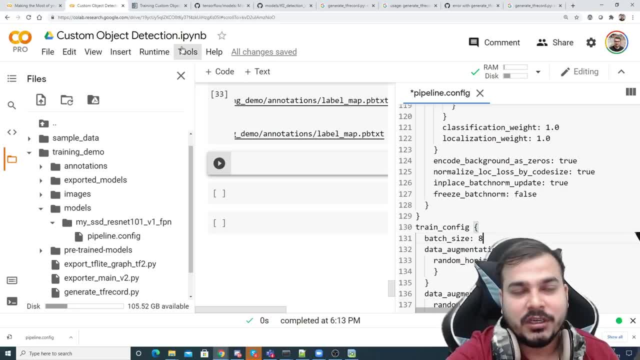 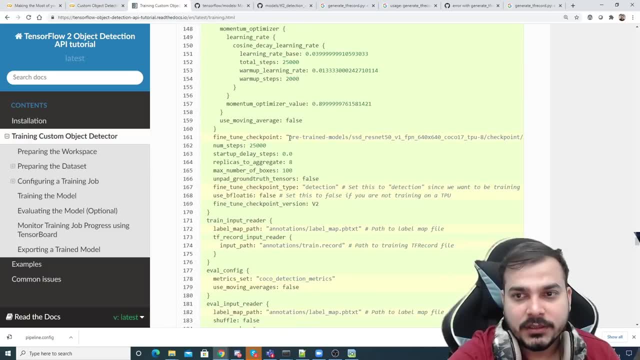 so i'm going to make it as eight, so that i don't want to give much, because, again, with within limited ram, we'll try to run it then. the next line will be basically this: fine tune checkpoints. now, in order to get this fine tune checkpoints, i have to basically take this particular path. 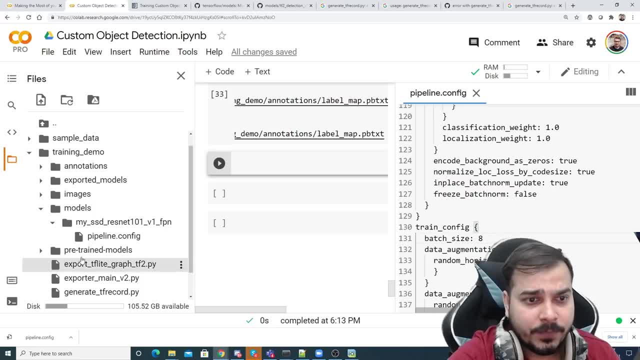 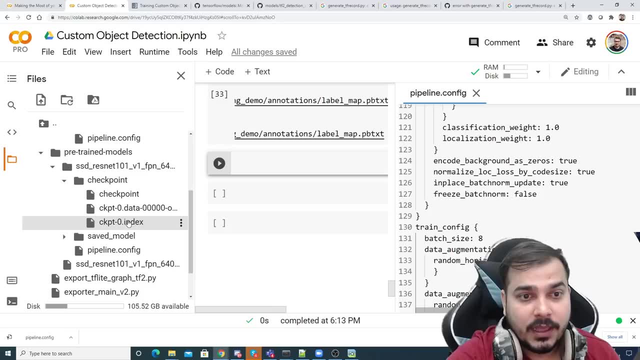 from my pre-trained model. so let's go over here and this will be my real, real train model, right from this. i'm going to refer it. so i'm just going to go over here, go into my checkpoint and then i'm just going to copy this entire path, okay, so? 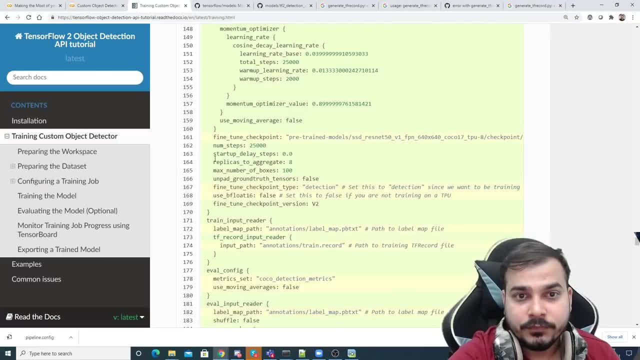 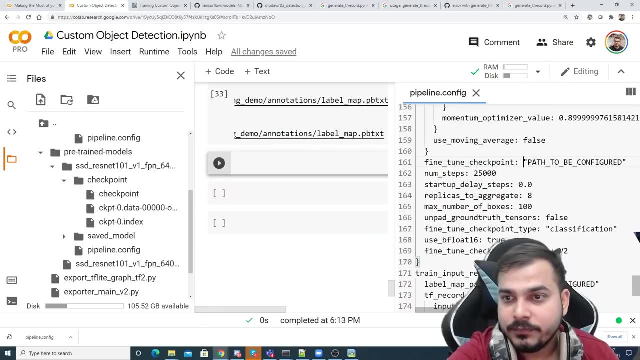 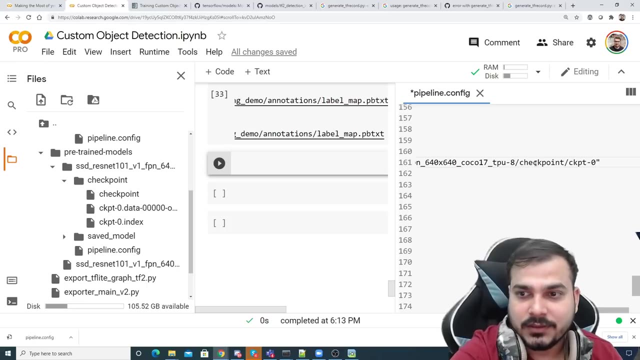 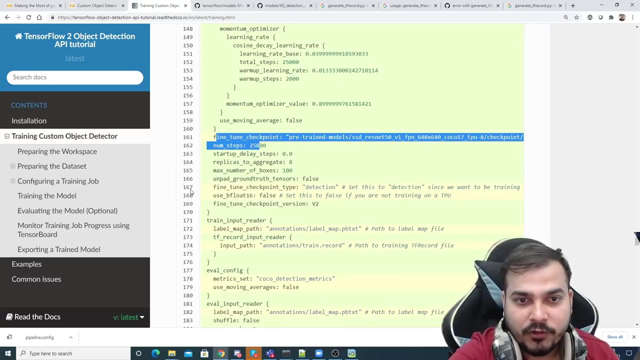 my checkpoint probably is in line number 161. okay, so this 161. i'll just go and update it. so here is my 161. okay, i'm pasting it. i'll just remove this index. okay, i don't require this index done. so this particular path is also updated. now, after 161, the changes i have to do. it is in 167. 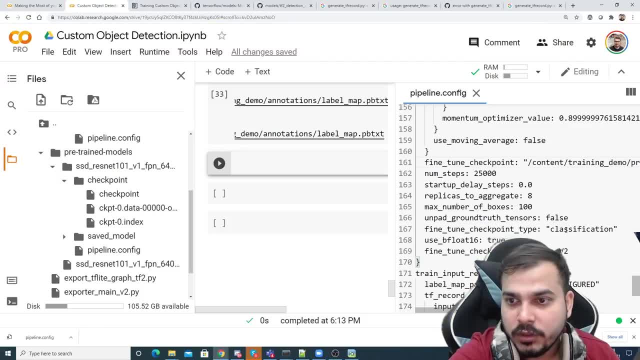 so i have to make this detection, remember, i have to go down over here. instead of classification, i have to make it detection. and the below path that shows true. this true is basically for if you only have, if you are using tpu, will keep that as true. so here, 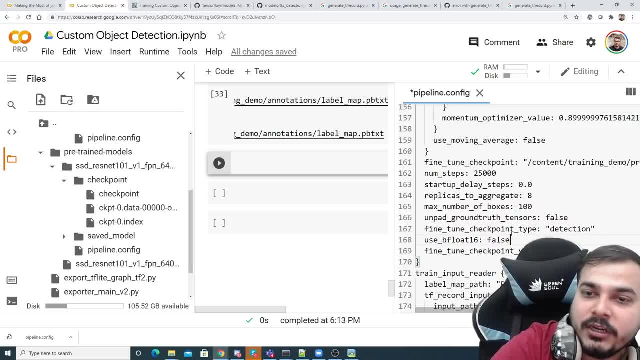 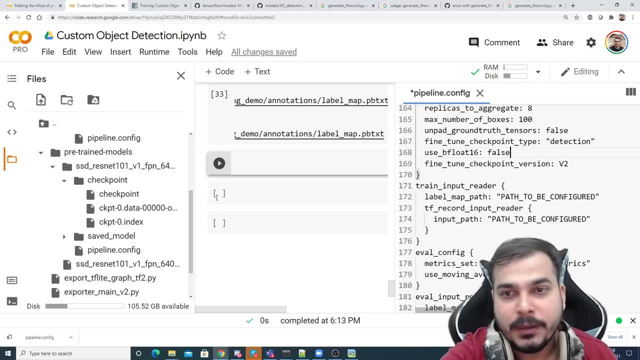 you can see the path, guys. so finding checkpoints i need to update then this: use b underscore, float 16. it should be false, okay, so here it is. i have updated it now again, i'll go back over here. next point that i need to update is 172, so i'll go over here to 172. 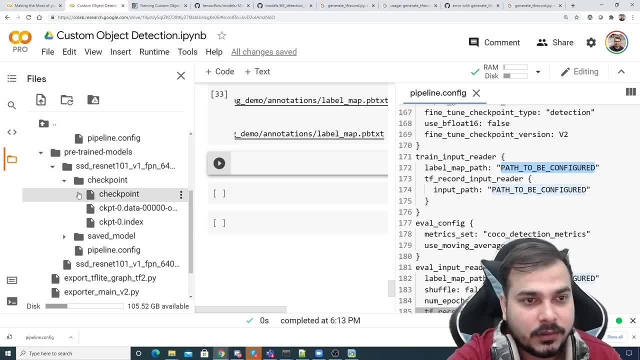 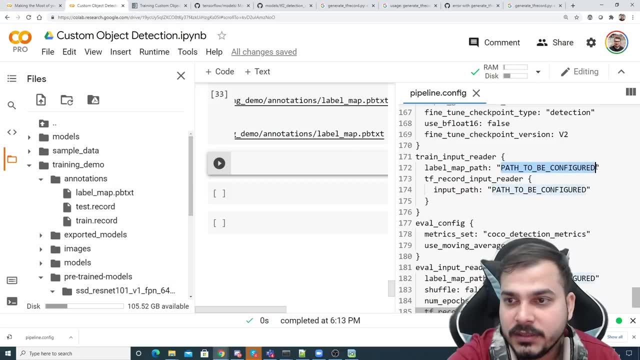 this path needs to be configured with the label map path. now what is my label map path? if i go and see inside my annotation, this is my label map path. i'm just going to copy this and paste it over here. it's like just copy and pasting, guys. 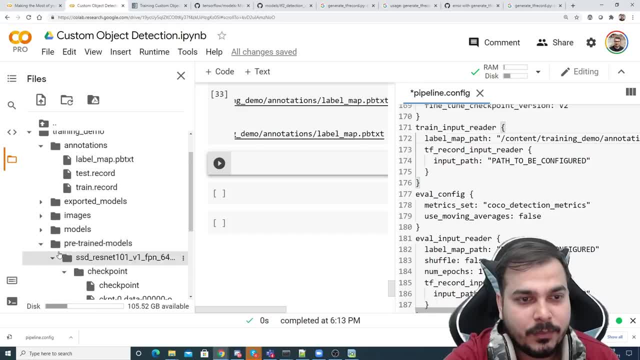 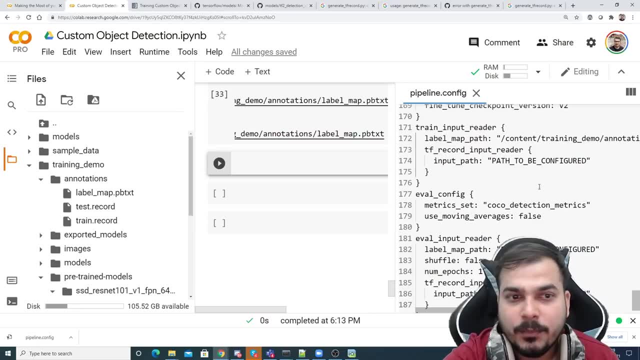 okay, then, uh, the input path that i will probably be having. so let me see the input path. this input path will probably have the path of my train dot record. okay, so i'm just going to copy this path and paste it over here. perfect, this is done, train dot record. then again, i need to change this, uh. 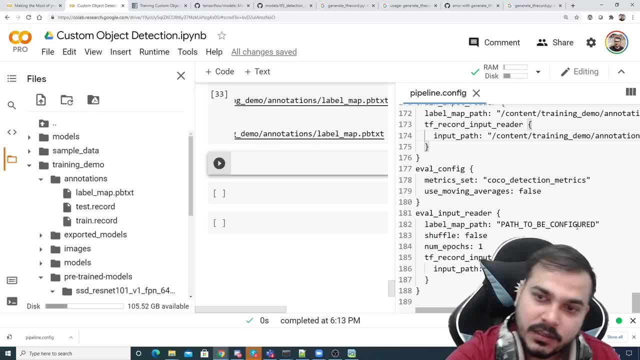 which is like label map, again, part to be configured. see this, guys. here you can see part to be configured again. i'll try to put my label map path. i'll paste it over here, perfectly done, and then i will be taking this input path, which will be with respect to my test. 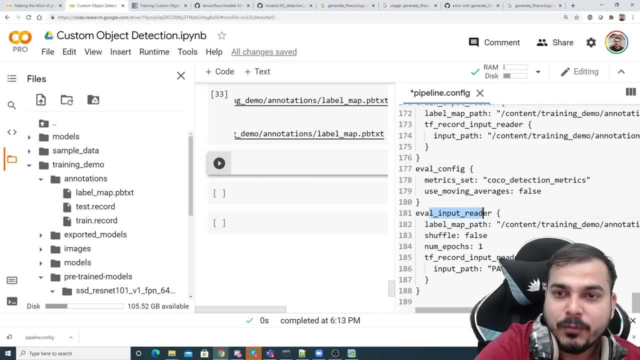 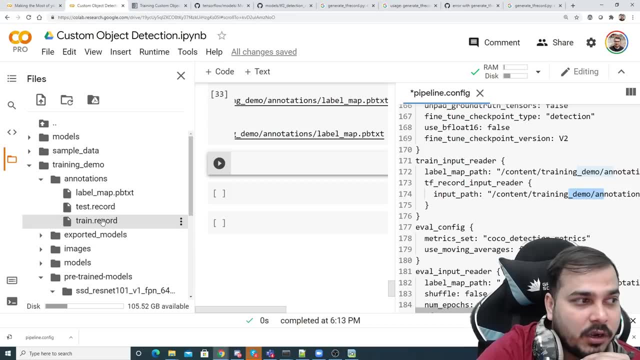 data right. so this is basically my in val input reader. this is my train input reader. when i have train input reader, i have to basically use this training path right, this trainrecord. for this i have to use this testrecord. okay, so here i'm just going to update it. 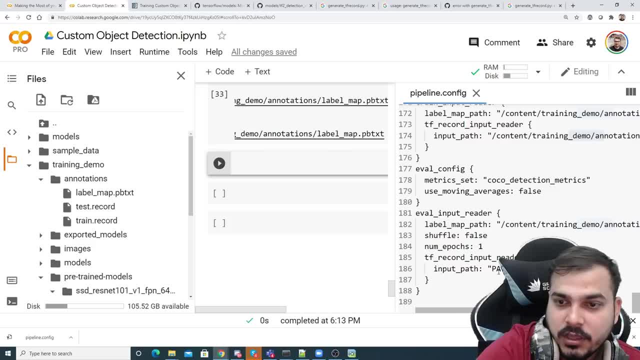 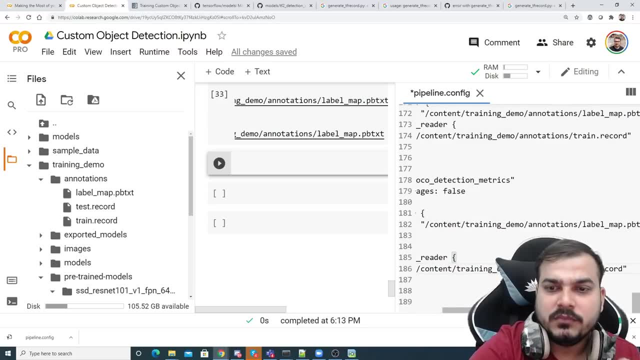 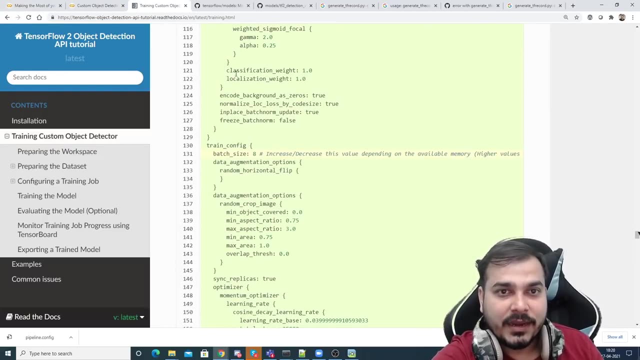 inside this label map path. i have done it, okay, guys? so let's see, there is this input part, so i'm going to make these changes and update the path over here. that's it, and this is the steps that we really need to do it. make sure you just follow this file- which which line, and remember which is. 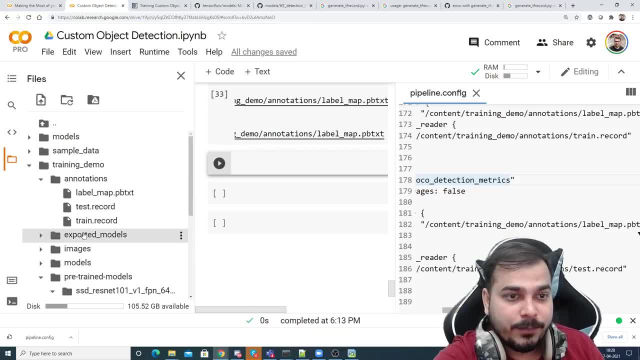 this pipeline config. so i'm just going to copy this and paste it over here and paste it over here: pipeline config. this pipeline config is nothing but the same pipeline config which we have pasted inside our models. see this? i'll just open this again. this is my models. okay, my shd, this one. 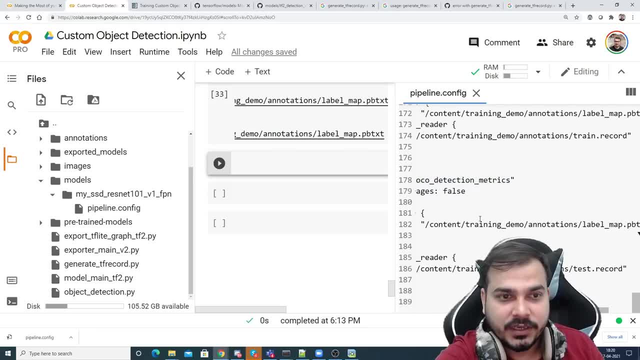 is their pipeline config. this is the pipeline config that i have made the changes in. okay, this pipeline config, i have copied and pasted it from my pre-trained models, right, if you remember, from this pre-trained models, i have to use it and that is what is the step basically mentioned over. 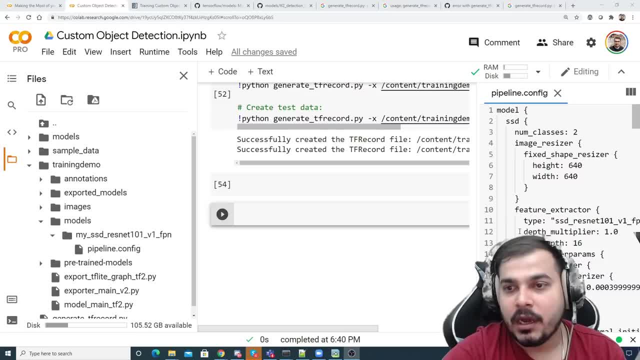 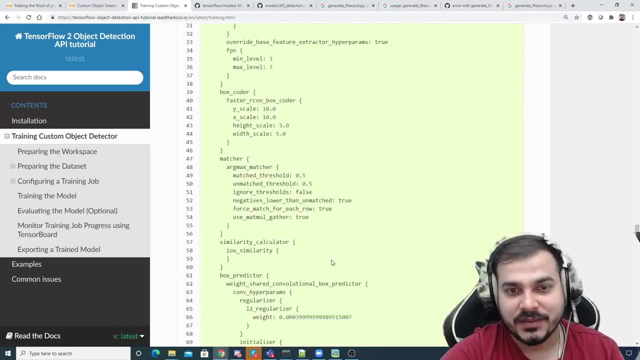 here. okay, guys, the pipeline config has been updated. now, probably the next step that we basically have to do. if i go down over here after the pipeline config, make sure that you follow the specific lines like this right, like number three: you need to make a change. then you need: 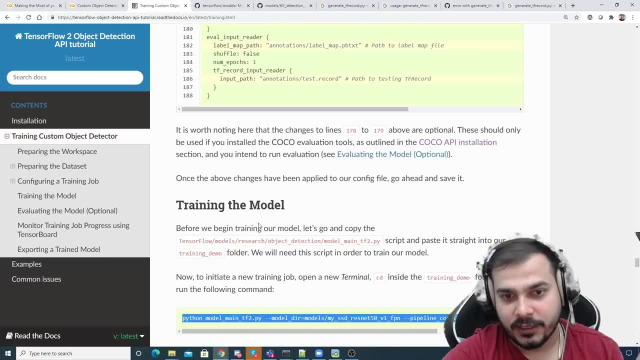 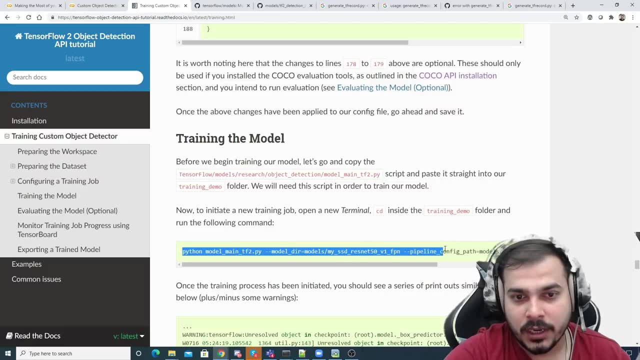 to make a change on 131. like the same thing, guys, nothing different. okay, so i'm referring to this particular block. now the next thing is that we need to execute this particular code. now, where is this model underscore main, tf2 dot py? i'll just go over here. i'll just close this. 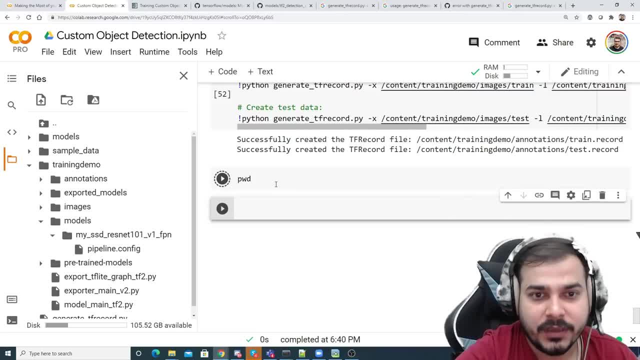 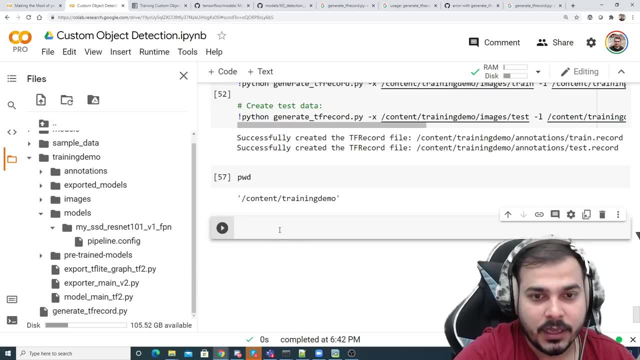 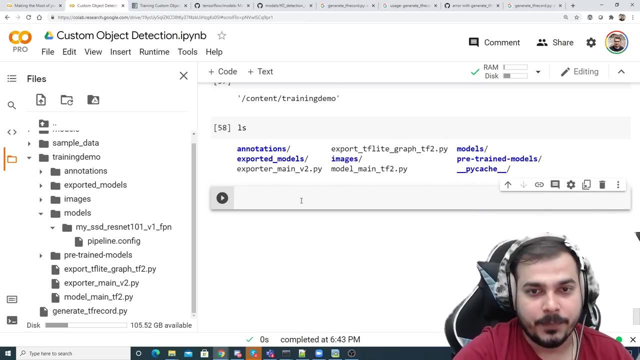 pipeline config. now right off. let me see where i'm in pwd. so it is in training demo folder itself. and if i go and see over here, model underscore main dot p, underscore tf2.py is there. so i'll just write less. so just see all the list of my files. probably i'll be able to see over here. now i'm 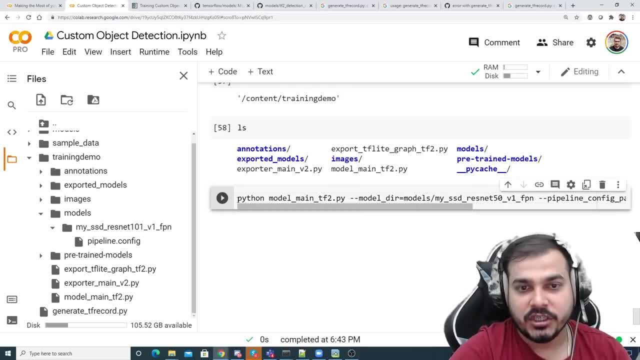 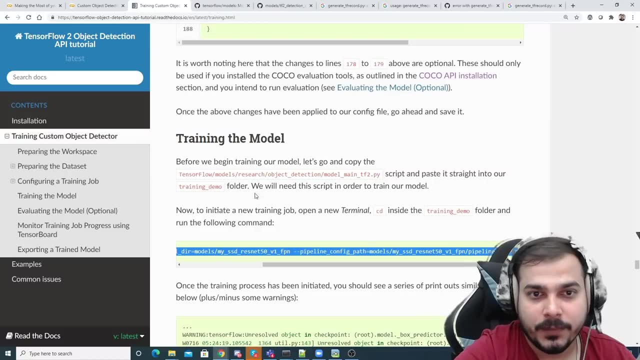 just going to paste it and remember: i have to make some changes over here, right? so this is for creating my training pipeline, right? so i'll write like this: see, this is the step i'll go over here, not training the model. i need to train the model now. what all path i need to change first of all, 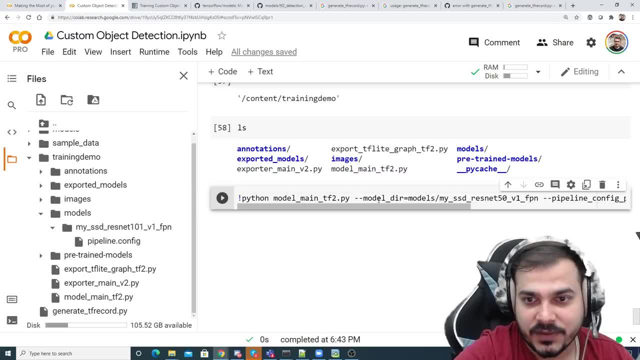 my model directory. model directory is nothing but this, this specific directory. so i'm just going to remove this and paste it over here, okay. similarly, i'm just going to remove this path and paste it over here with the pipeline config. okay, only these two changes will be there. fine, we are done this. 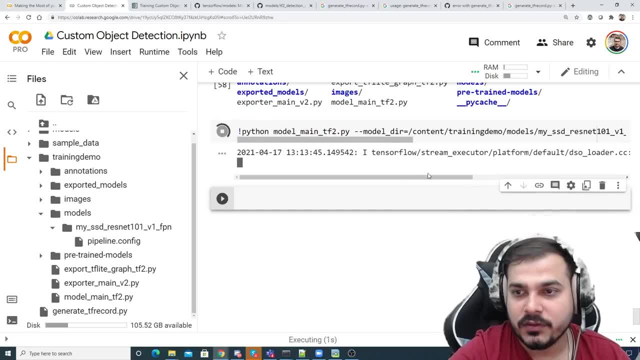 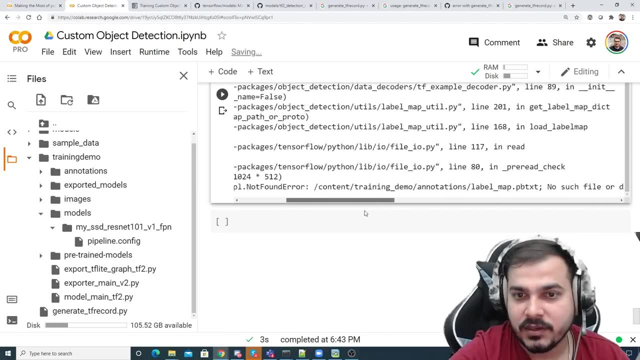 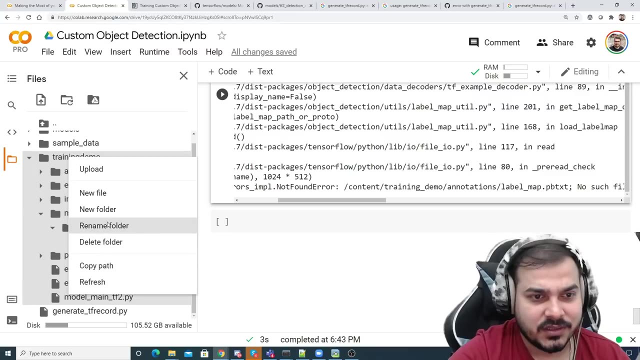 i'll go over here and execute it now. once i execute it, you'll be able to see that probably the training will start. uh, i'm getting some errors saying that no file or such directory. okay content training demo annotation. let's see. uh, oh, why did i rename this? sorry, it should not be renamed. 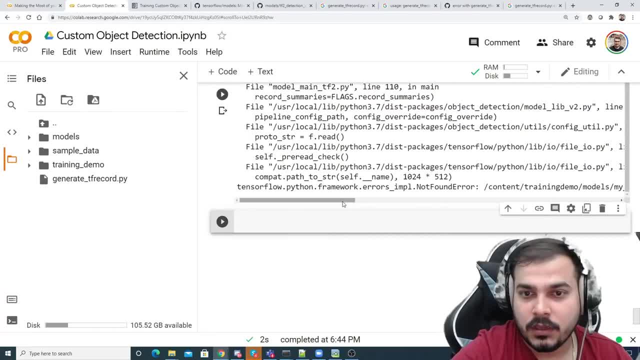 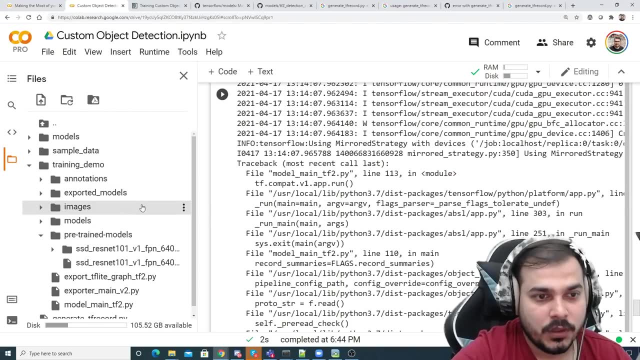 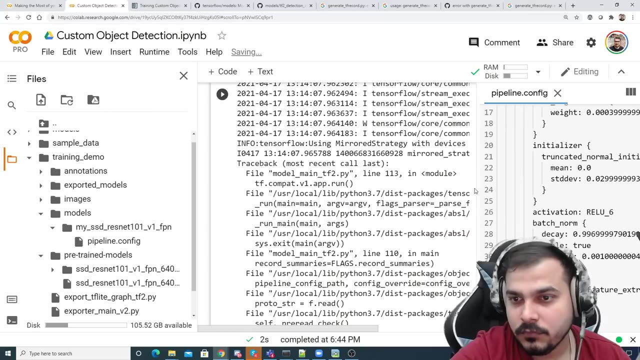 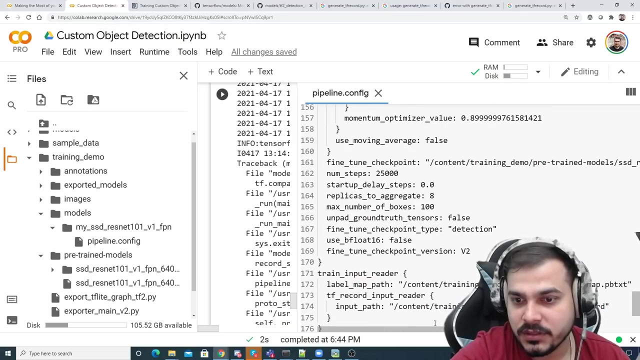 so now the execution is started. content: training demo. so let me just go over here. with respect to the path, there's some problem right in my pipeline config. let me just see. okay, so i'll just go and check out my path. so where is my path? training underscore demo. this is there. training underscore. 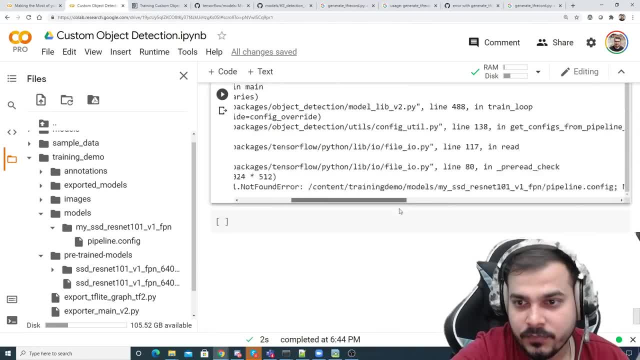 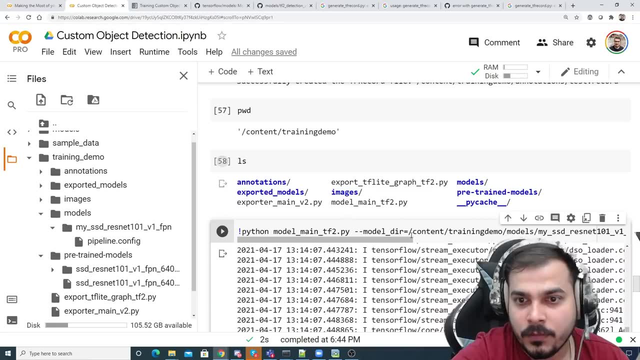 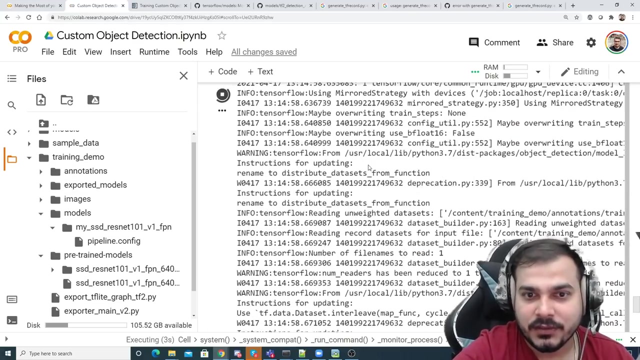 demo. all the paths are perfectly fine. what is the error that i am getting? okay, so training okay here. i had written training demo. sorry for that, but this will get fixed, don't worry. this is a smaller issue with respect to my path. i made it training underscore demo. i don't know how it got renamed, so now it started. 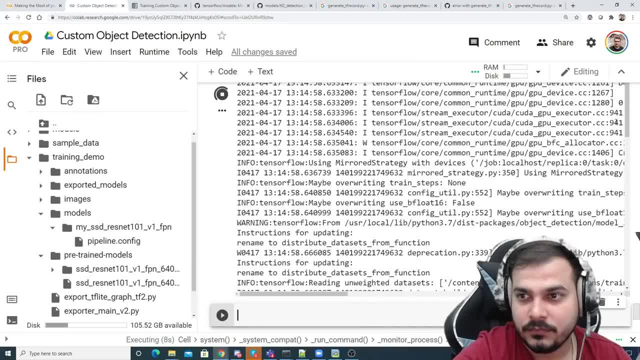 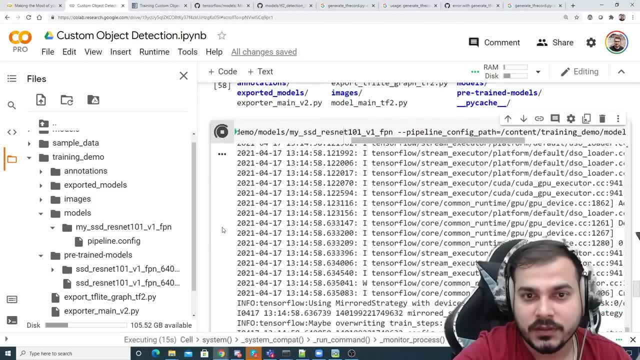 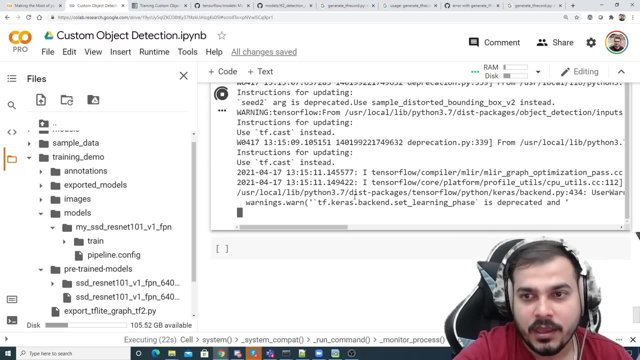 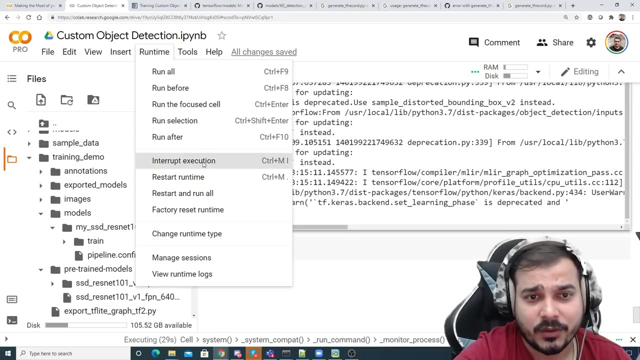 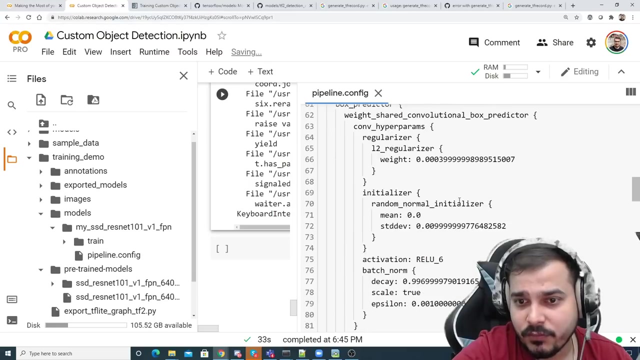 over here. so here you can see all the execution are happening perfectly fine, and now it is started. see this now, if you remember, guys, uh, one thing, oh, one thing. i did not make change. let me just interrupt it. okay, interrupt this execution. okay, let me go to my pipeline config. again, inside my pipeline config, i want to see: 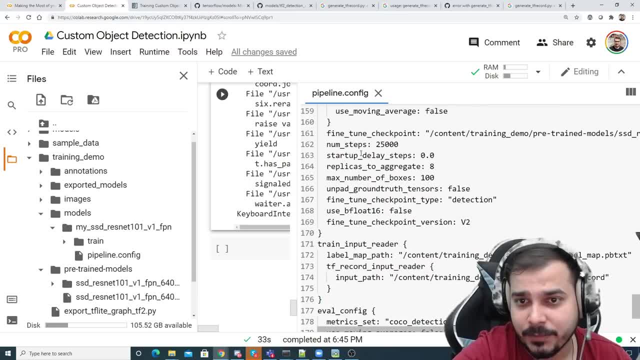 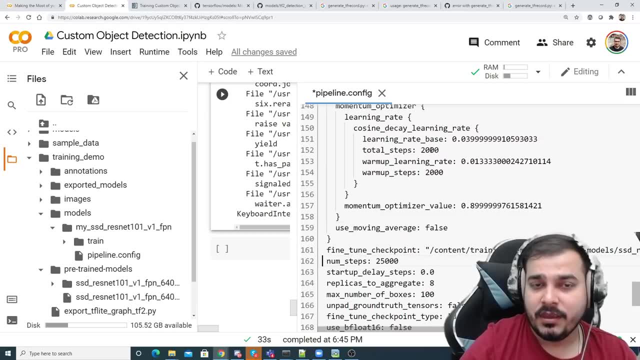 that how many. number of step size that i keep it. so again, number of step size: i've kept it as total steps. i've kept it as 25 000. it is obviously going to take time, so what i'm going to do is that i'm just going to make it as 2: 2000. you know, 2000 step size. make sure that you make the changes. 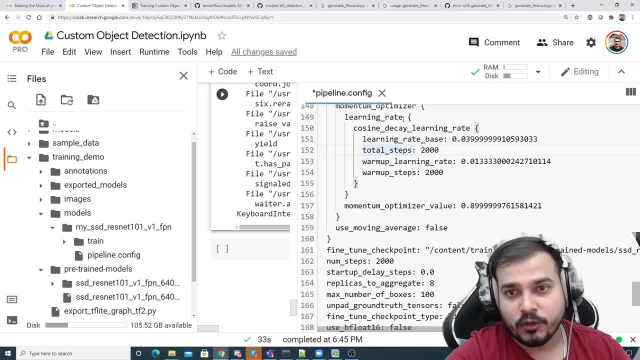 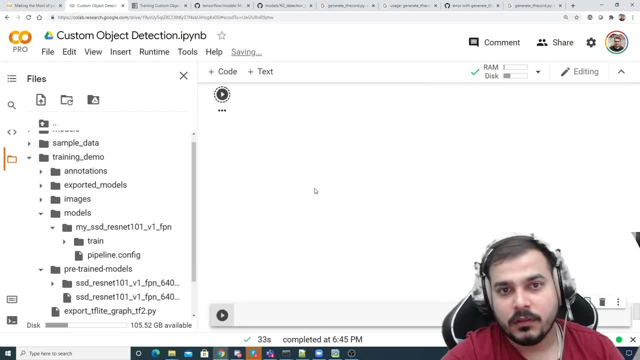 in 152 and 162 and the current step size. just make sure that you make the changes in 162 and 165 you to like. okay, quickly. so I'm going to save it, close this and again execute it once again now. I think it should work fine, okay now. now the execution will. 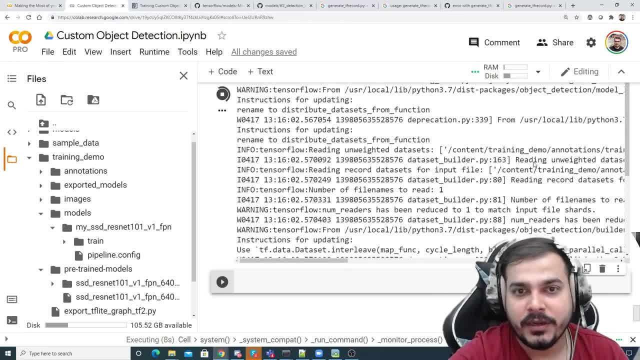 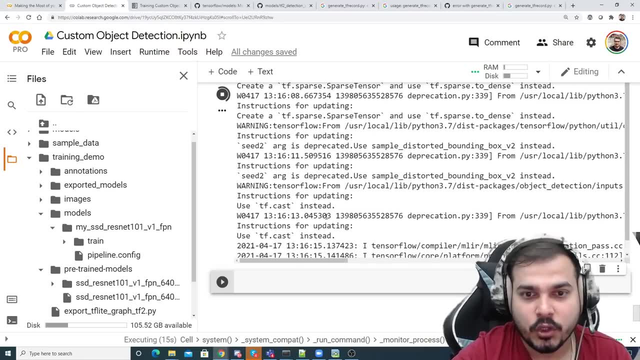 start. okay, now let's see, let's wait. how much time it will take now, if this is working fine, probably at after some time, you know, you'll be able to see steps. you know like hundred steps, two hundred steps and all right, and probably, if I'm 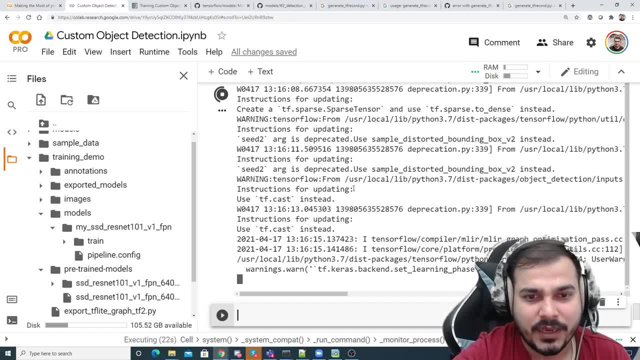 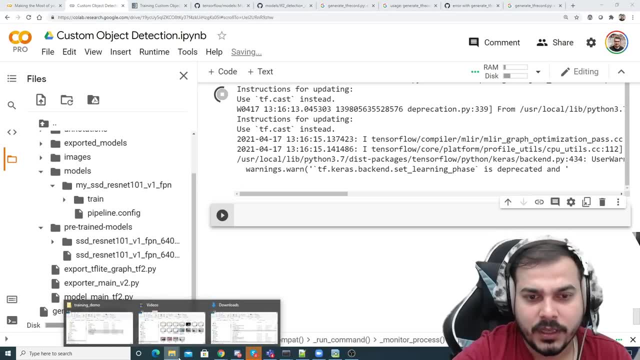 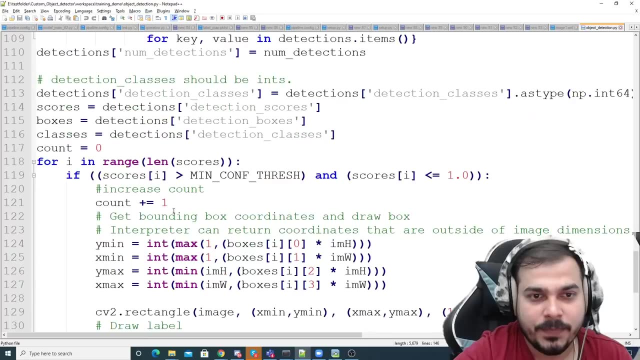 doing it in Google collab. two thousand steps will be done very, very quickly. now, after this, what I will do is that I have already uploaded one. probably, if I go over here in my training demo, there is an object detection file, right, so I'm just going to execute this particular file, okay, and this will basically take. 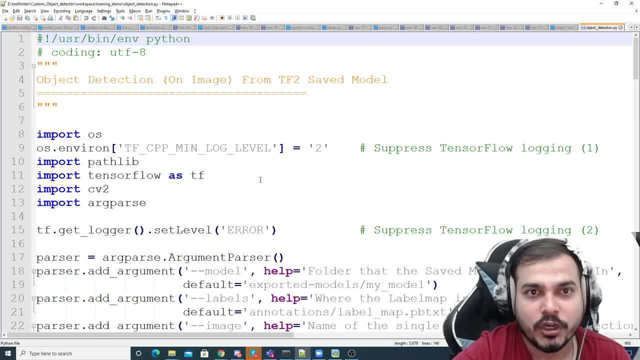 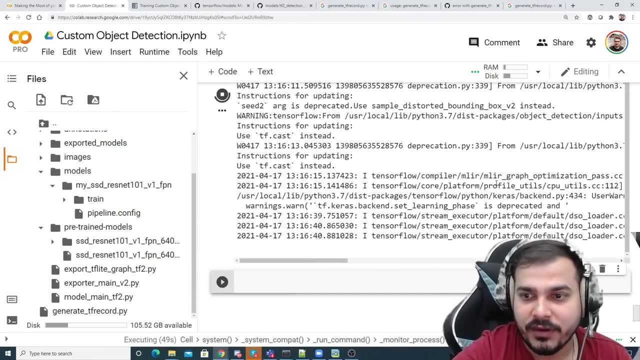 images and once it takes the images, it is going to basically give the prediction. this is my dot py file. okay, but before that, let's see this training. okay, the training will start. okay, so I'm just going to go ahead and click on the start button, and it will take some time, I think. till now, everything is working. 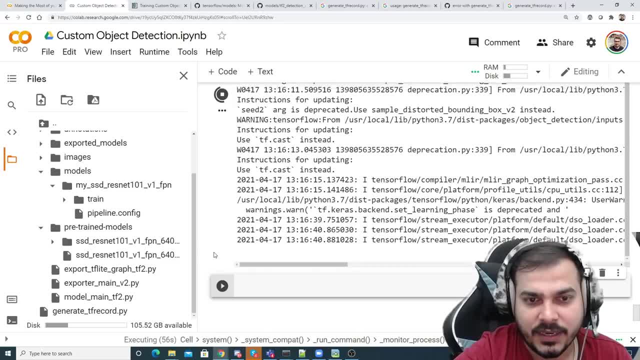 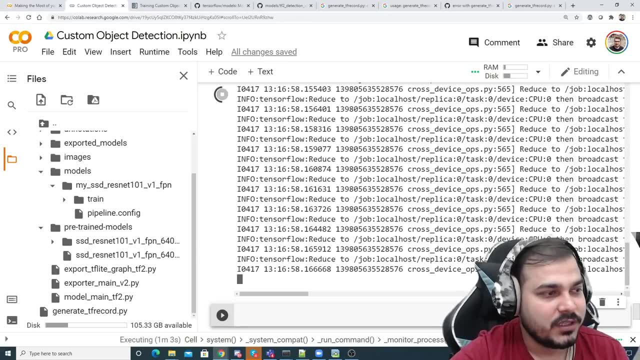 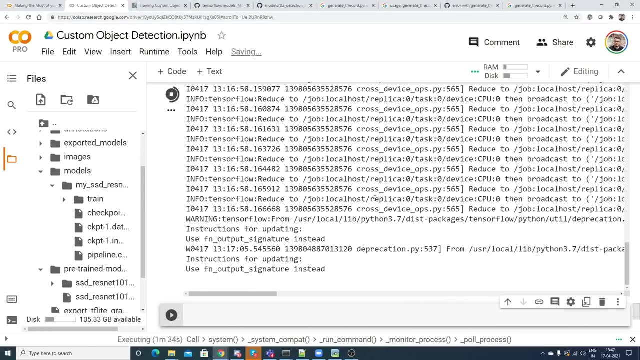 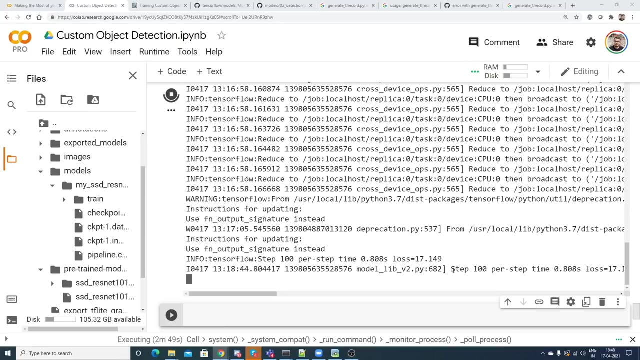 fine. I guess it is using the GPU. everything is working. fine, we'll wait. okay, we'll wait some some time. until then, I'll just switch off my video so that you'll be able to see the training process. okay, enjoy the training, you, you, you. so now, here you can see guys step hundred per time stamp with loss. this. 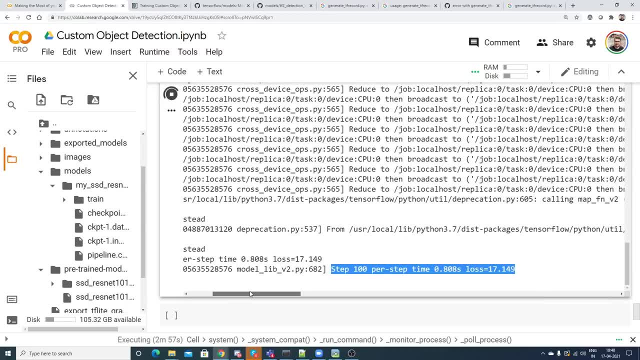 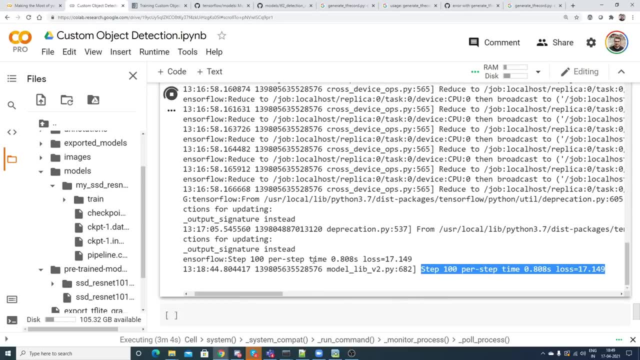 much. we have started running it and probably it'll be running for some more steps. total steps will be two thousand. okay, so we will just wait till sometime. so you this type, if you are getting it, that basically means that you are. your training is happening properly, okay. 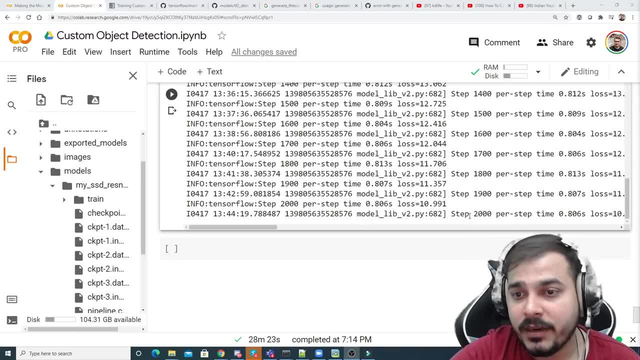 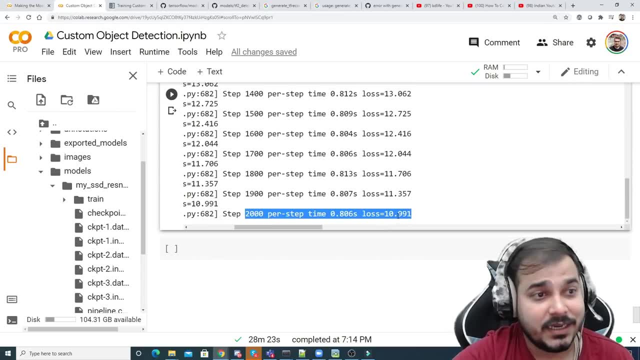 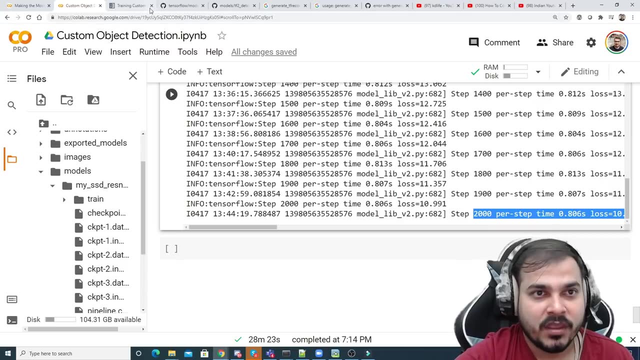 so, guys, the training has happened. it has completed two thousand steps and you can see the loss function initially was seventeen, point one, four, nine and it is coming till ten. just to show you quickly. I've stopped the training right now, but let's see how the performance of the specific model is there. now I'll go back. 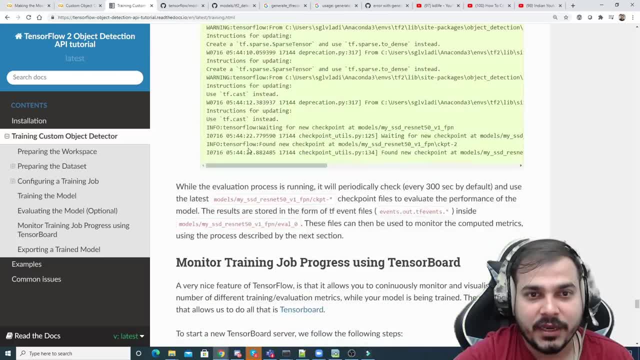 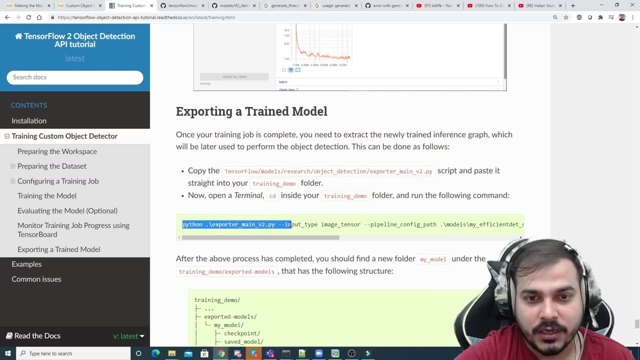 to the blog. the next step is basically: after doing this, you know, after training it, you need to export this particular specific training model and in order to for doing this, you need to write this specific code, right: exporter, underscore, main, dot, py, right. so I'll just copy this particular code, this line of code, and 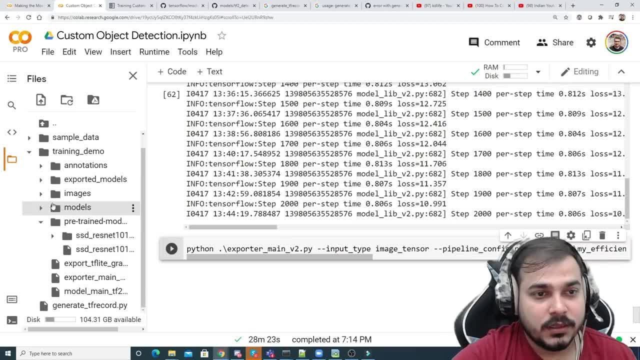 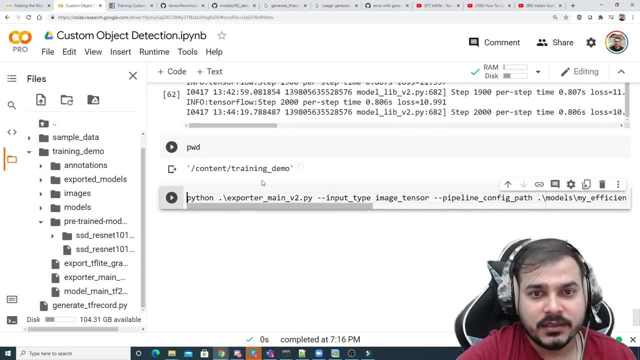 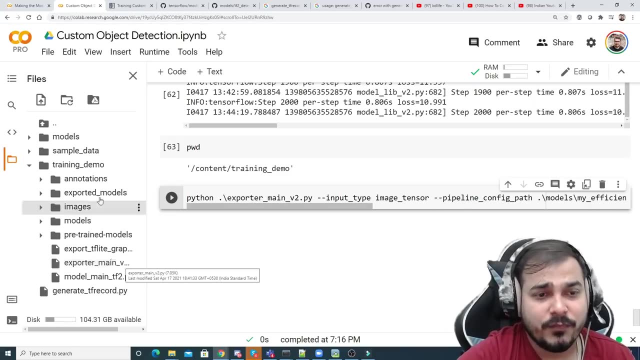 then paste it over here. remember right now, if I, if I go and see which is my PWD, that is my current working directory. it is inside training demo, and inside training demo I already have this specific file: exporter, underscore main dot py. now you may be thinking from where I'm taking this particular file. 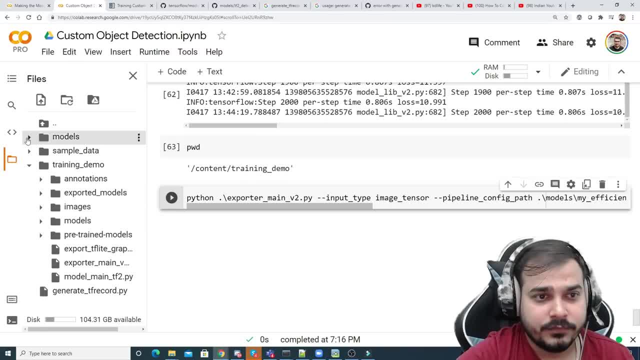 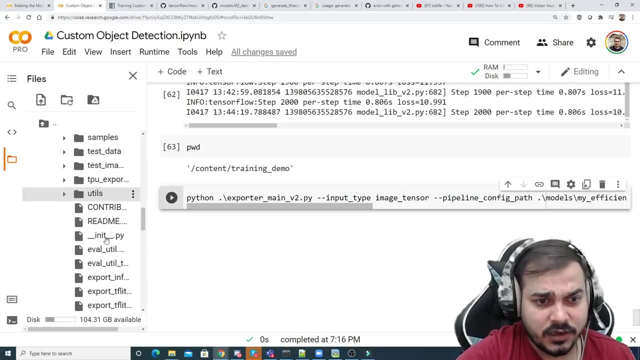 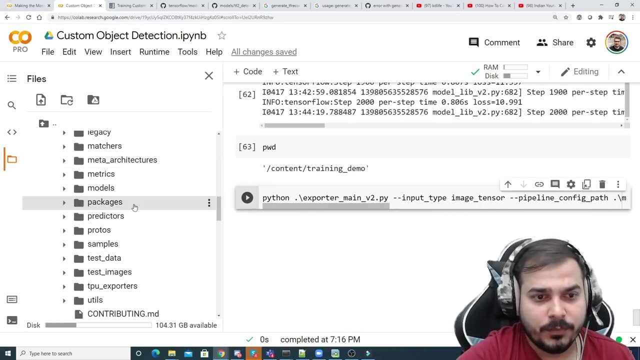 guys, it is already present in our research folder. see that: models research. if you go inside this and if you go inside object detection, this file is already present. okay, export, every, every file is present over here and I'm just reusing that same file. okay, exporter, main dot py. see this somewhere. this will. 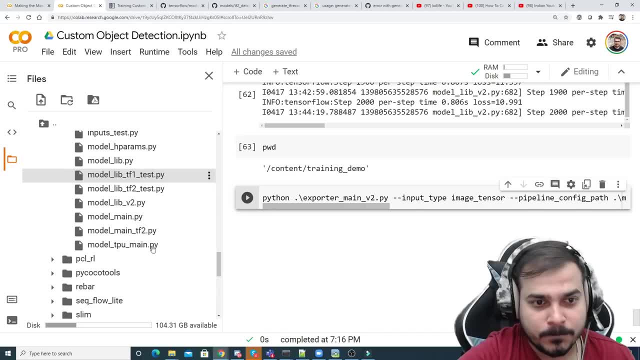 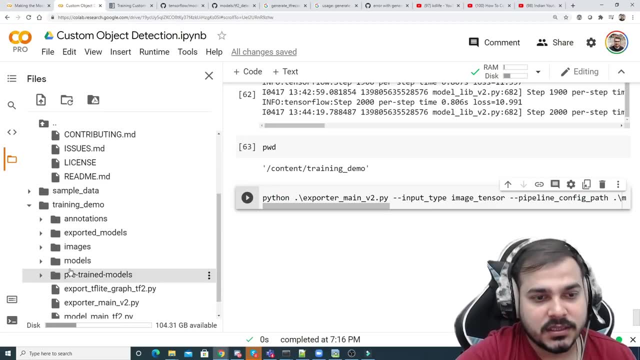 be there model main tf2. is there exporter main py file? I don't see it, but don't worry, I'll try to give it you in this, in the github link, all this particular file. now I have this particular file. now what I'm going to do. 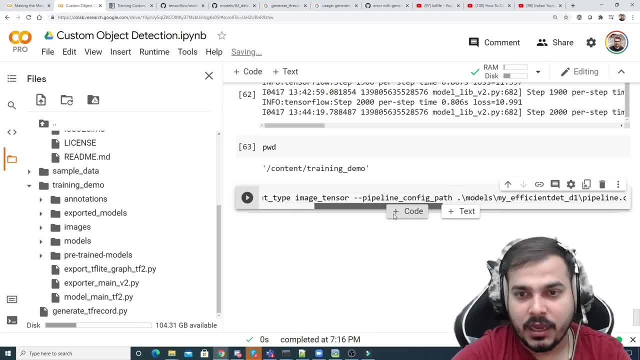 is that I'm just going to remove this dot. I don't require it now. one thing that I really need to change is my pipeline config path right right now. currently, this is my path. now, if I go to my pipeline config path, this should be the path. it should get updated with right. so I'm just going to copy this. 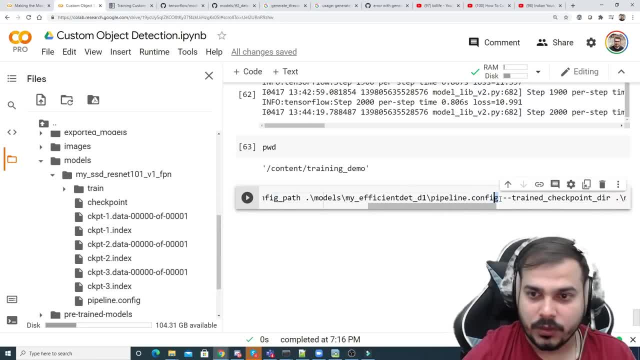 particular path. okay, and then I'm just going to remove this, because every command you need to change this specific path, guys. then my train checkpoint: again, this should be my directory path. so this is my directory path over here. I'm just going to change it. okay, this is done. then the output directory is nothing but the exported. 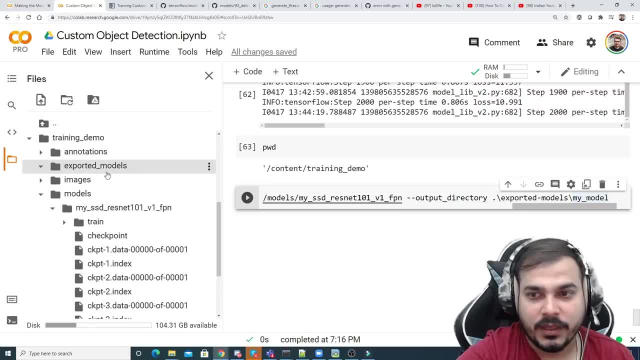 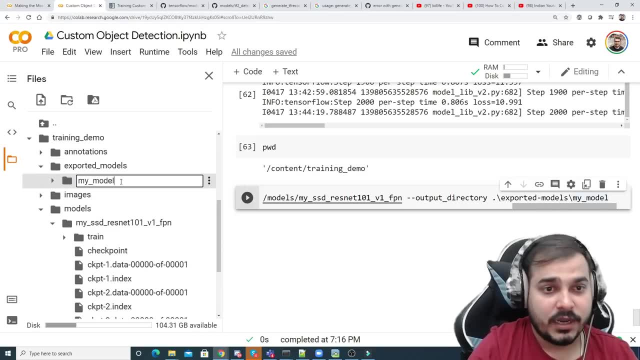 models- exported models. for this I've created a folder over here and inside this I will create another folder which is like my underscore model, so that my exported model will be available over here. right, so I've done it, so let me take this specific path and paste it. 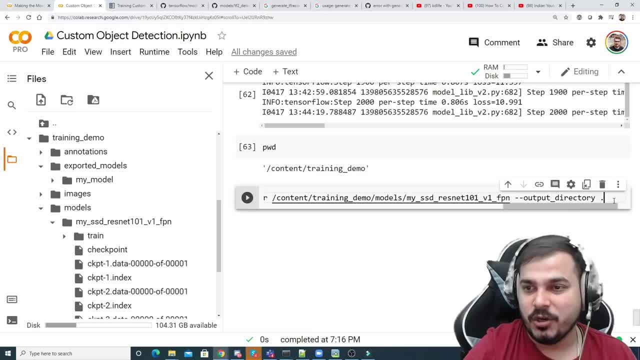 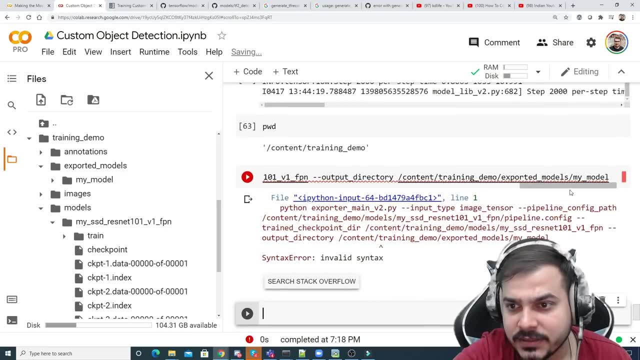 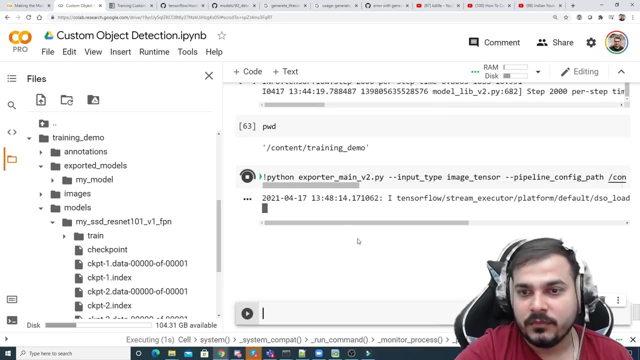 over here. only this: many changes that I have to do. I know it will take many steps to do it, guys, but just follow these steps, whatever I have done. okay, it shows invalid syntax. let me see. okay, invalid syntax. it is probably showing because I have to write over here now. it will work fine now after some time you. 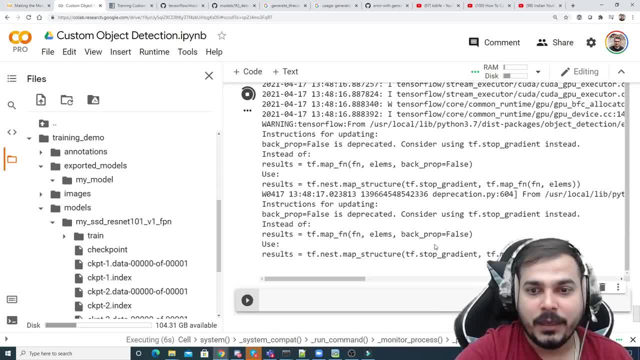 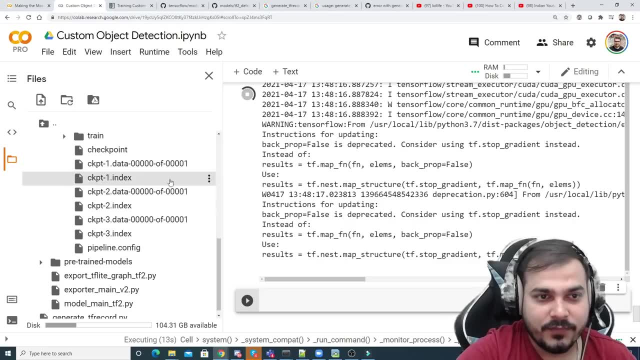 will be able to see inside this, my model. you will be able to see a PB file that will be present inside it. okay, we are exporting the model, exporting the model from here, right from this particular checkpoint. right, because here we have this entire train checkpoints. so, again, 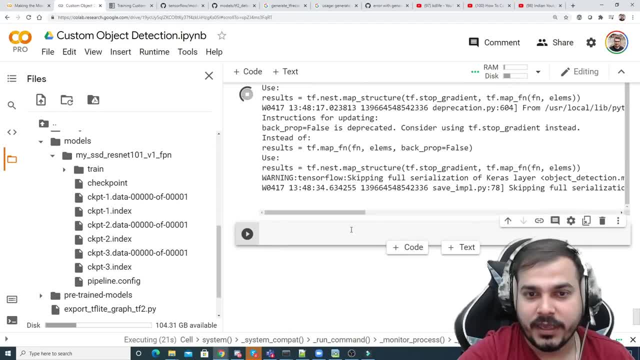 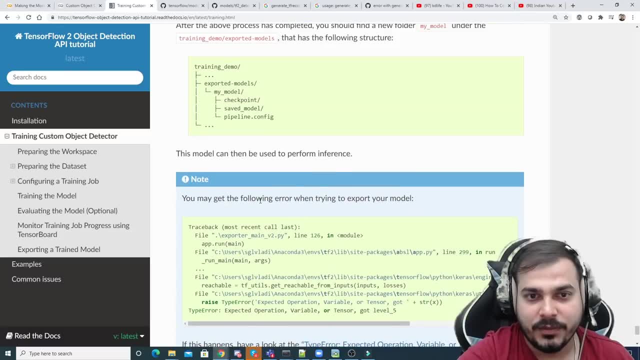 it will take some time. let's see how much time it will probably take. skipping full serialization, all these things, kind of things are there. so here you will be able to see: if you are getting this kind of error, then probably you have done something wrong, but other than that everything will get executed perfectly. 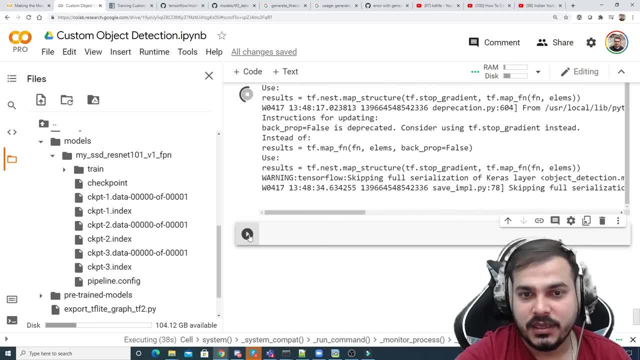 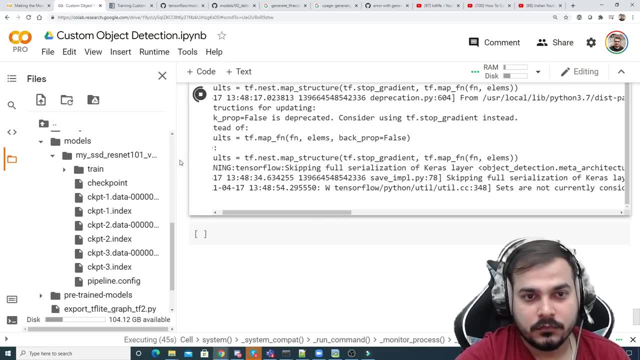 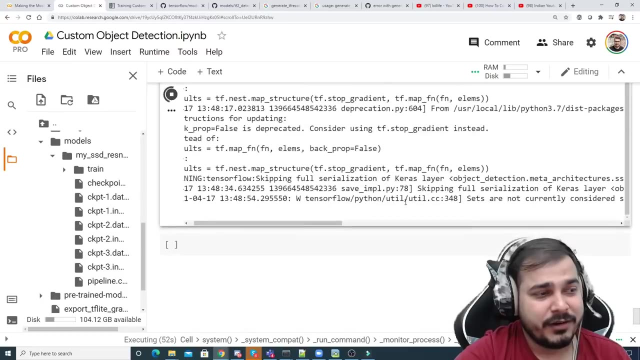 right. so here it is. let's see how much time still. I don't think so you will get any error, because I have done it many number of times. to create this kind of videos right, you really need to execute it more number of times and probably check whether you are getting any error or not. 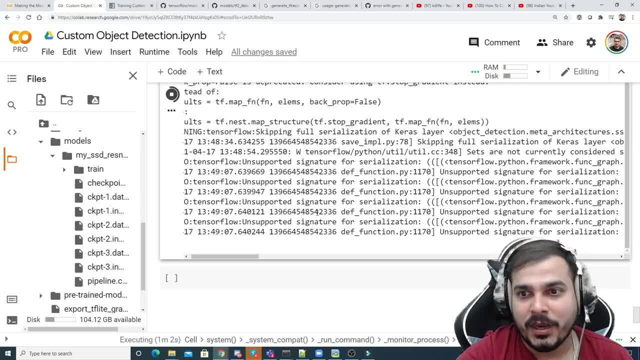 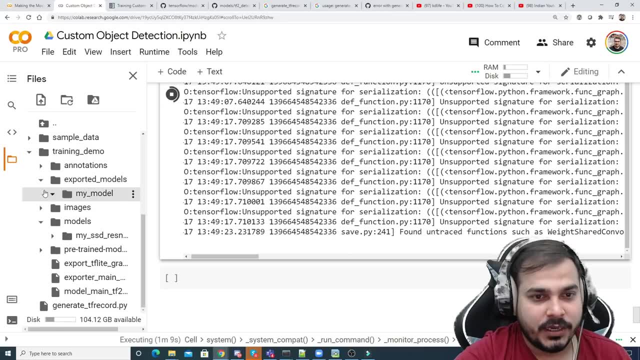 otherwise it will be very, very difficult while teaching you and again doing this particular task, and all right. so anyhow, but this will get trained, I know. so training demo. okay, tell this, exporting is happening, guys. I really want to copy and paste one referencing. now I really need to check about inferencing, right. so 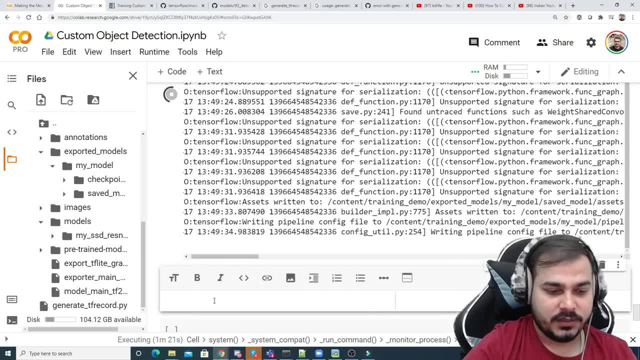 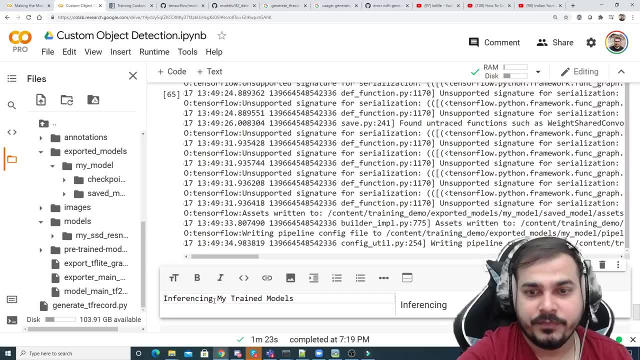 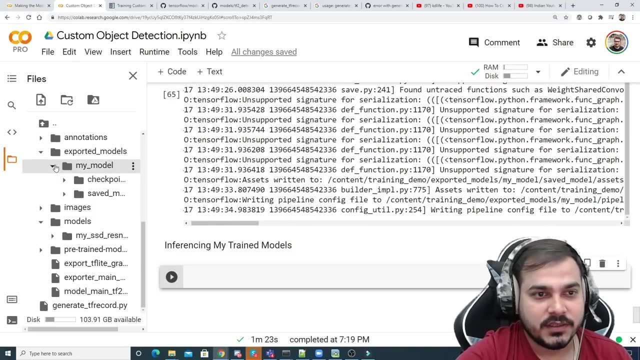 for checking inferencing what I'll do. I'll just write down the comment saying that inferencing my trained model. basically, now I'll try to see how my train model is basically performing. okay, okay, perfect, I see it has got executed. now let me go and see in my models. oh, 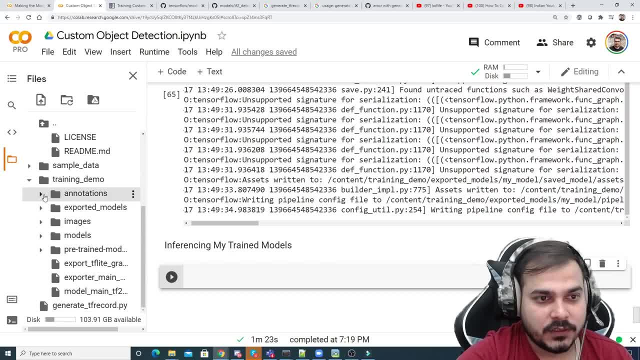 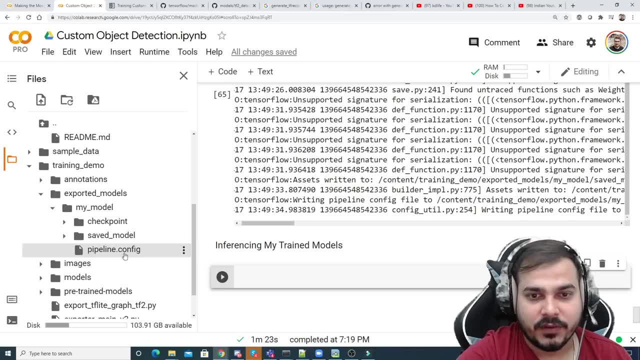 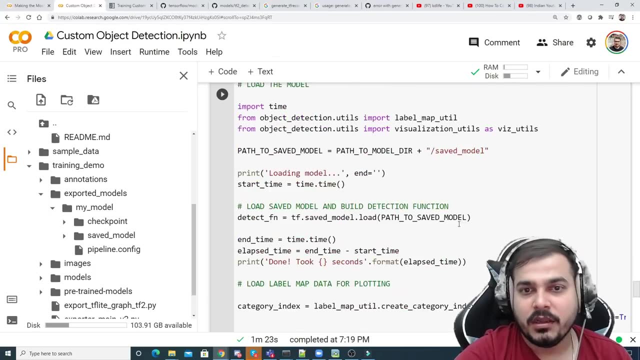 sorry, I'm in research folder- exported models- my models- and inside this you'll be able to see checkpoint folder, save model folder and pipeline config. perfect now inferencing my trained model. I have already written a piece of code, so I'm just going to paste it over here now. 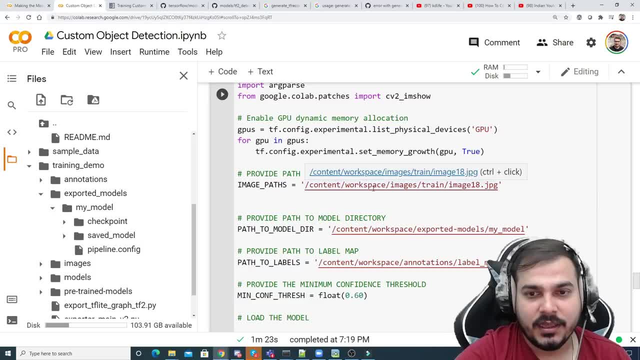 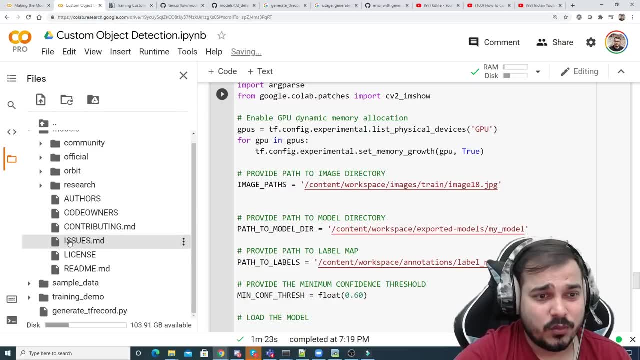 this particular code will say that: okay, for which images you want to check? let me check for one specific image from the test, the trained data, or trash data, whatever data you want. so I'll take one example. so let me go over here training demo. first of all, let me minimize this. 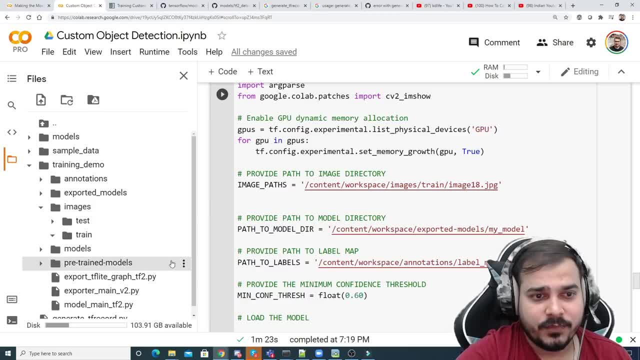 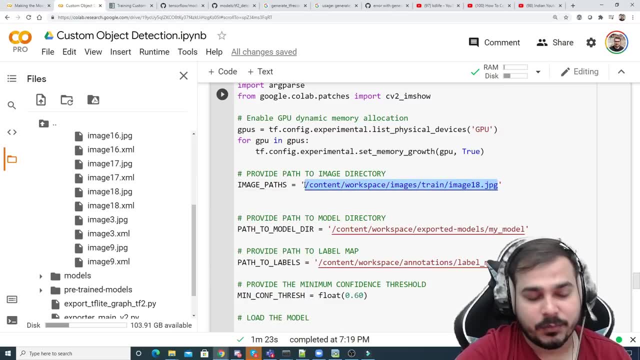 this also now inside my images folder i have this training. any image will take just to see the performance. i see we have just trained it for very less number of images right for very less number of steps. so i feel there may be some kind of problems, but at least we'll be able to see some. 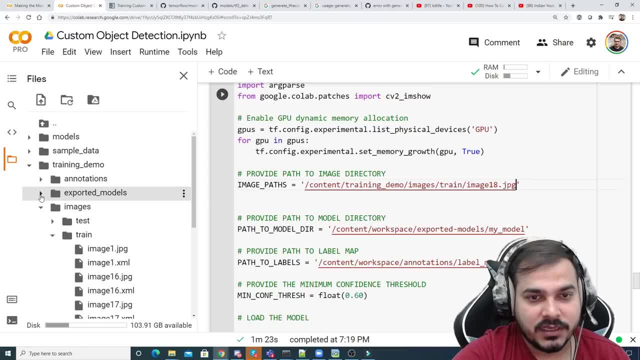 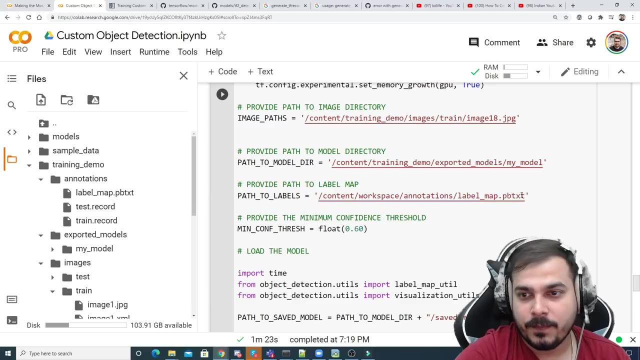 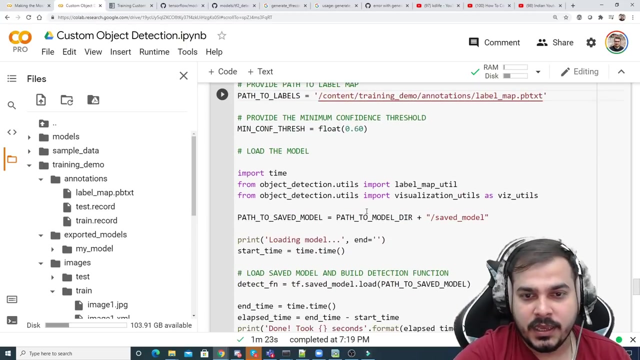 kind of outputs. then, uh, my model directory. obviously this is my model directory and i'm going to copy this entire path. okay, i'm going to copy this entire path and then path to the labels. it is basically present inside this annotation path, annotation path, perfect. and then i just have to make that many number of changes and we are good. 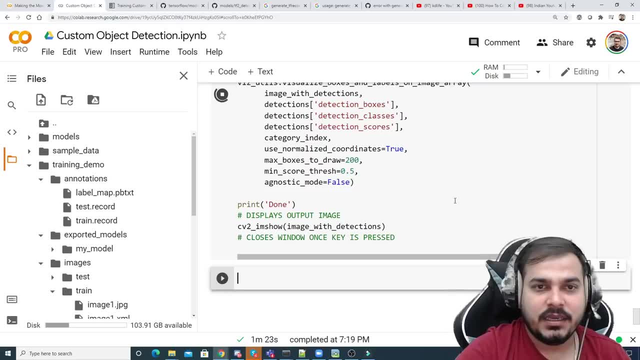 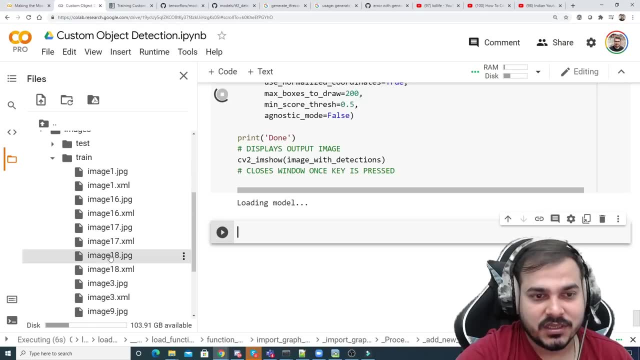 to go now. i'll just try to execute it and let's see how will i get an accuracy. so it's loading a model. so what i've done is that i've given this specific image. you know this 18th image and probably it will try to do an object detection, so this specific image is. 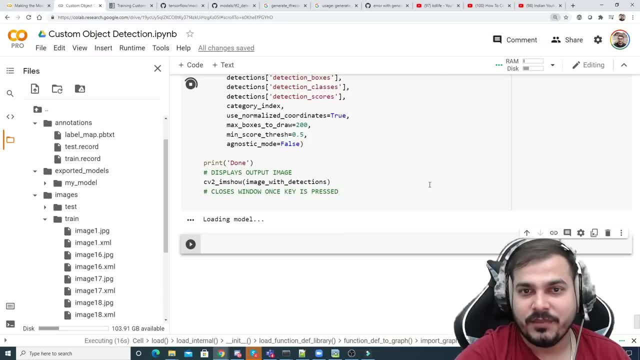 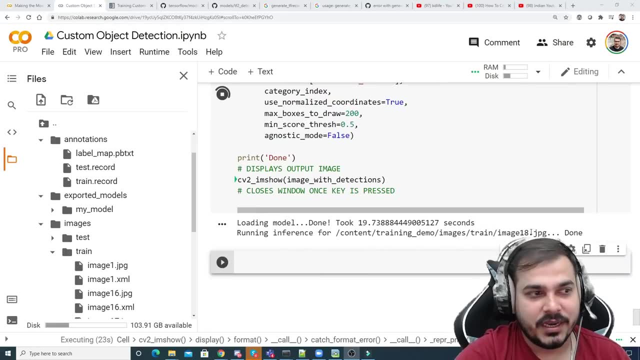 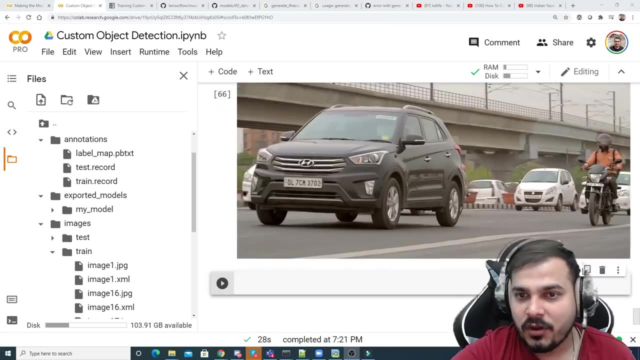 there and it will try to do an object detection for this. okay, so let's try, let's try it out. so, running inferences for this particular 18, image 18: probably you may not get a good result also, but at least you should be getting some kind of bounding boxes. so no, the bounding boxes. 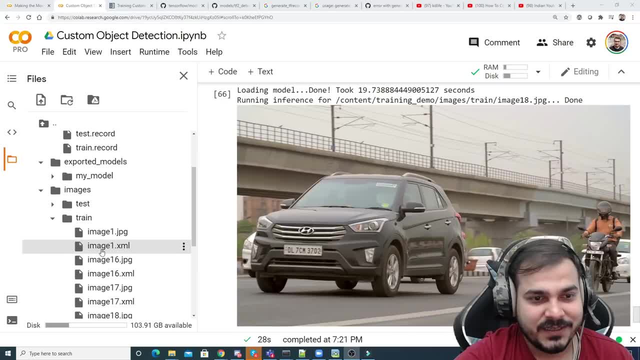 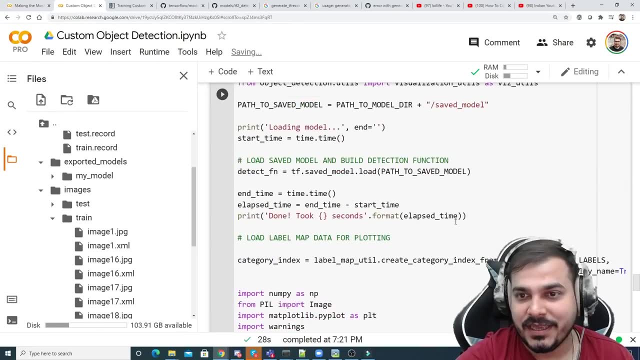 has not come. let me try some other images if possible. i don't know why the bounding boxes has not come, so i'll say image1.jpg. let's see. let's take some more example, it's? it's okay to take multiple examples and check it out, right. 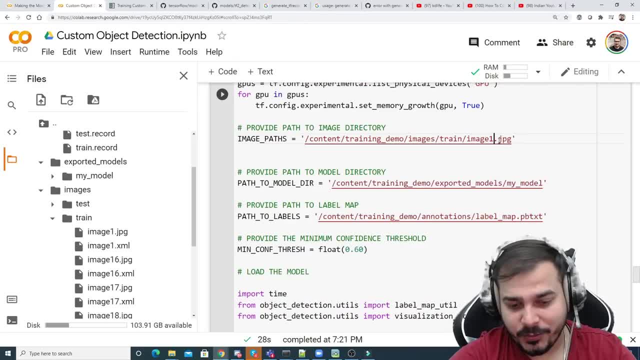 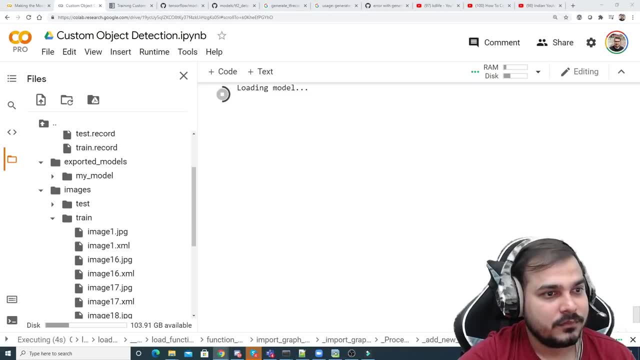 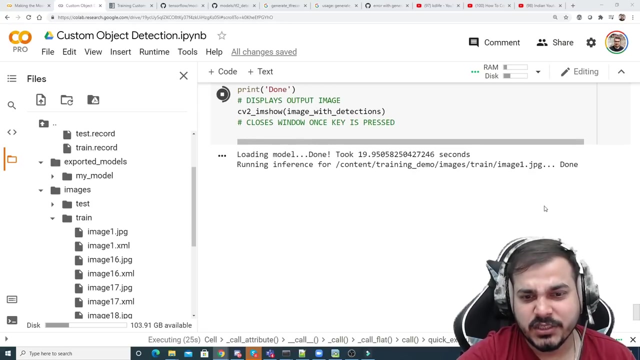 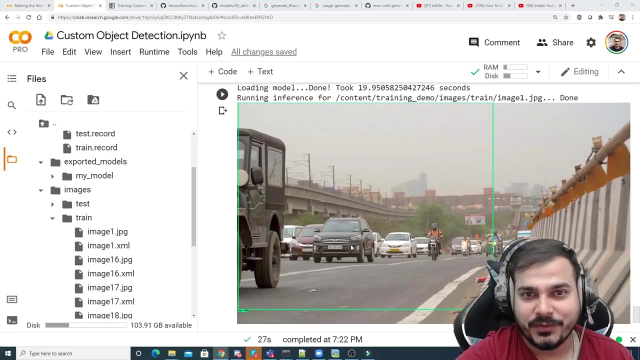 and probably the accuracy may be down, because i really need to train for more number of time. okay, running inferences for this. at least you should be able to get something. otherwise, if you are not able to get it now, see at least some bounding boxes. one bounding box we got. okay, one bounding box. i know that. see, our loss is too high, right. 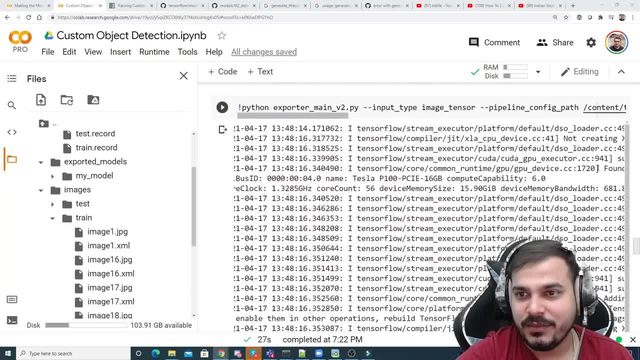 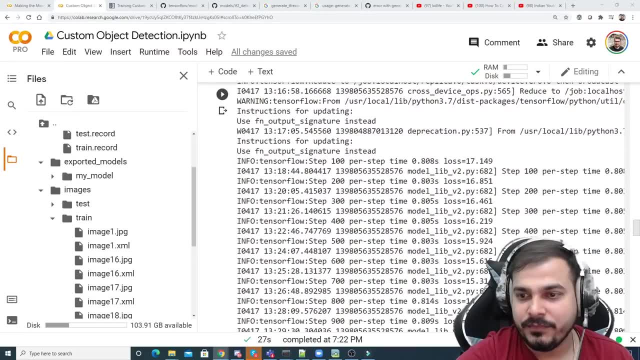 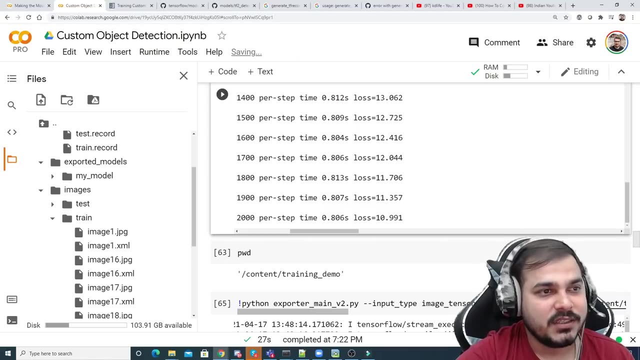 say, if i go and see my loss, we are getting somewhere around. ah see, what is the loss that we were getting inside the box. okay, so at least we get some boundaries under the box. okay, it's getting results. right, so we get inside this. we're getting somewhere on 10.99. now what i'll do is that i will try to execute for. 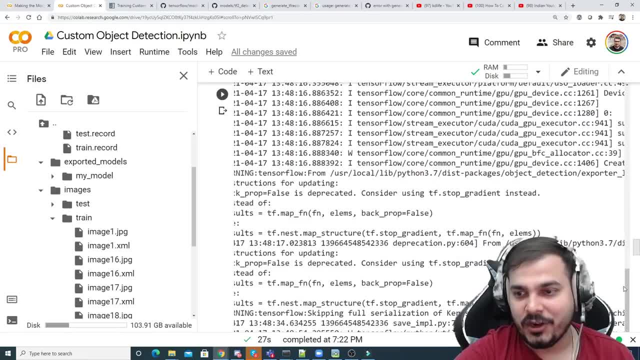 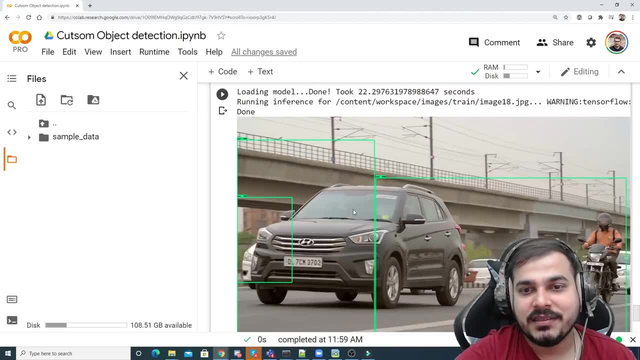 some more time and let's see. uh again, i cannot just do the retraining again and wait for that entire training, but better than this, we'll try to show some results. okay, guys, now what i have done is that i ran it for more 2500 steps. now you'll be able to see it over here. i'm getting this kind. 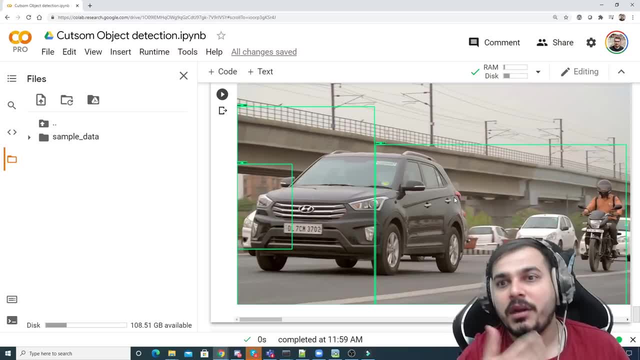 of bounding boxes now. now the thing is that if i keep on increasing the number of training steps- probably i'll try to make it to 25 000- then you'll be able to precisely get the output like this: okay, and this again. after that 2500, i again retrain it for another 2500 steps, and it was. 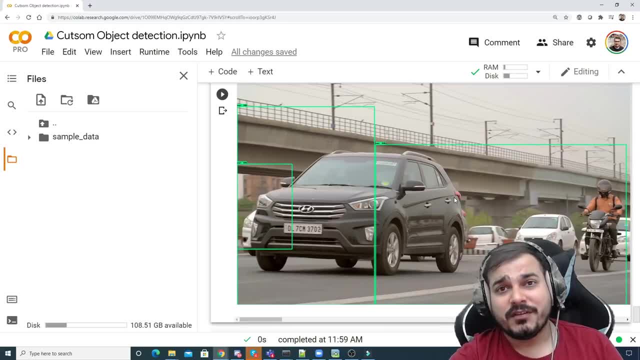 getting improved and i will still try more for more number of steps, and then probably i'll try to check it. but again, the main agenda was this: to show you how you can actually do a custom object detection right. so don't worry about all the files i will definitely make sure that i'll give you all. 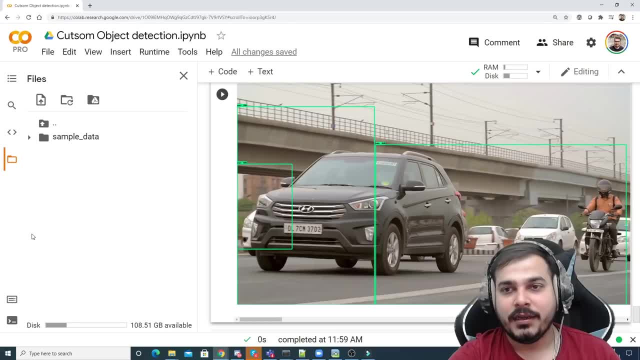 the files in a zip, probably by uploading in my google drive, and you can just follow the steps. make sure that you follow the documentation also. so i hope you like this particular video. please do subscribe the channel. if you're not yet subscribed, i'll see you in the next video. have a great day ahead. 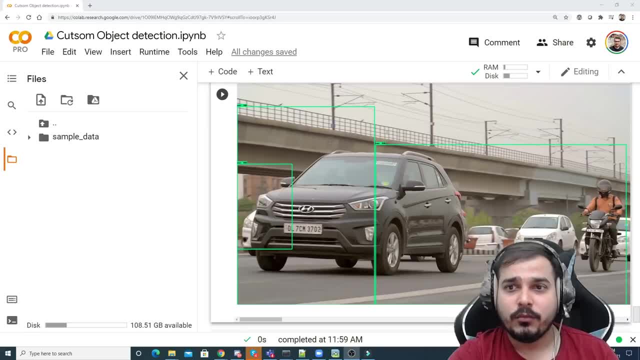 thank you and all and guys, what i'll do also do is that i'll try to make one more live session with respect to object detection. so, thank you, i'll see you all in the next video. bye.